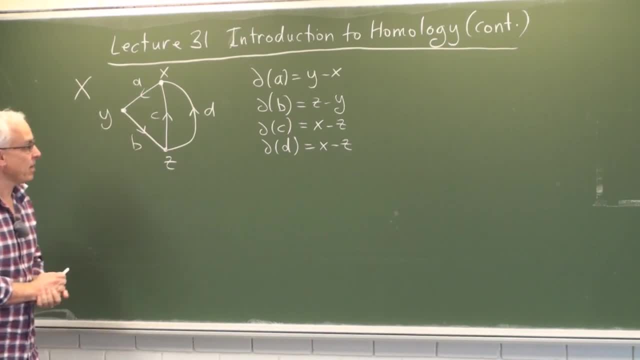 And it's basically just a graph. at this point, a one-dimensional graph, We defined the boundary operator taking an edge, actually a directed edge, Like A, to the difference, the formal difference, between its final point and its initial point. So Y minus X. 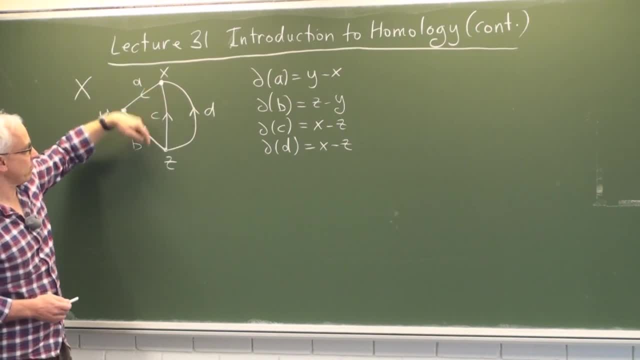 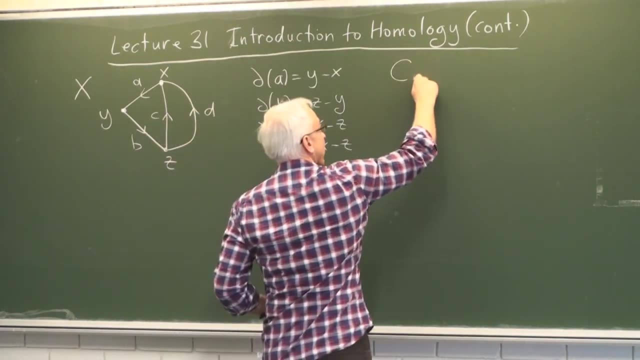 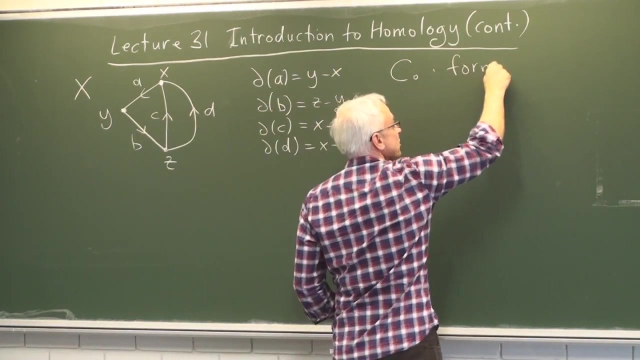 The boundary of B was Z minus Y. The boundary of C and of D were both X minus Z. So what we're thinking here is that we're working in some kind of algebraic framework where we have group C0, which is just, if you like, formal combinations, formal integer combinations. 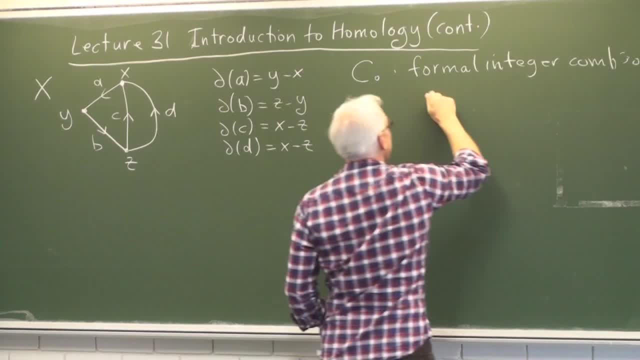 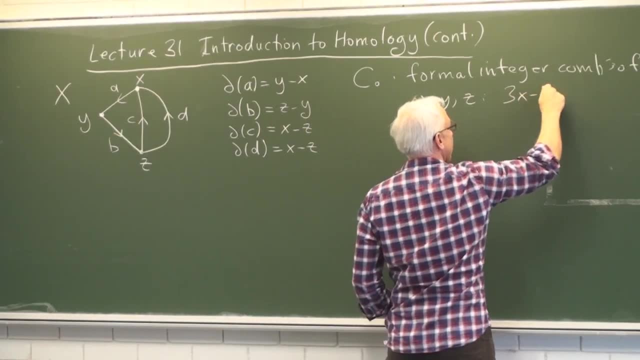 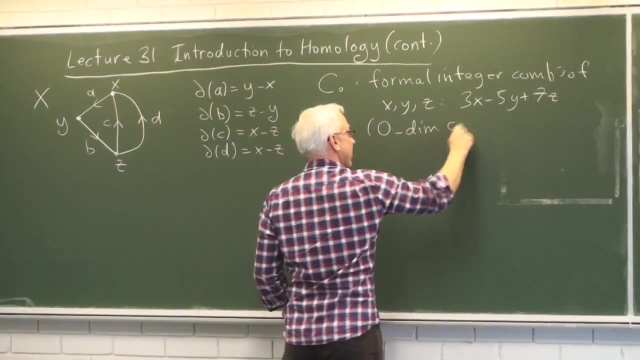 Formal integrations of the vertices X, Y and Z, So things of the form, you know, things like 3X minus 5Y plus 7Z, for example, And these are zero-dimensional chains, Our name for these kinds of objects. 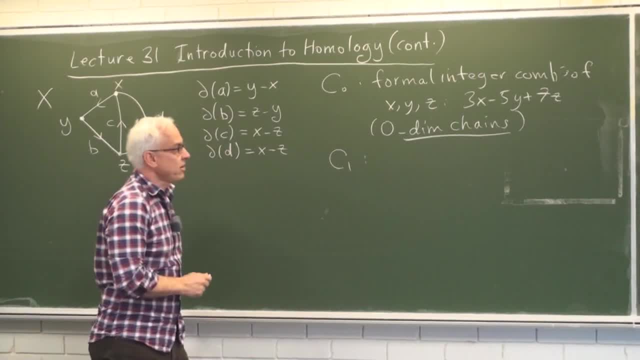 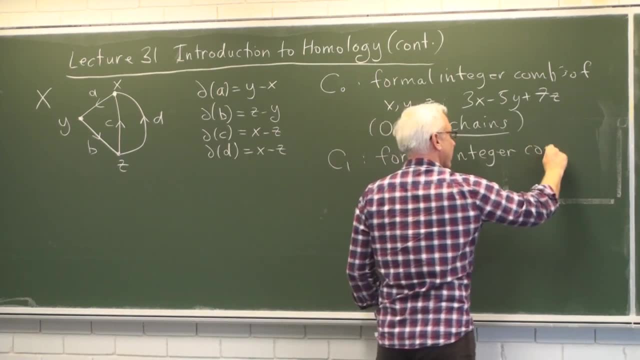 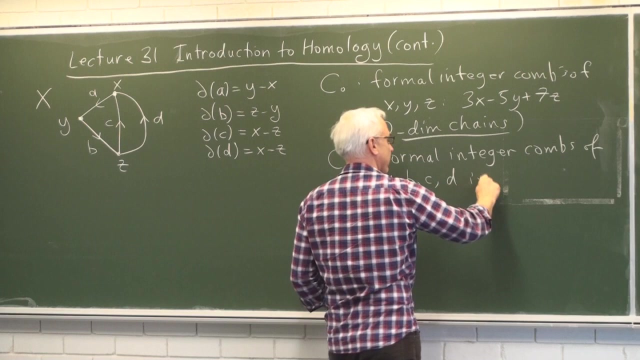 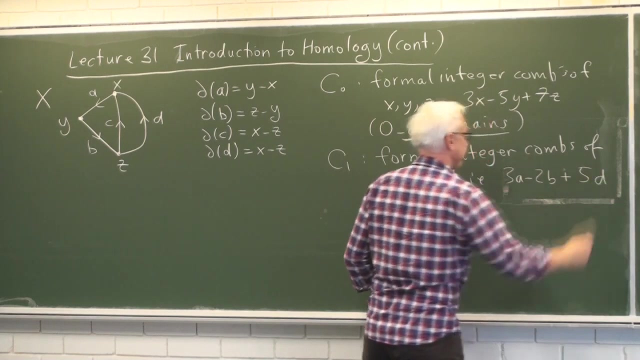 And then we also have sort of one-dimensional version, Formal integrations, Integer combinations of the directed edges A, B, C and D, For example 3A minus 2B plus, say, 5D, And we call these one-dimensional chains. 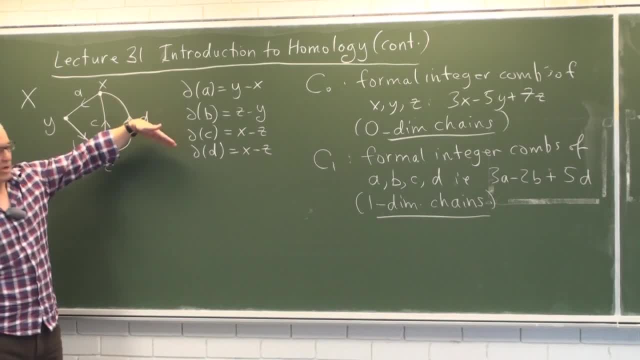 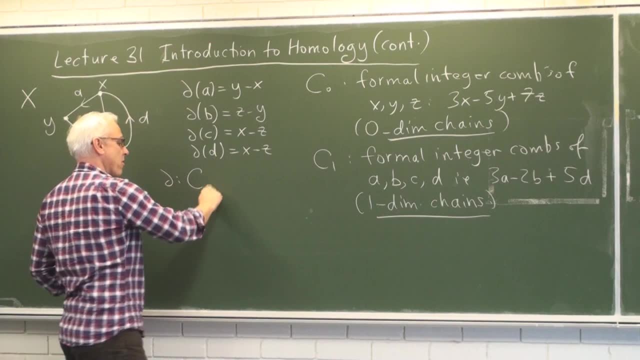 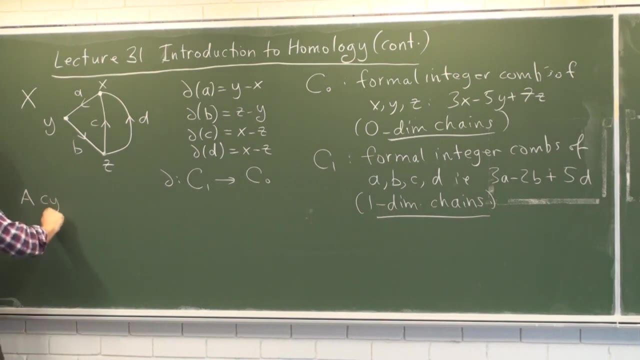 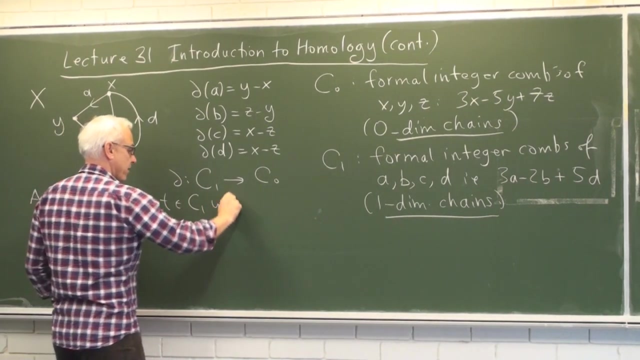 And then what we had is we had this boundary operator. The boundary operator extends to a map or homomorphism from C1 to C0.. And we defined a cycle: in C1 is an element T, in C1 with its boundary being 0.. 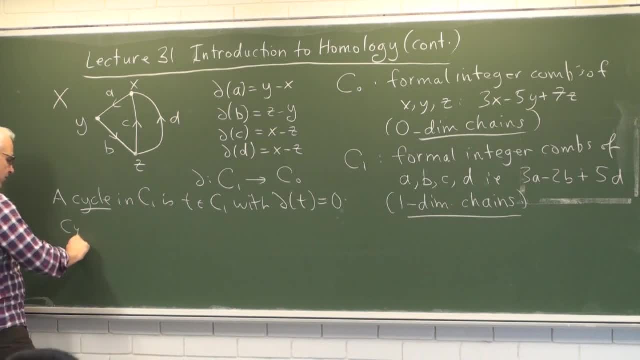 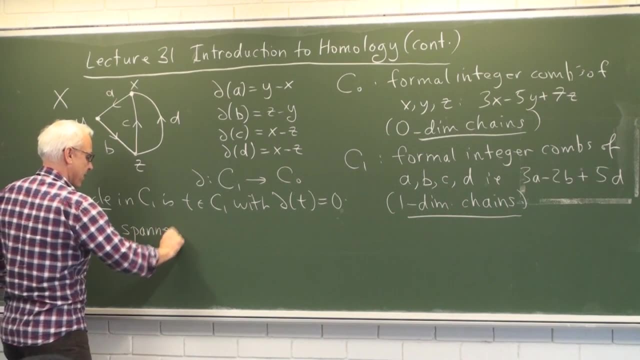 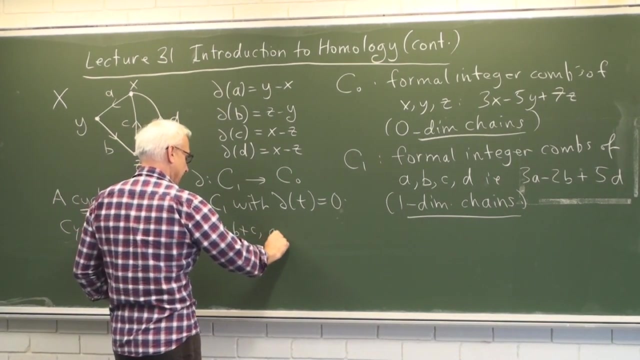 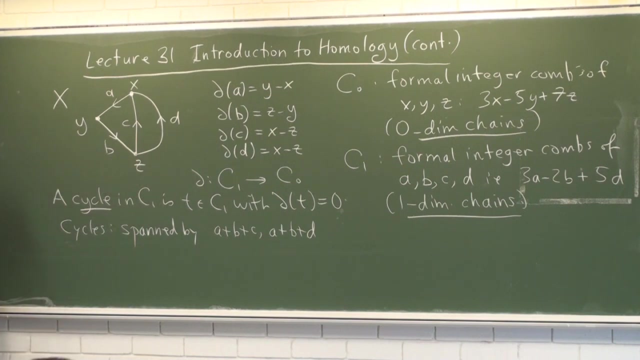 And we found, making a computation, that the cycles were were spanned by, or combinations of two particular cycles. I think we found A plus B plus C and A plus B plus D, So that the other cycle, for example C minus D, was a linear combination of these. 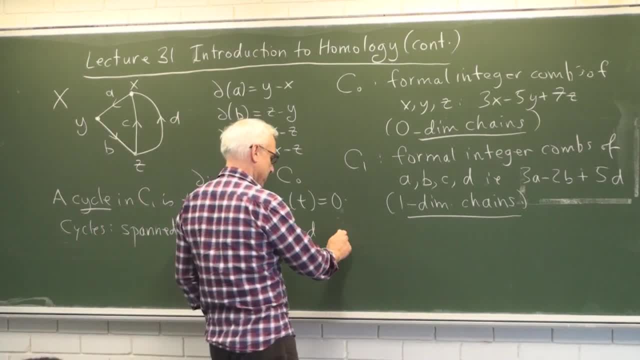 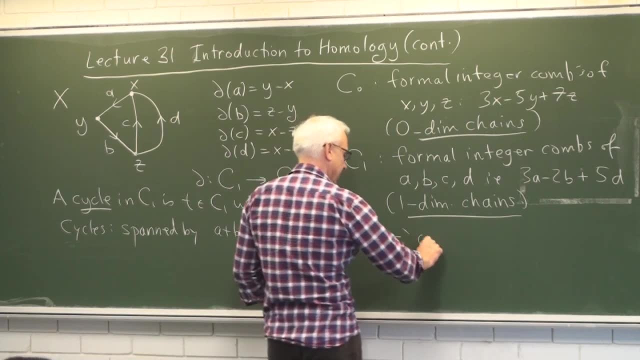 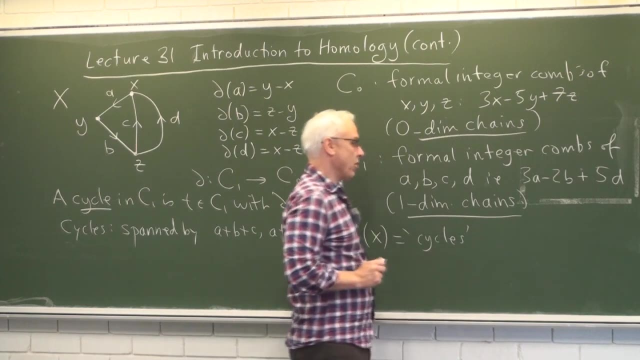 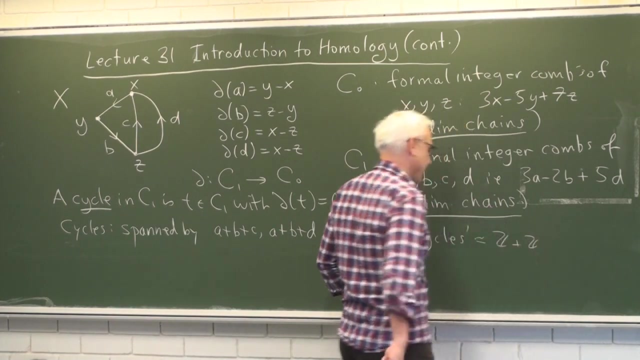 And then we defined, sort of in a preliminary way, preliminary way, The first homology group of the space X to be the space of cycles, Or it's basically the subgroup of the one chains which are cycles, And this is then algebraically the sum of two copies of Z. 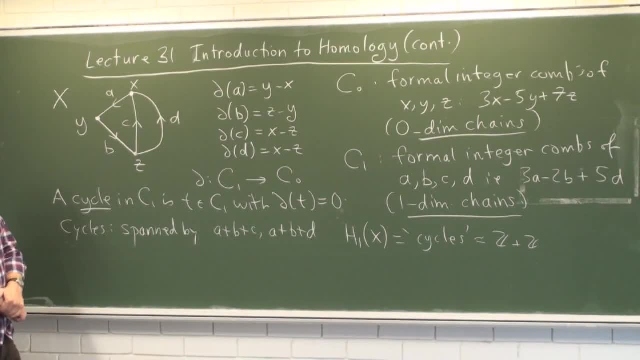 one for each of the generators. This is sort of a preliminary thing, And to make it more clear what's going on and to extend the definition a little bit more accurately, we have to introduce some additional structures now. So we're going to go up in dimensions. 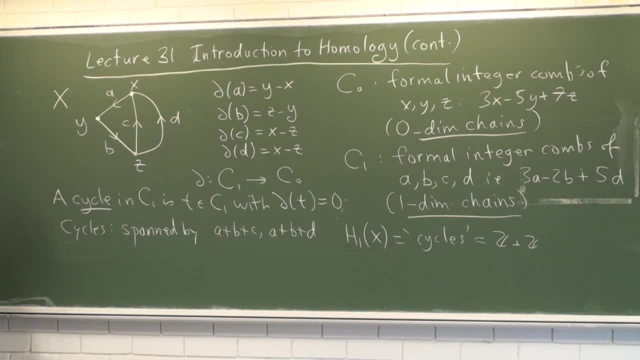 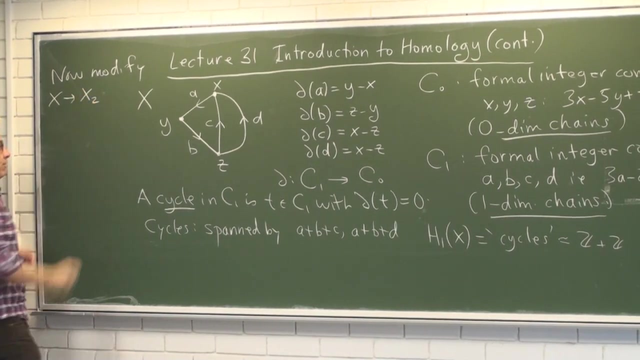 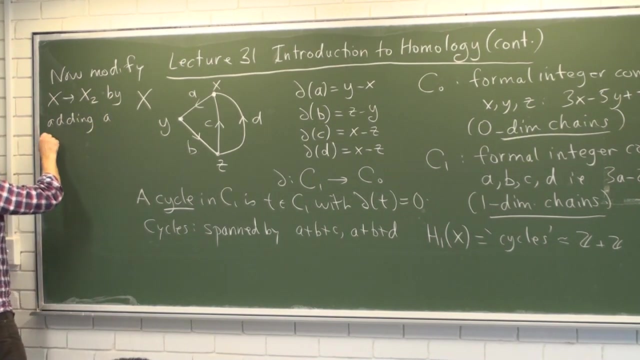 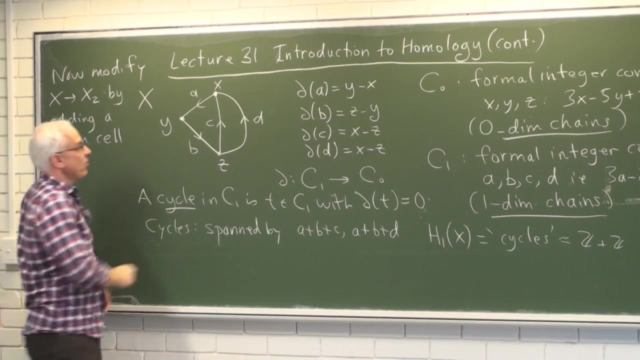 and then we're going to modify this space by adding some two-dimensional cells. Okay, So we're now going to now modify X- Let's send it to say X2.. By adding a two-dimensional cell And the two-dimensional cell that we're going to choose to add. 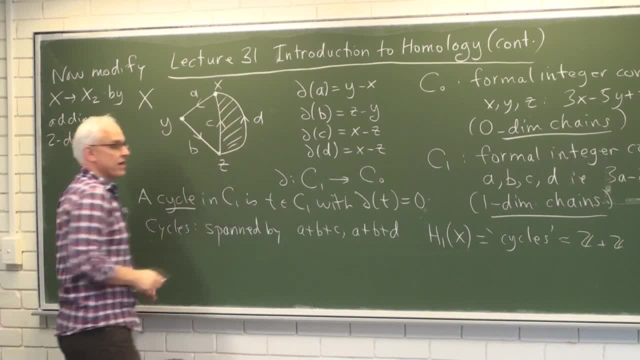 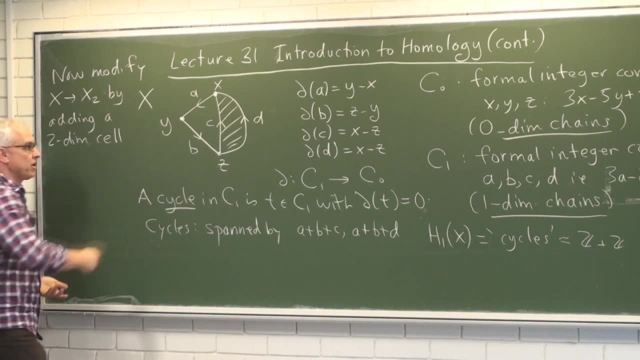 will be right in here. We're going to put in a little plate between these two edges so that we now have a little disk inside there, And we're going to give this disk a name. Let's call it A, So a two-dimensional cell A. 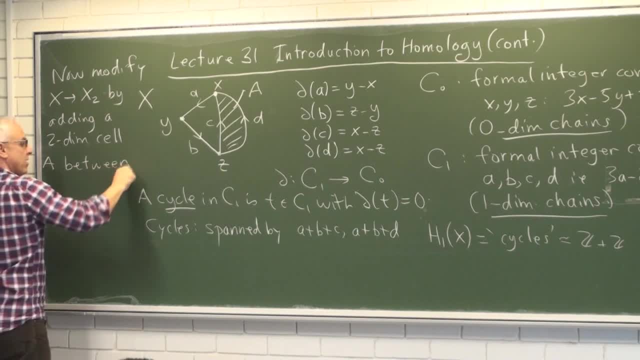 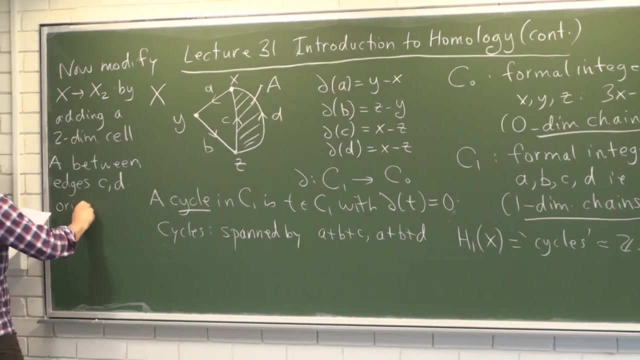 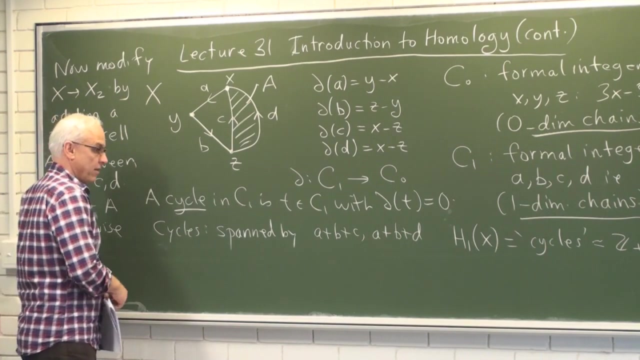 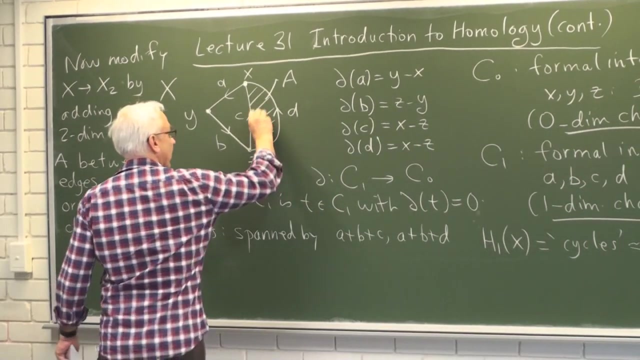 between two-dimensional cells. The edge is C and D And let's also orient this edge. Let's agree that we'll orient A clockwise Meaning that we're going to. we'll think of this two-cell as having an orientation. So, looking down on it, it looks like this: 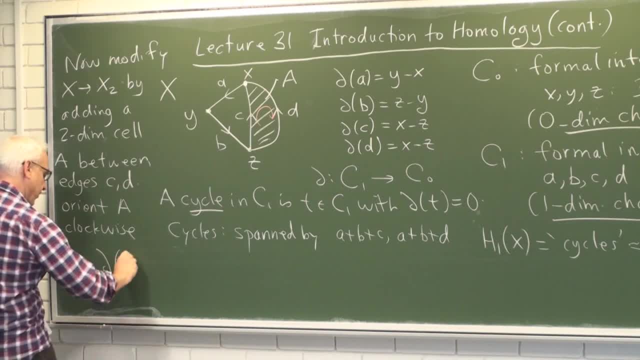 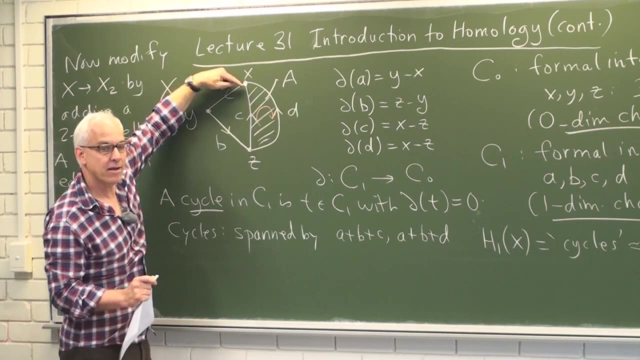 So the boundary. so the boundary of this new cell A consists of C and D, But we agreed that the orientation induces a particular form for the boundary, Namely it's C minus D. The boundary is the loop or cycle going in this direction. here, 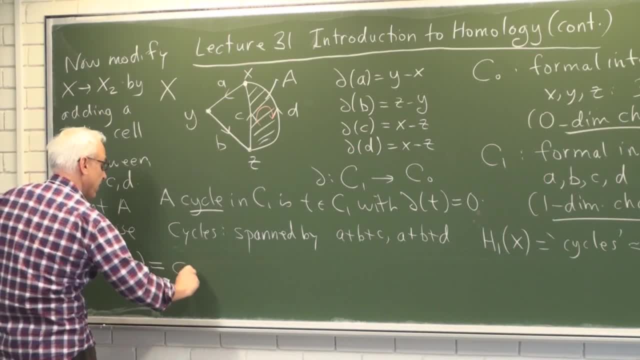 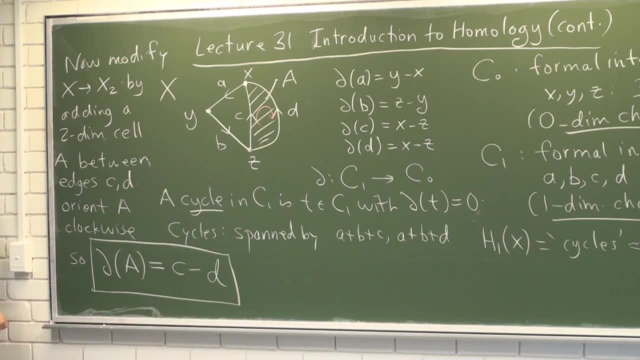 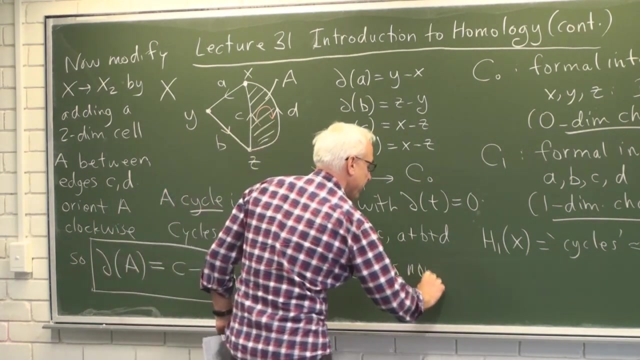 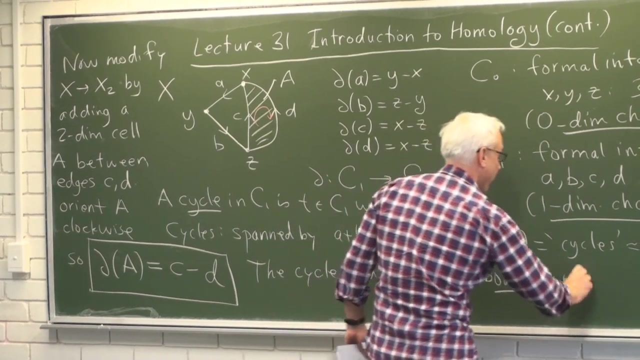 That's what the orientation means. So the boundary of A is, by definition, C minus D. That's one of our cycles. That cycle is now the boundary of this two-cell. So the cycle C minus D is now the boundary of this two-cell. 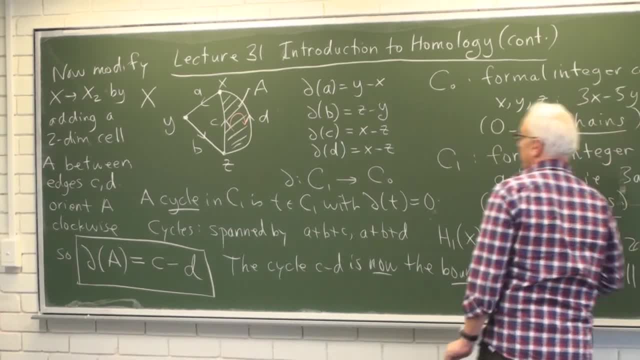 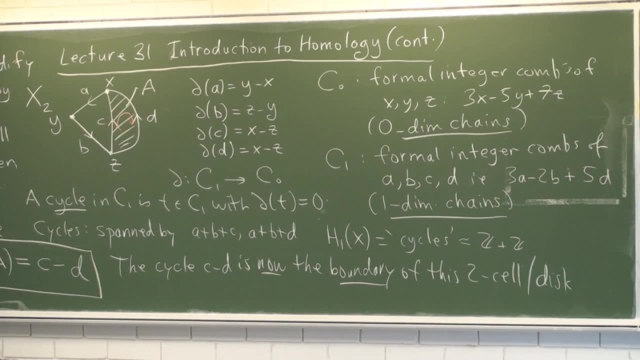 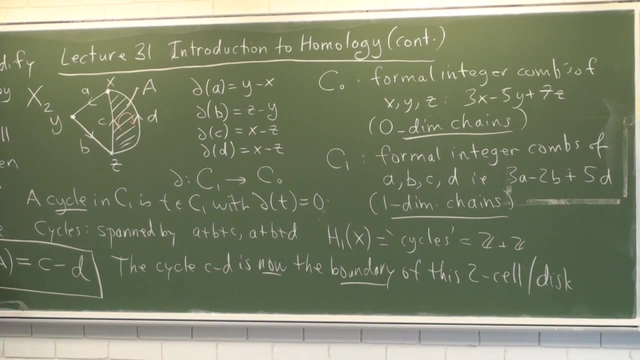 Two-cell is just another name for disk, two-dimensional disk, And let's so. we'll re-label the diagram. This is now X2.. It's a modification of our space by adding this disk. All right, so now what we can do is we have not just zero-dimensional objects, not just one-dimensional objects, we now have two-dimensional objects as well. 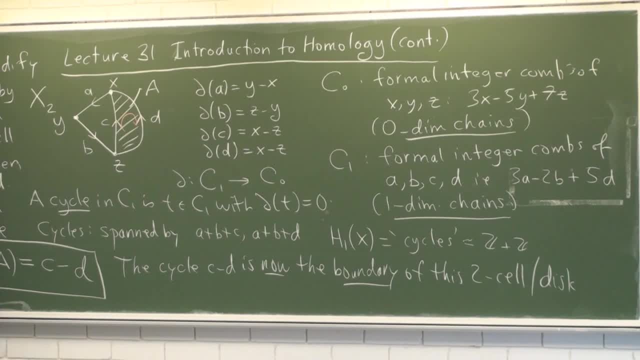 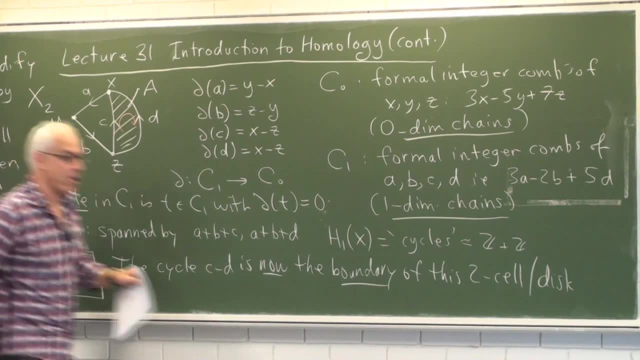 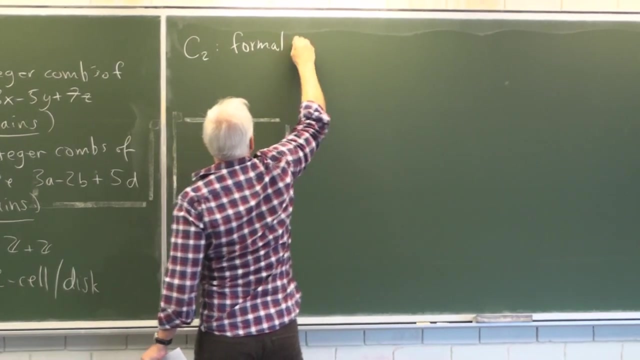 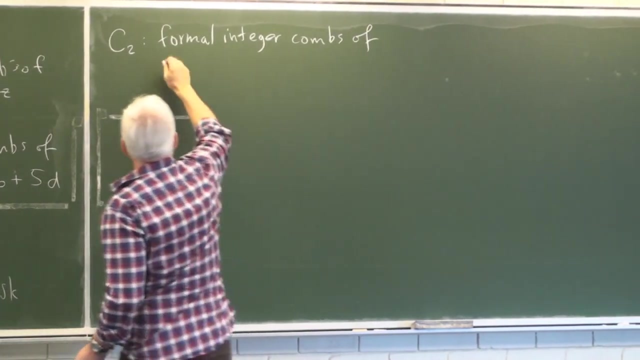 So we need to extend our algebra to consider formal combinations of the two-dimensional objects. In this case there's only one so far, so it's rather modest, But nevertheless we'll introduce C2.. C2, which is formal integral combinations of well, in this case just A. 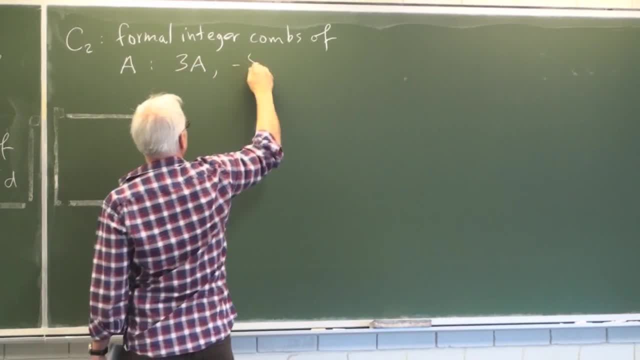 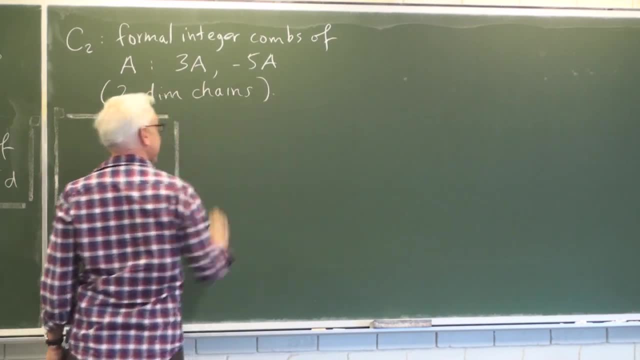 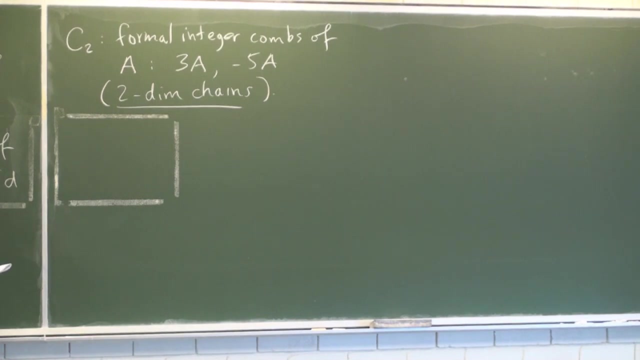 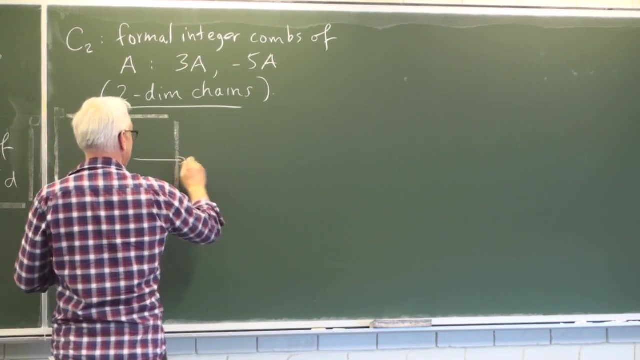 Okay, so things like 3A or maybe minus 5A, And we'll call these things two-dimensional chains. So we have the situation now where we actually have three different groups: We have C2, we have C1, and we have C0. 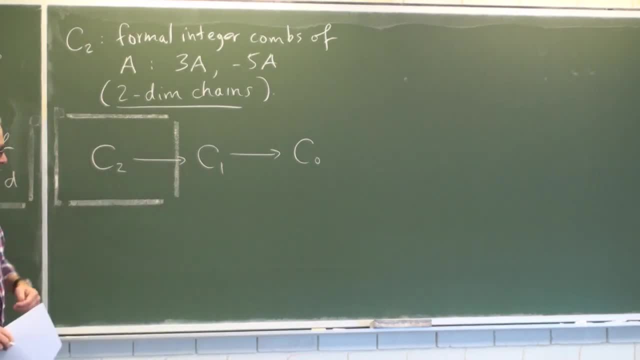 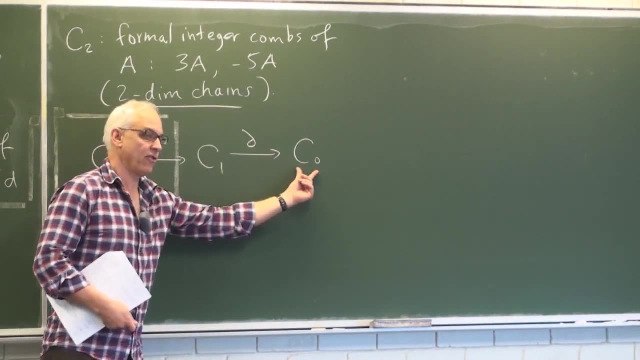 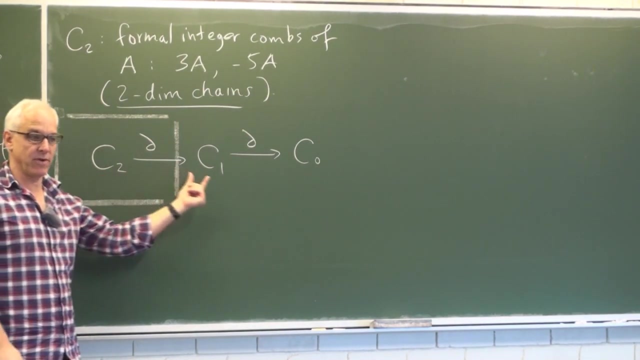 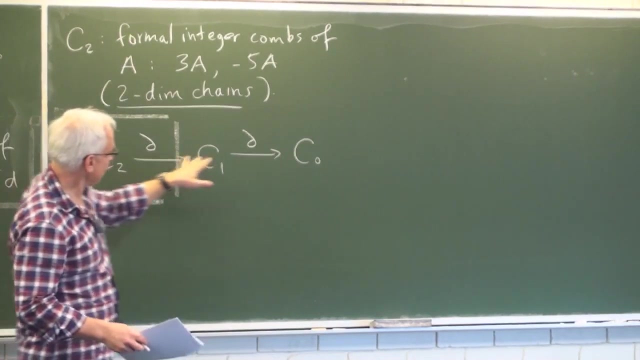 Zero-dimensional chains, one-dimensional chains, two-dimensional chains, And we have boundary maps going not just from edges to vertices, but now also another boundary kind of operator, taking two cells to edges or to combinations of edges. Now it might get confusing if we have these different del operators around here. 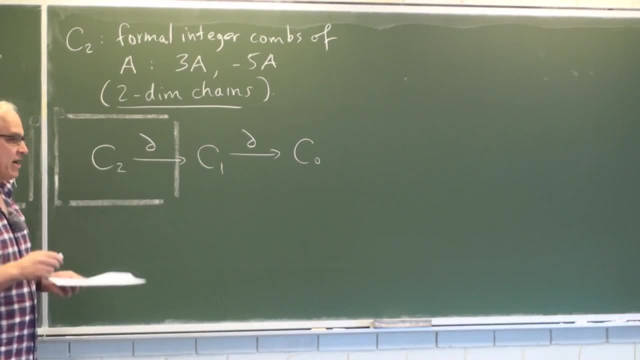 So what we do is we introduce a little bit of notation to make it clear which boundary operator we're talking about. We'll call this one del 1 and this one del 2.. All right, so now we have del 1 going from. 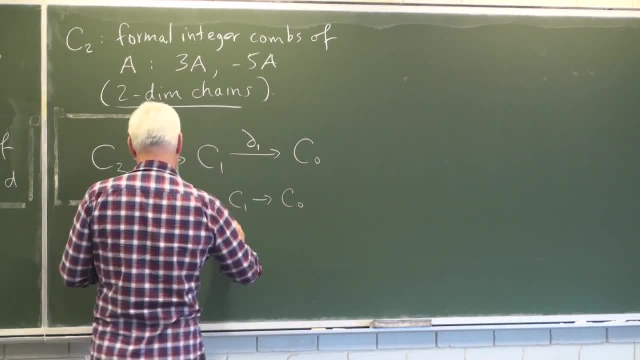 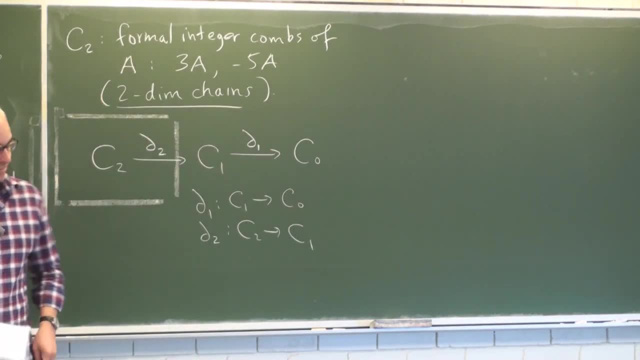 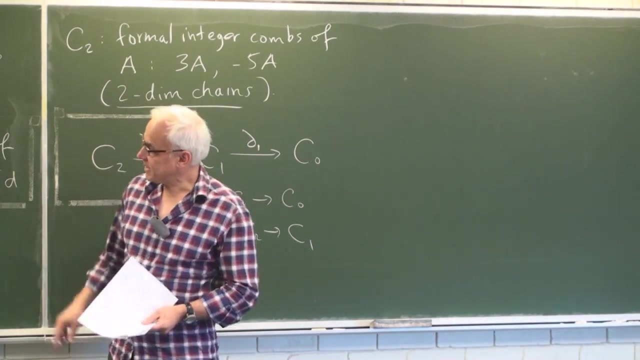 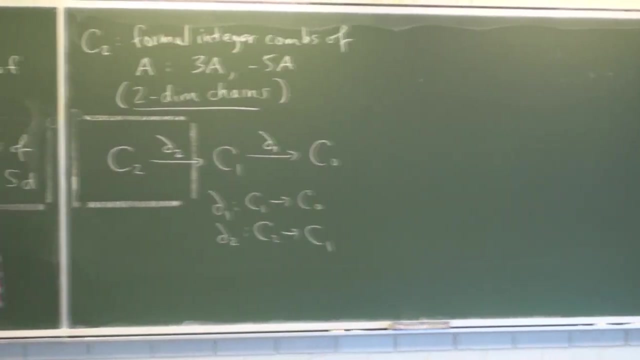 C1 to C0, and del 2 going from C2 to C1.. All right, so now let's see what does the presence of this two-cell do in terms of the cycles that we've established previously. So we've already talked about the cycles in C1.. 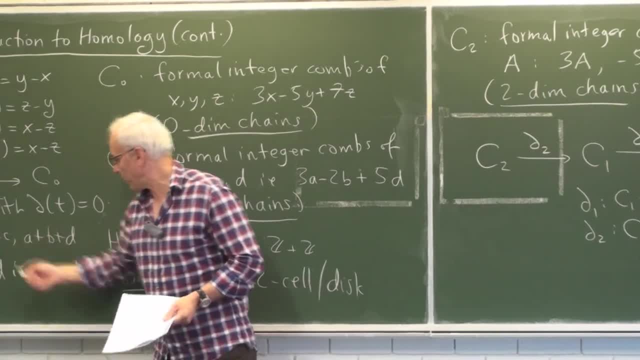 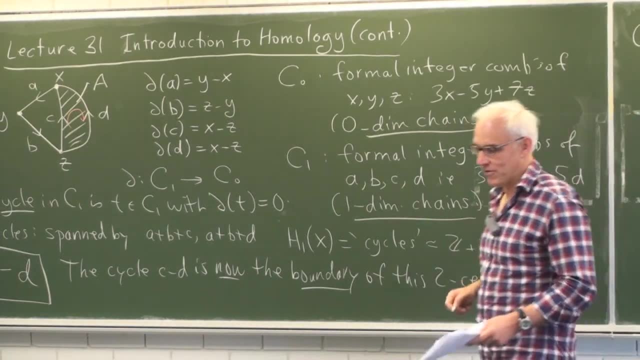 Cycles in C2.. Cycles in C1 are spanned by A plus B plus C and A plus B plus D. But now this new cell that we have here has an effect of creating or sort of reducing a cycle that we previously had to zero. 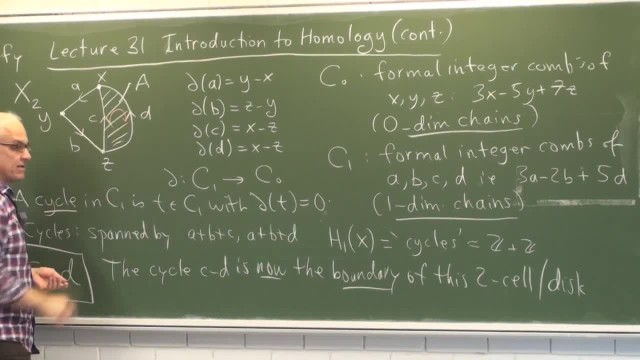 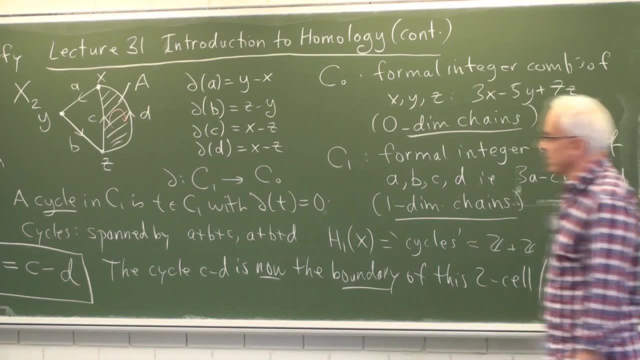 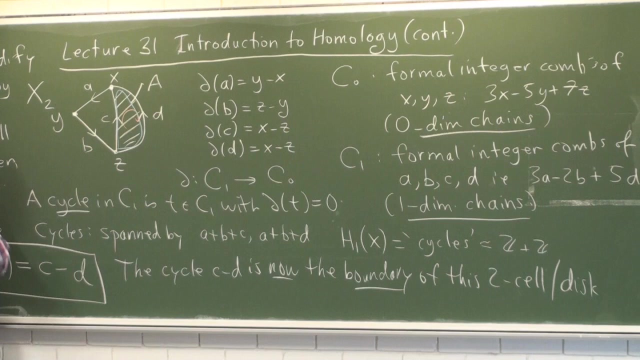 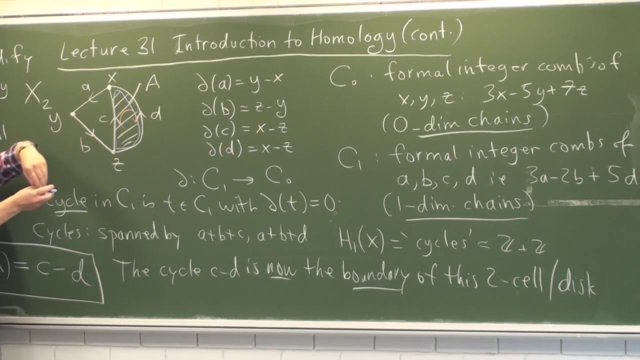 So the cycle that we formerly had, C D, that cycle is no longer really enclosing a whole. So this cycle here that was formerly a legitimate cycle is no longer a legitimate cycle anymore in the sense that it's homotopically shrinkable to a constant. 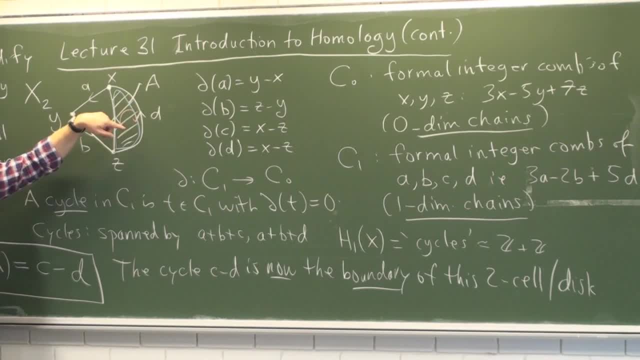 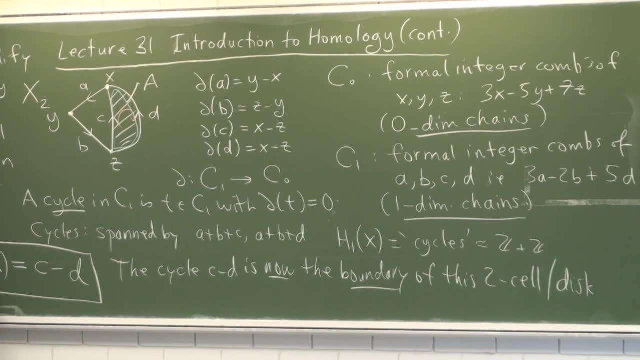 In other words, it no longer surrounds a whole. So the presence of this two-cell means that we have to modify our idea of what a cycle is. Formerly, C minus D was a cycle and it represented a whole. C minus D is still a cycle, but now it does not represent a whole anymore. 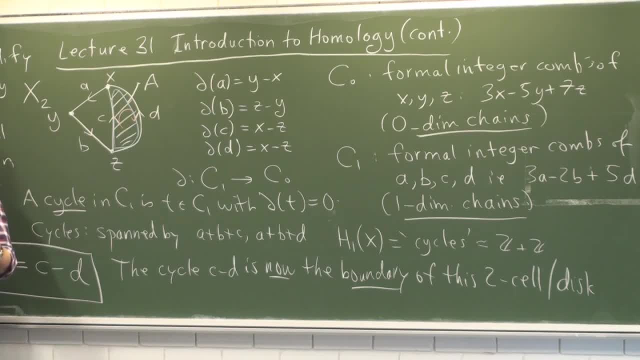 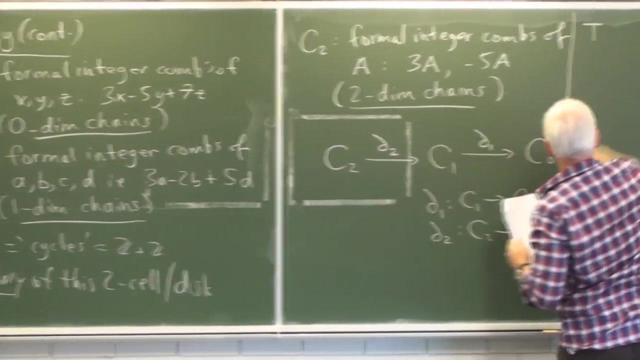 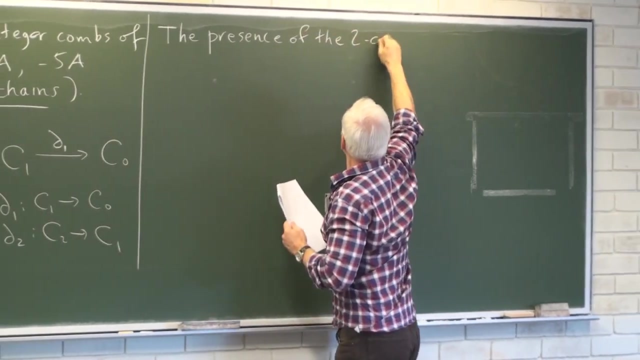 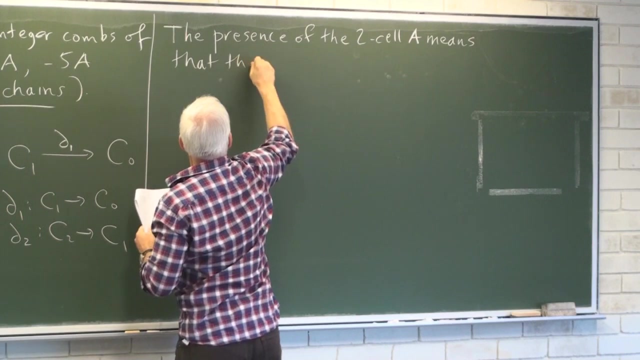 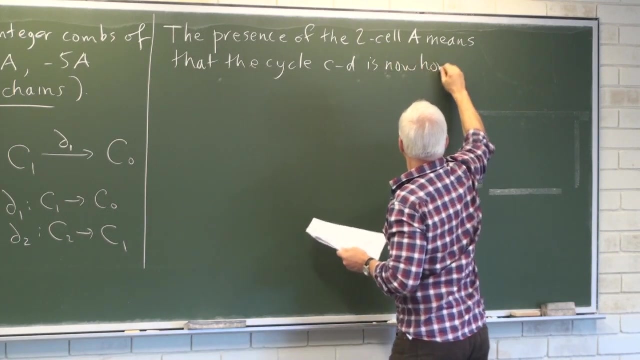 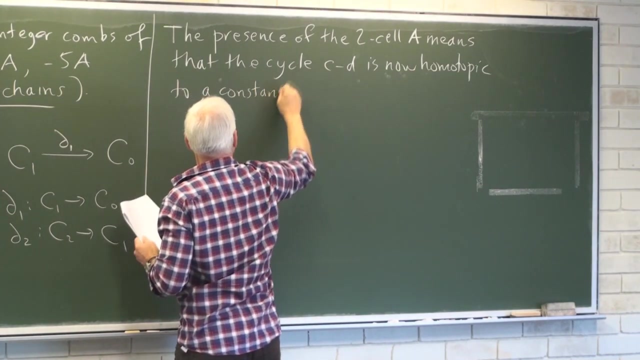 And we want our homology to capture wholes. So it means we have to modify our notion of what the homology is. So the presence of of the two-cell A means that the cycle C minus D is now homotopic to a constant, namely a zero. 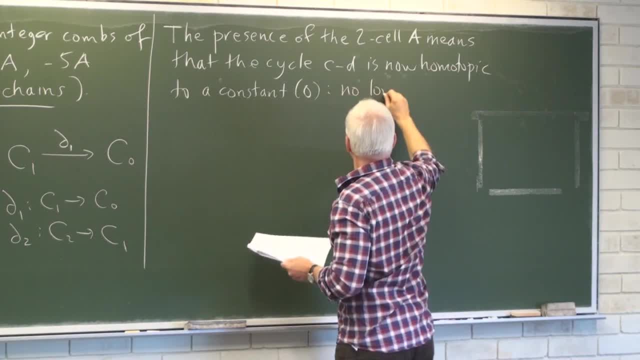 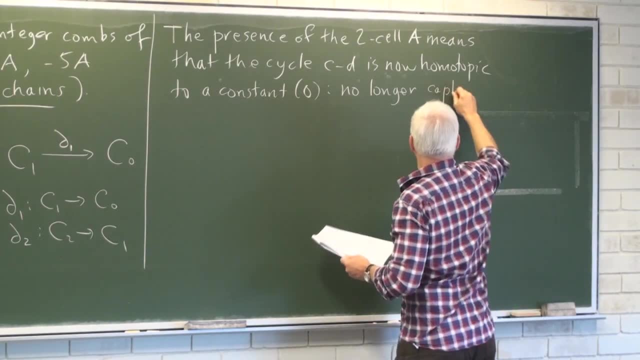 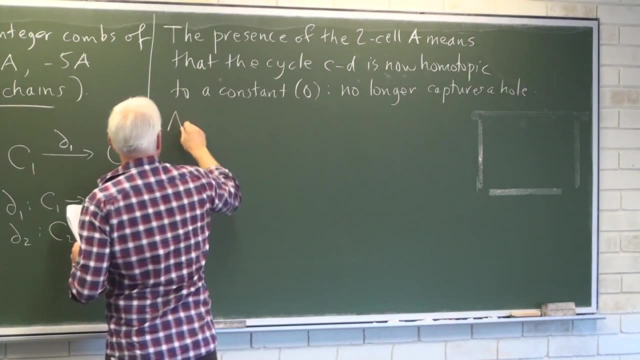 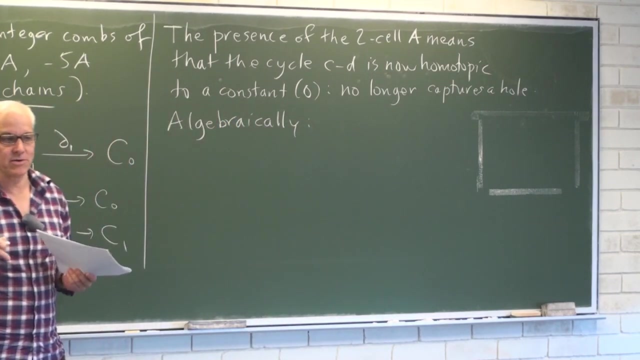 So it really it no longer. it no longer. it no longer goes around a whole or captures a whole. So algebraically, what this means is we actually now want to consider C minus D to be zero as far as measuring wholes goes. 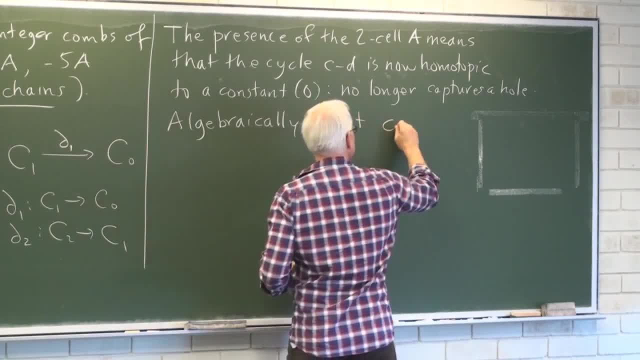 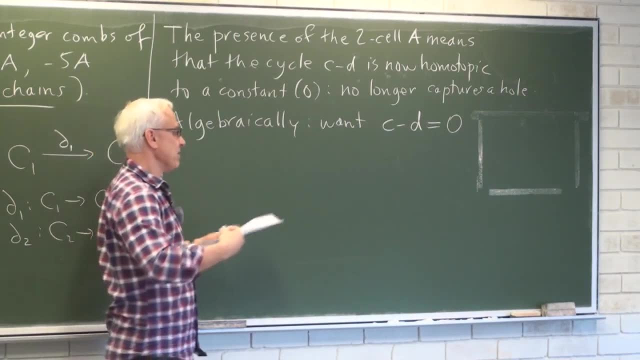 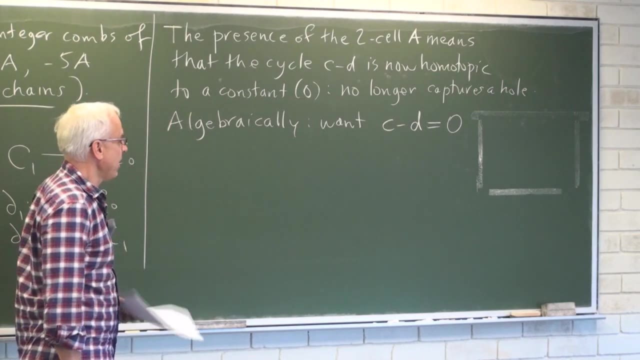 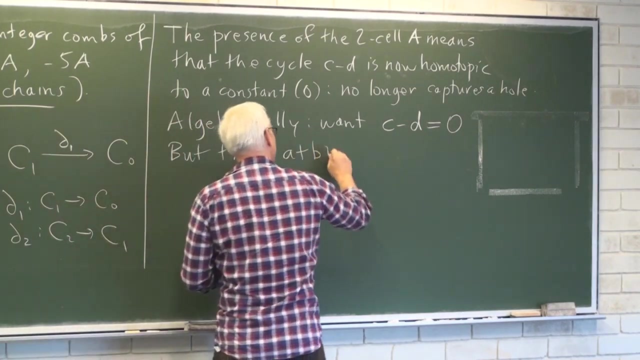 So we want C minus D to be zero. in homology, In other words as far as measuring one-dimensional wholes, C minus D should not count anymore. But then if C minus D is zero, then the two generators that we have, A plus B plus C. 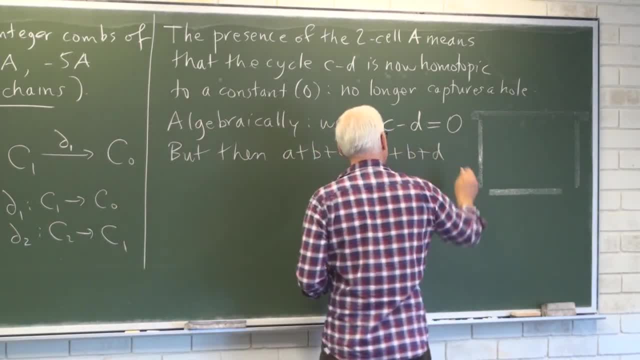 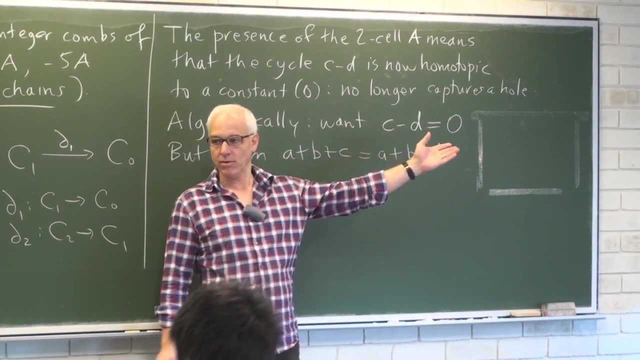 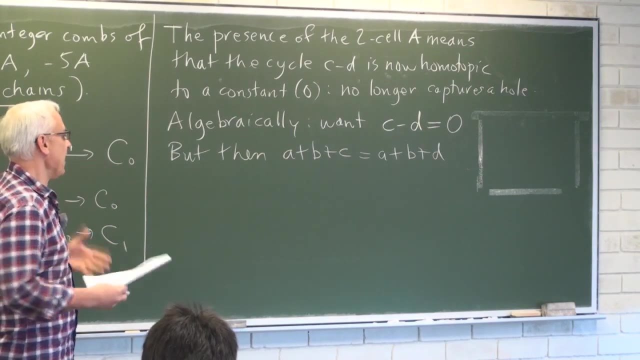 and A plus B plus d are now going to be equal. They're now going to be equal because their difference is c minus d, which is zero. So how do we say what we're doing algebraically here? Well, what we're doing is: 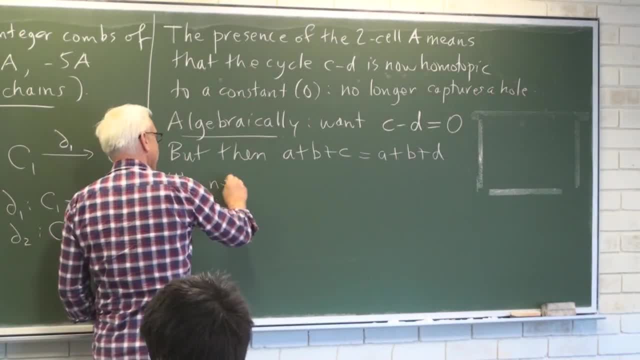 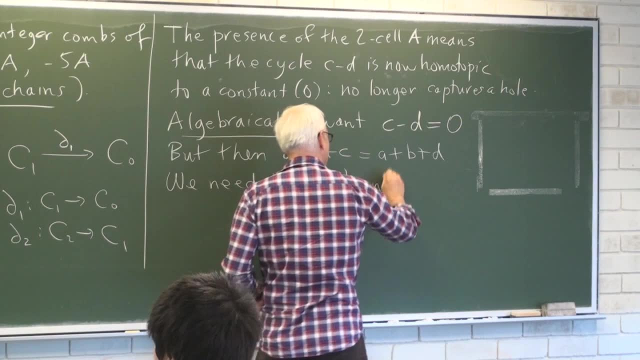 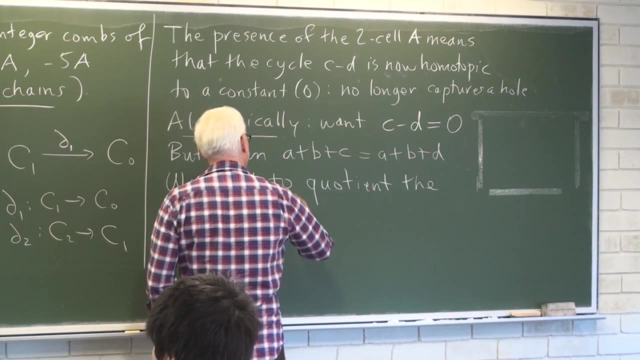 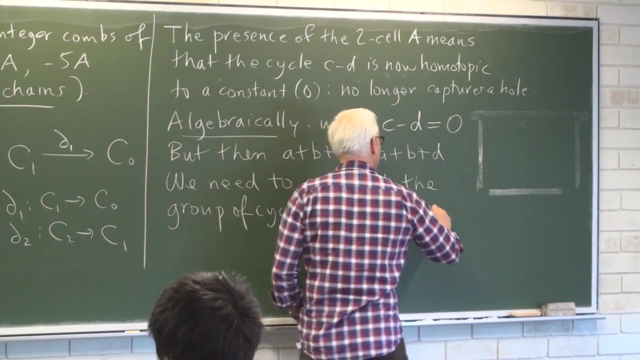 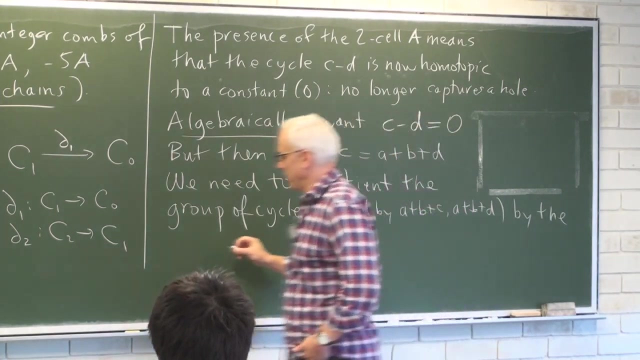 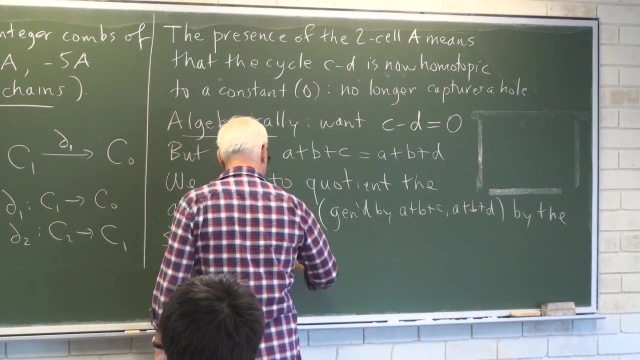 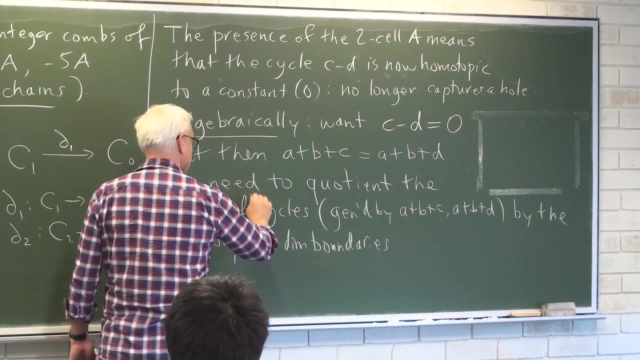 we're, or what we need to do is we need to quotient the group of cycles which was generated by a plus b plus c, together with a plus b plus d, by the subgroup of one-dimensional boundaries- Maybe I should put one-dimensional cycles here. So we need 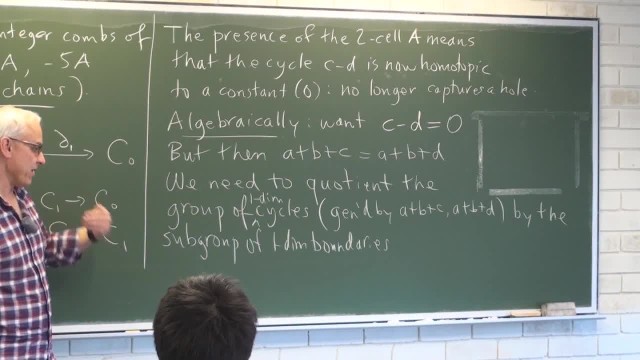 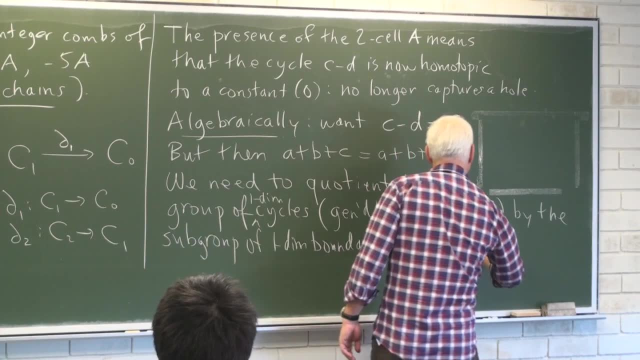 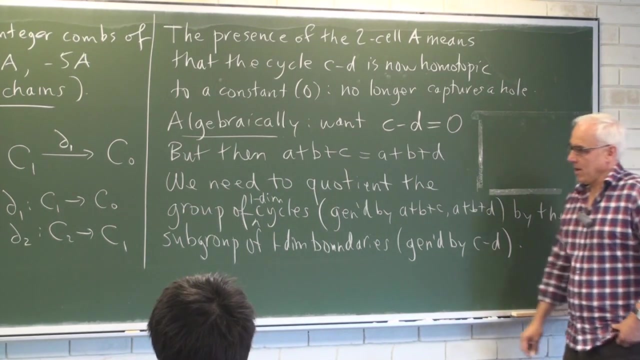 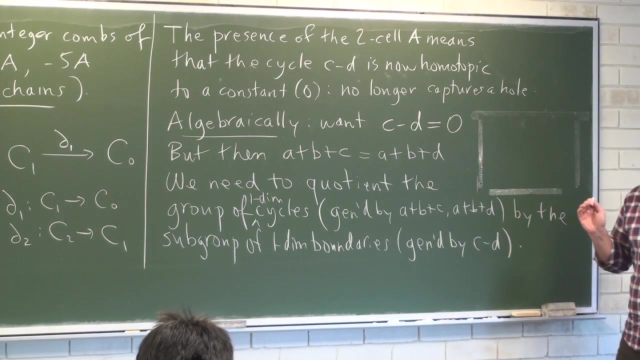 to quotient the group of one-dimensional cycles by the subgroup of one-dimensional boundaries, namely generated by c minus d, And that's in fact how we're going to define the homology. The homology is not just cycles. It's what you get when you take cycles and you sort of disregard boundaries or mod out by 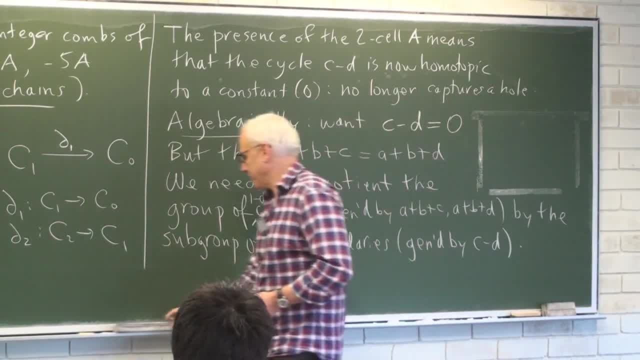 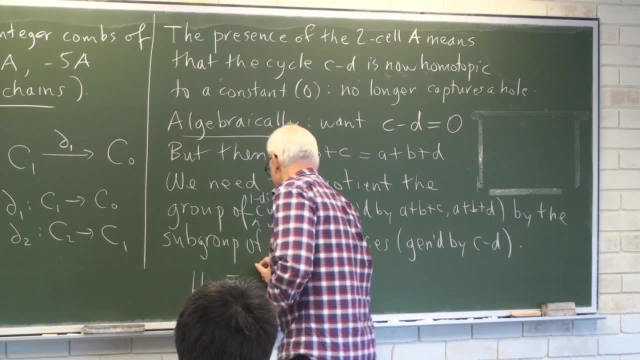 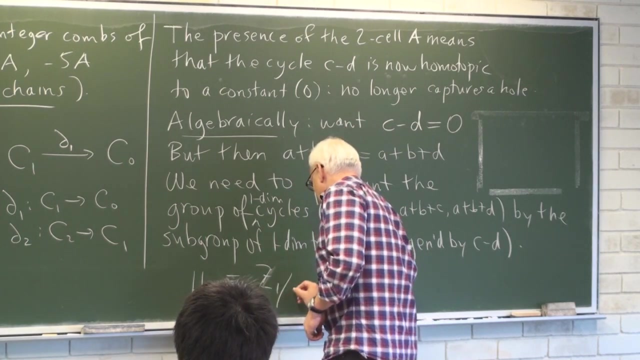 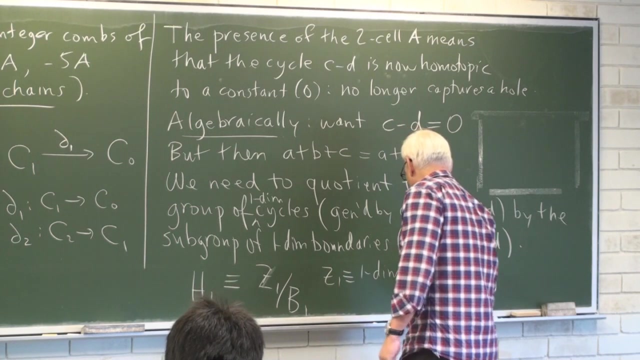 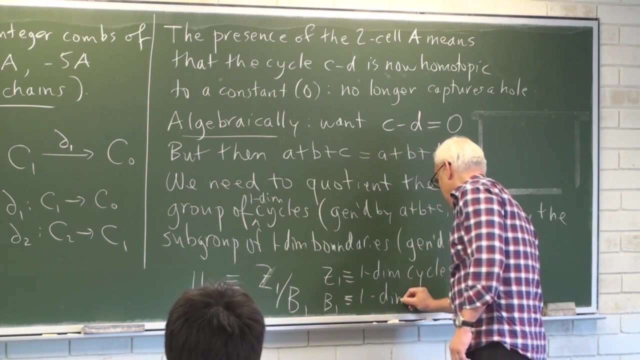 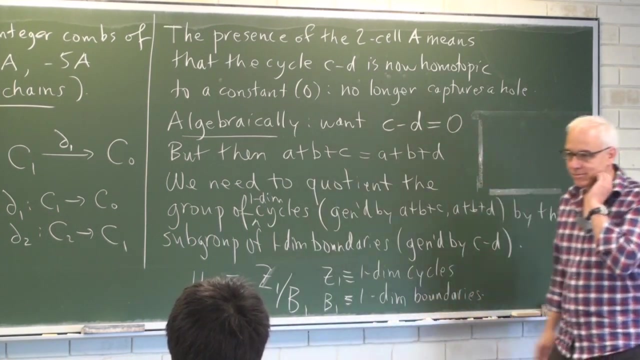 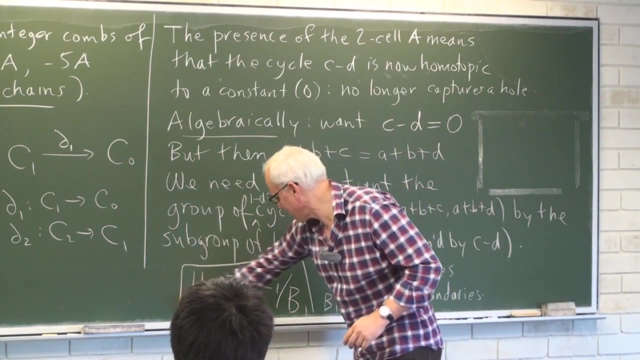 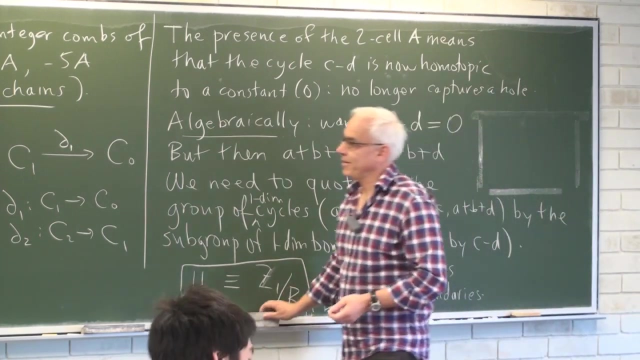 boundaries. So maybe I'll write this equation: that h1 is going to be theка for one-dimensional, to be, by definition, z1 divided by b1, where z1 is one-dimensional cycles and b1 is one-dimensional boundaries. Well, when we do that in our example, the homology shrinks so from going. so the homology of 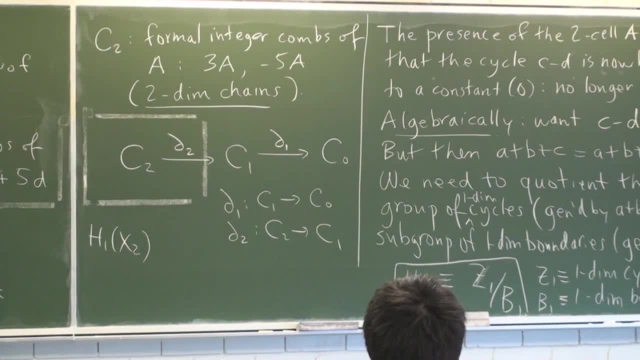 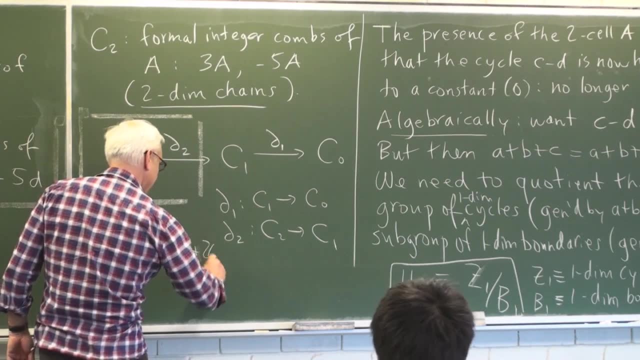 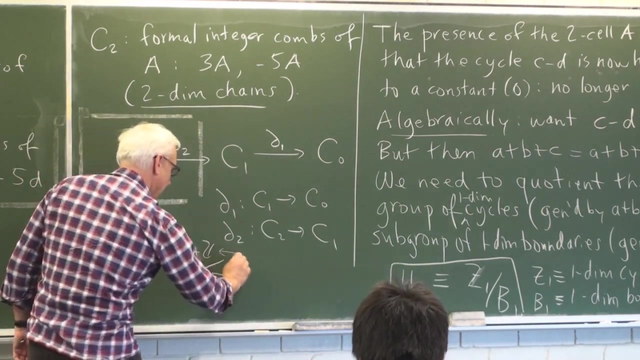 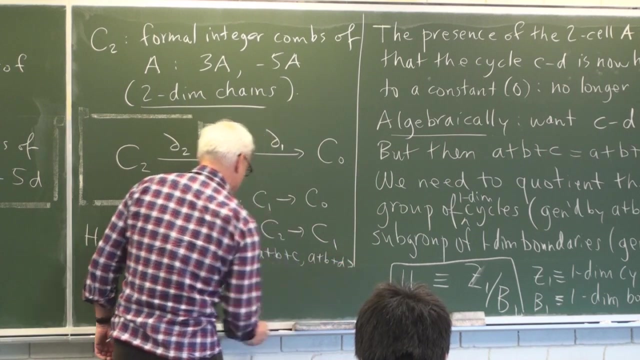 this new space x2,, the h1, is. then we started with the cycles, which was z plus z, and now we're modding out by the boundaries, which are z. So the top here represents the group spanned by a plus b plus c and a plus b plus d, and 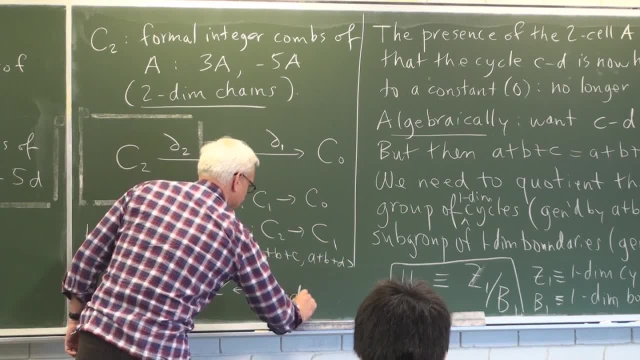 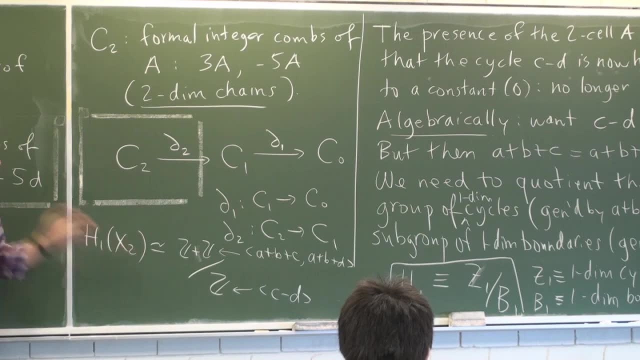 the bottom group is the span of c minus d. So those are the cycles And we're modding out by the boundaries and that's how we define the homology. So in this case, here that's going to be just an isomorphic to the group z. 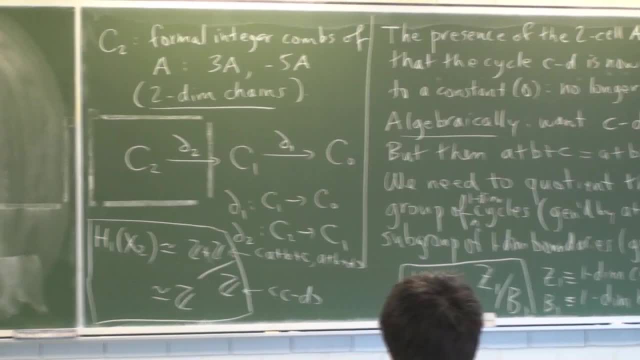 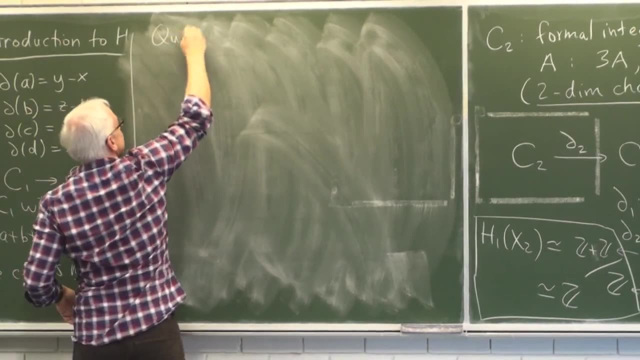 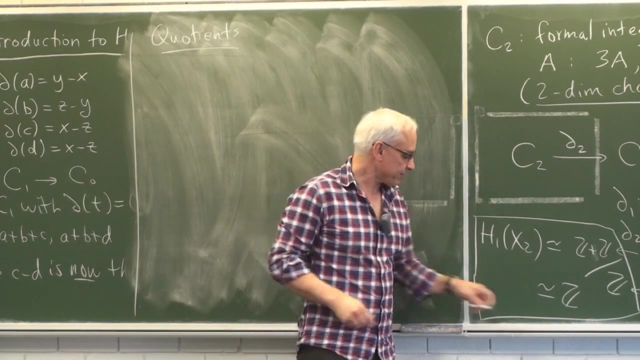 All right, let me remind you a little bit about taking quotients. So we're talking about taking quotients in the commutative setting. So quotients is a little bit different. It's called commutative. It's a tricky thing sometimes, so it's probably worth reminding you that there's a very familiar 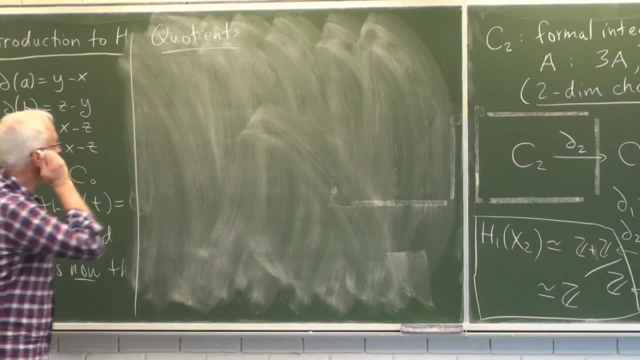 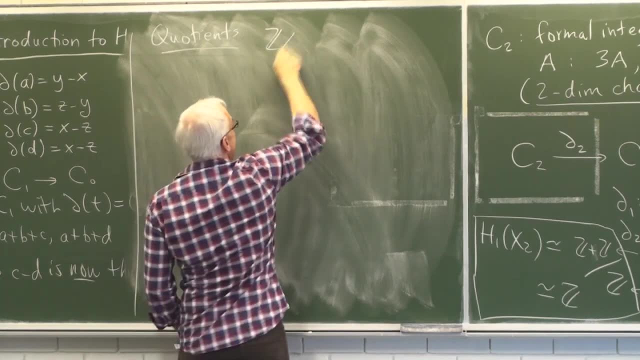 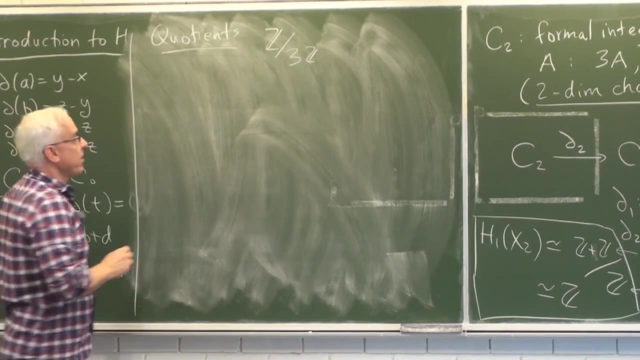 example of taking a quotient which you should keep in mind. So the simplest example of a quotient is probably what you get when you take the integers and you mod out by a subgroup, like say 3z, And what you can think about here is this: 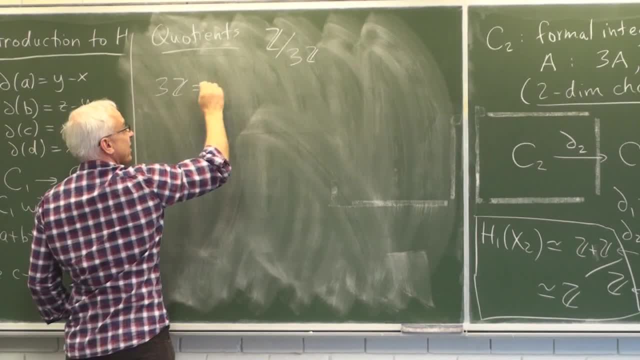 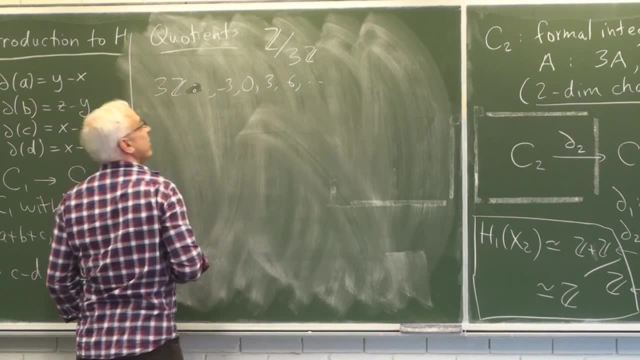 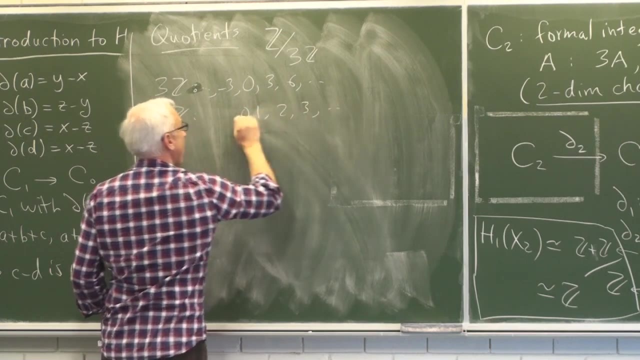 So if 3z is just the Multiples of 3, say 0,, 3,, 6, minus 3, and so on, inside z, which is just all the integers, That's a subgroup of z. 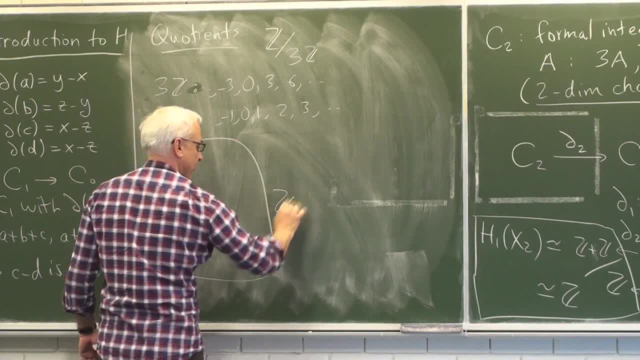 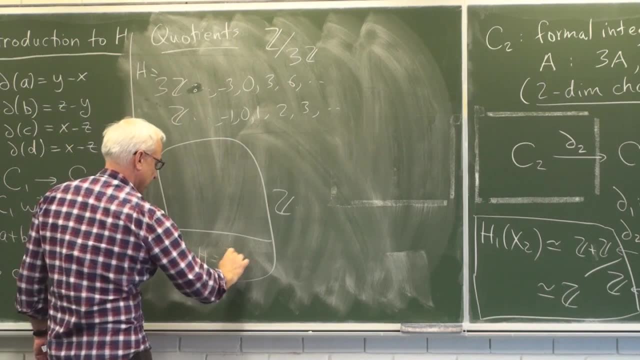 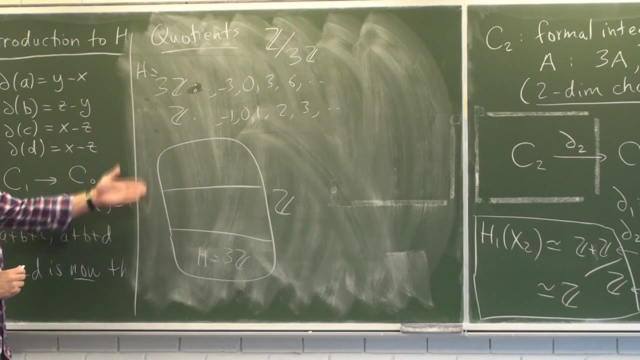 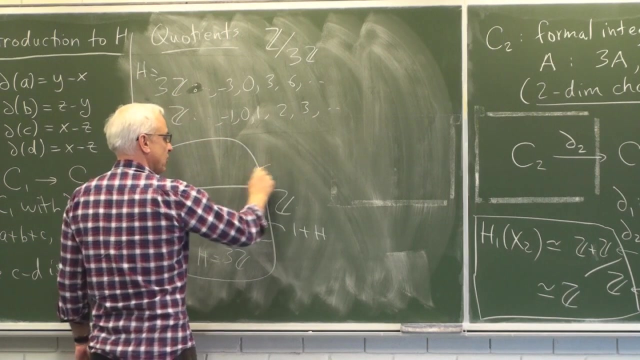 Then if we draw sort of a picture roughly of their z, and here's this subgroup, Let's call it h, Here's the subgroup h, which is 3z, Then it has these two cosets. okay, The cosets of h in z are the cosets well, 1 plus h and 2 plus h. 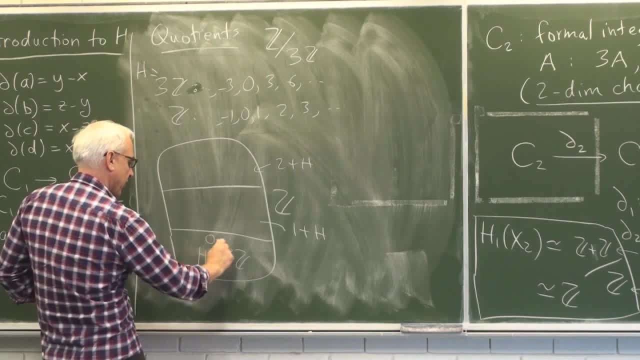 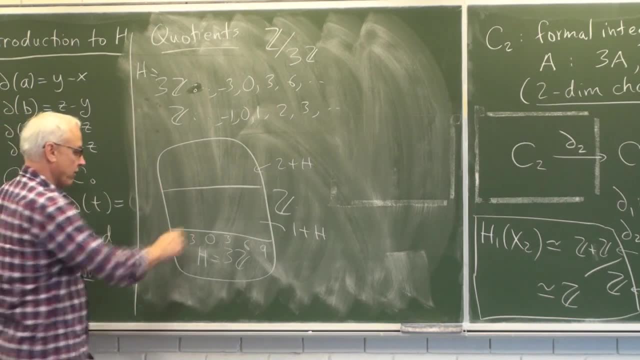 So if this is all the multiples of 3, like 0,, 3,, 6,, 9, minus 3, and so on, then 1 plus h is what you get when you add 1 to all of those. 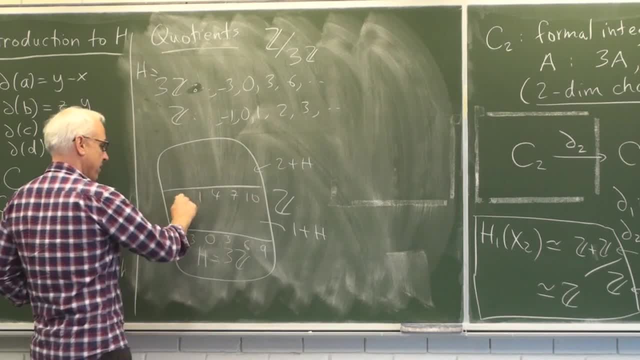 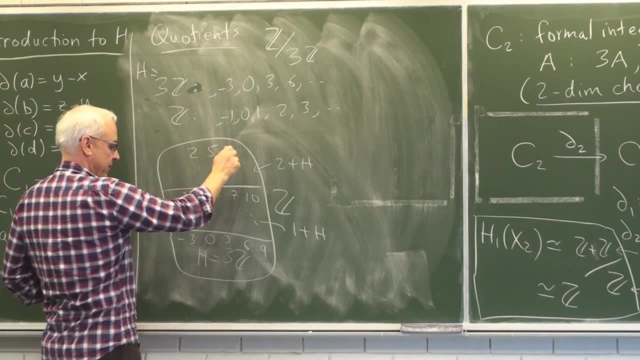 So 1,, 4,, 7,, 10, minus 2, and so on, and 2 plus h is what you get when you add 2 to all of these, 2,, 5,, 8,, 11, minus 1, and so on. 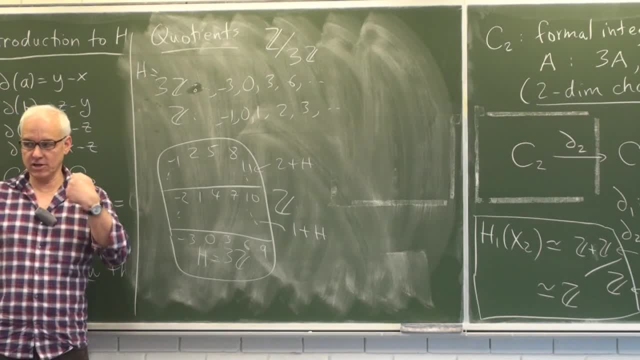 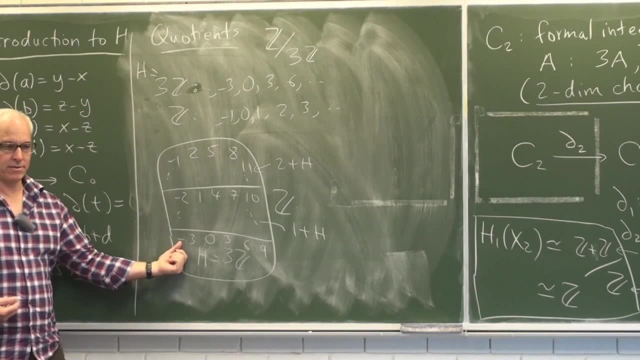 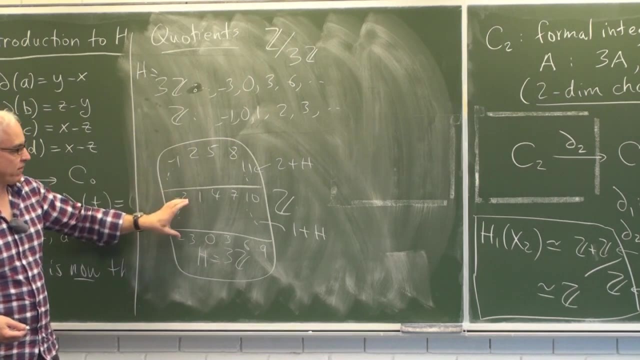 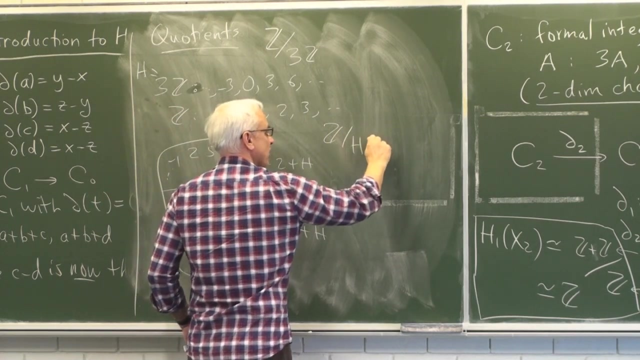 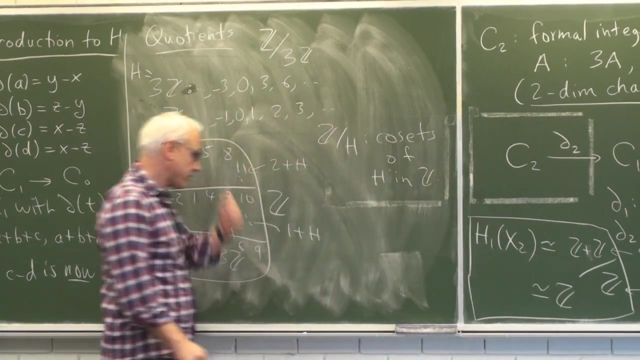 So what we're doing when we're doing a quotient algebraically is we're regarding all of these elements as essentially one object. So the quotient has three objects, namely the cosets of h in z. So I remind you that in this case z mod h is just the cosets of h in z. 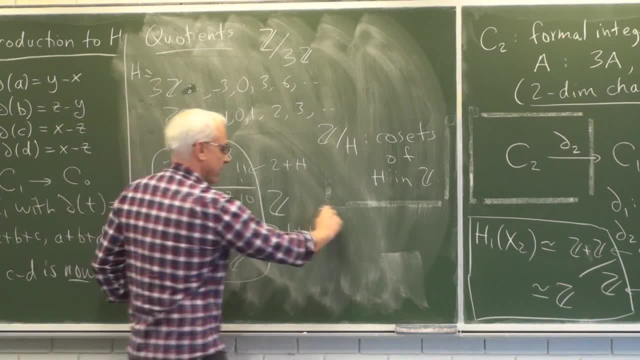 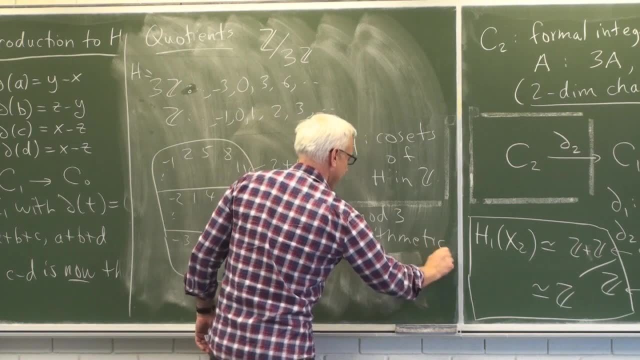 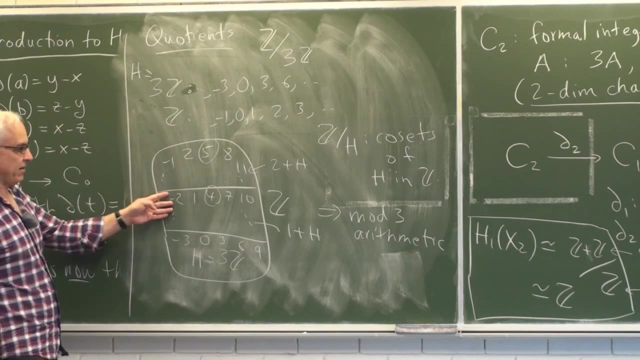 And this is the, this is really mod 3 arithmetic, Gives us mod 3 arithmetic. Okay, So that if we want to add 4 and 5, so if we want to add this coset and this coset, 1 plus. 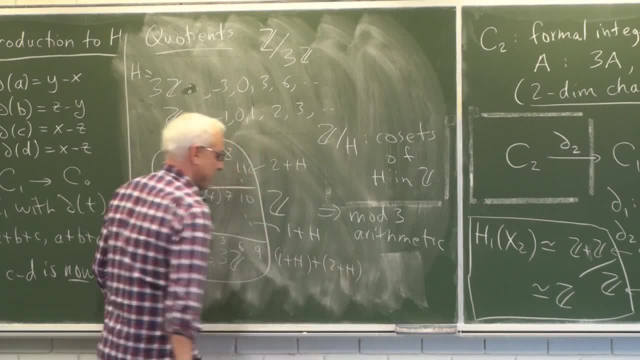 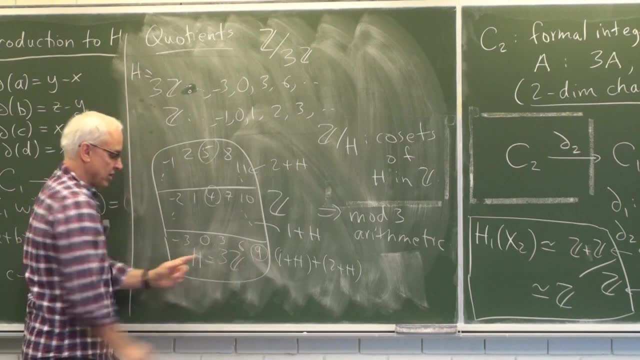 h plus say, 2 plus h, then we can add any two representatives. We can choose 4 and 5 and add them. If we add them, we get 9, which is in this coset, And it doesn't matter which ones we do. 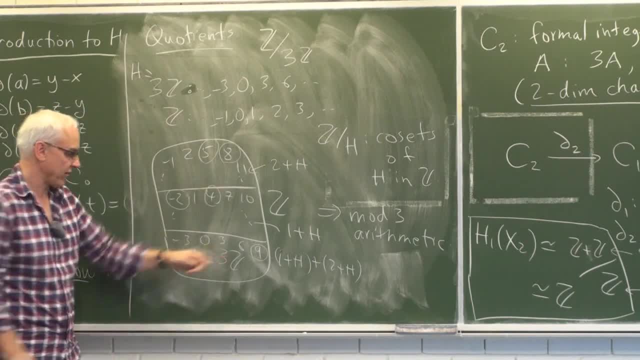 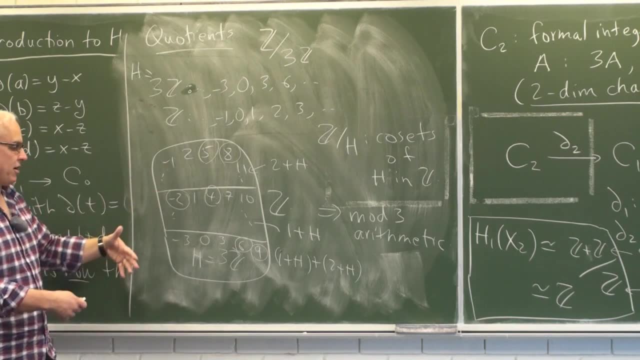 If we choose this one and this one minus 2 plus 8 is 6.. Any one in here plus any one in here gives us one in here. So the addition descends to addition of these cosets. So this would just be h. 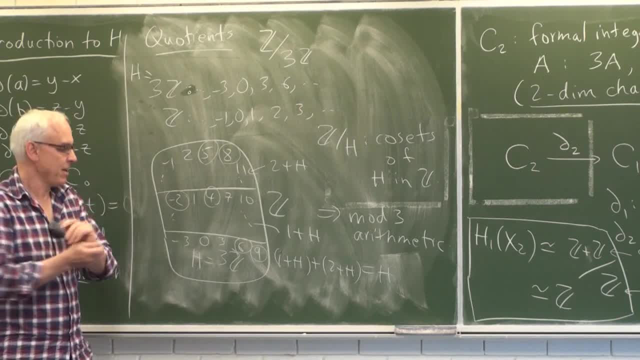 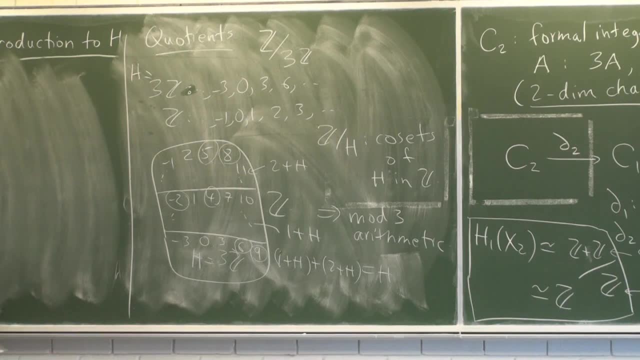 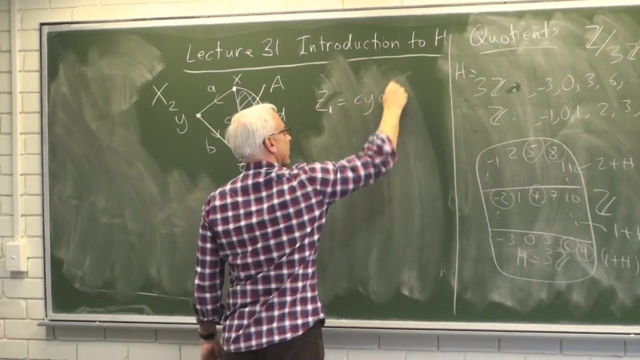 All right. So that's the same kind of thing that we're doing here. Okay, And with this homology, we are Okay. We're looking here at the cycles, which is z1, which is the cycles. What is this? 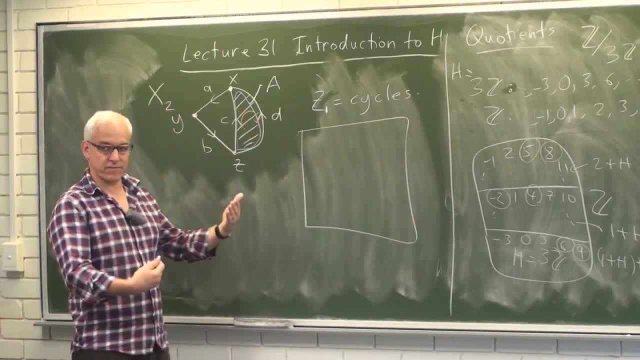 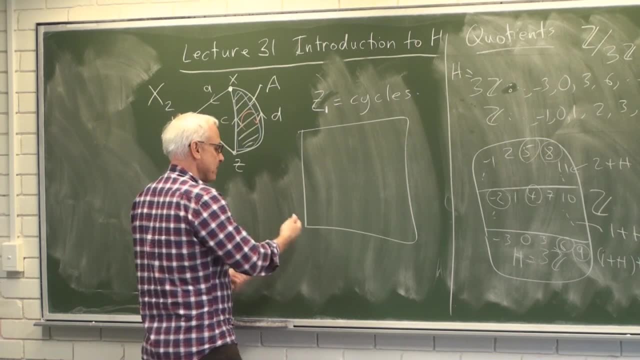 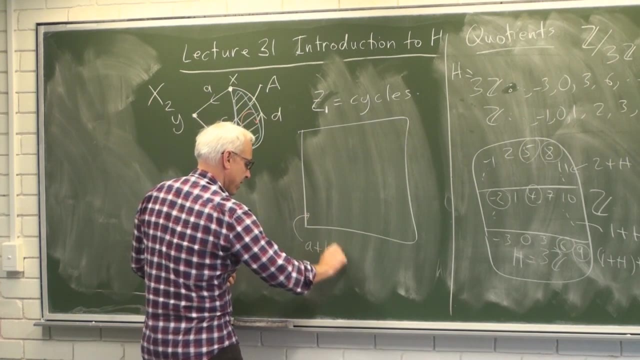 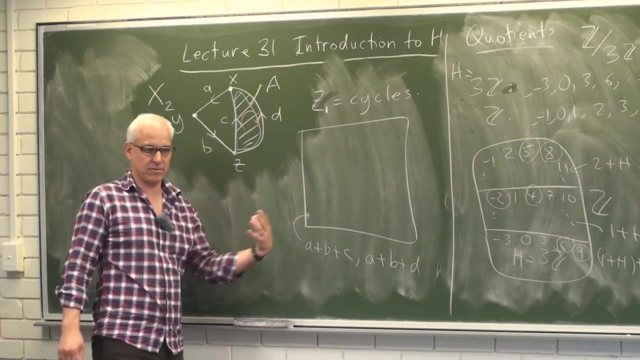 This is a subgroup. Well, this is the subgroup of one chains that basically- okay, in this case just consists of multiples of a plus b plus c. Okay And Okay. Okay, And a plus b plus d, So combinations of these two things. 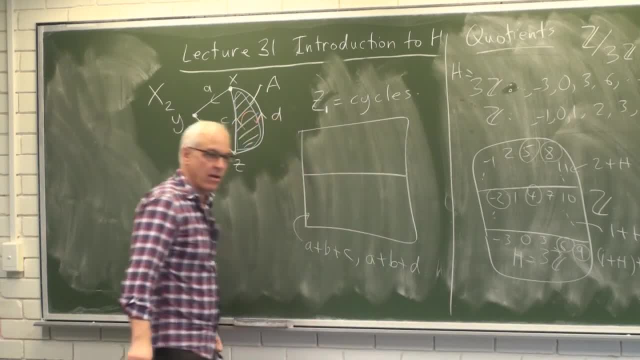 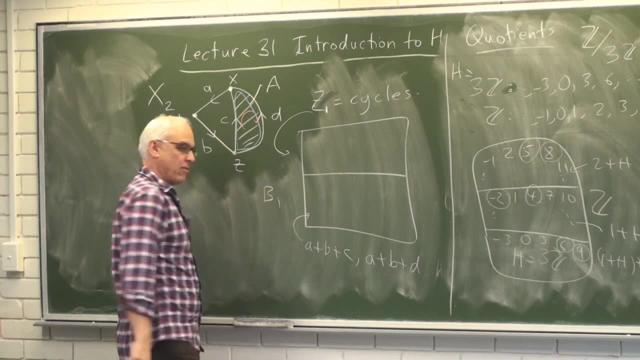 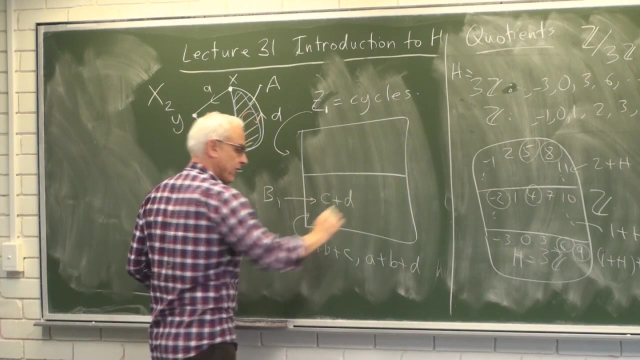 What we're doing now is identifying inside here a subgroup. So this is all of z1. And inside here we have b1, which is a subgroup of boundaries. Inside here is just all multiples of c plus d. Okay, So what we're now doing? 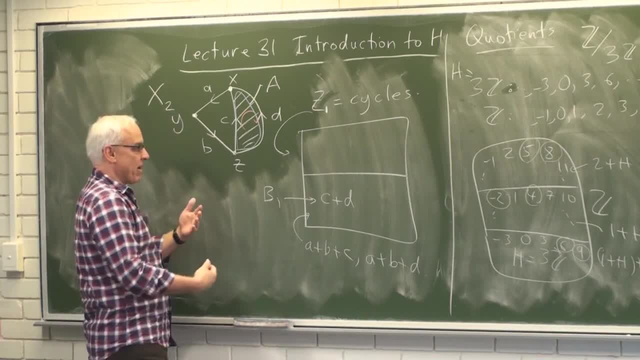 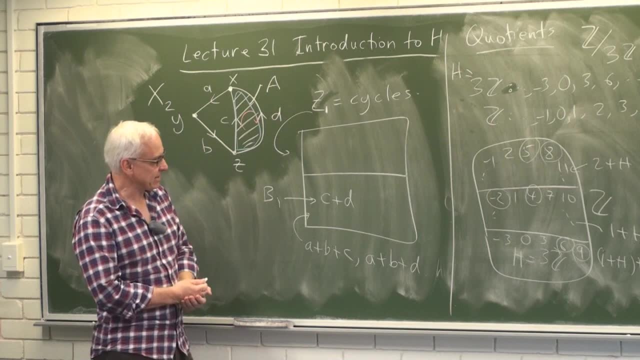 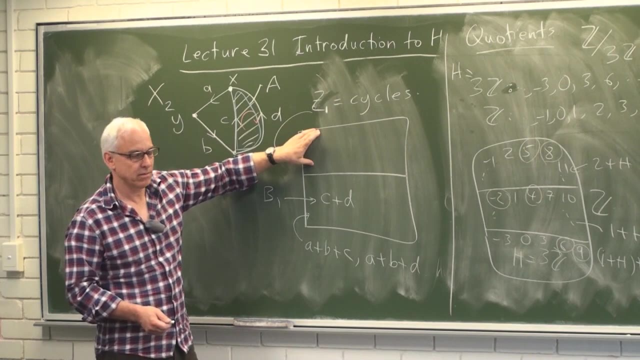 Okay, Okay. So what we're now doing is we're thinking about having a quotient. The quotient of z1 mod b1 means that we are basically looking at cosets of b1 inside z1.. Okay, Okay, Maybe the situation. 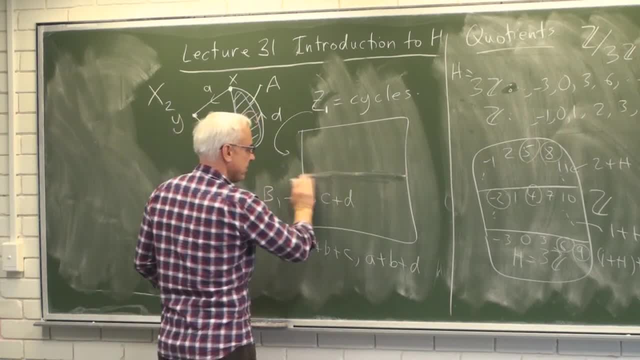 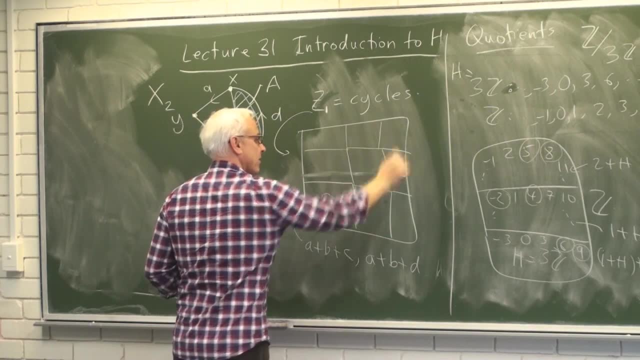 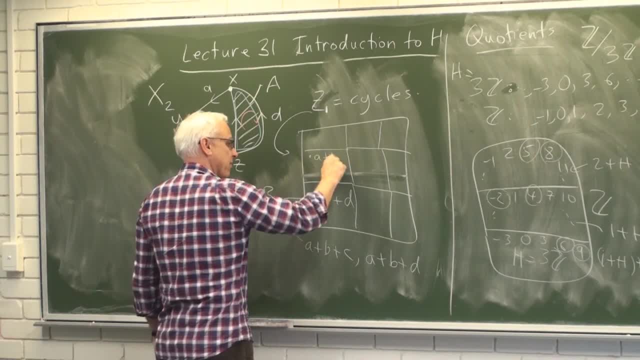 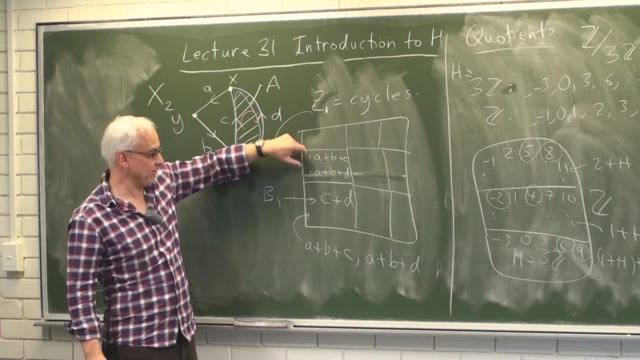 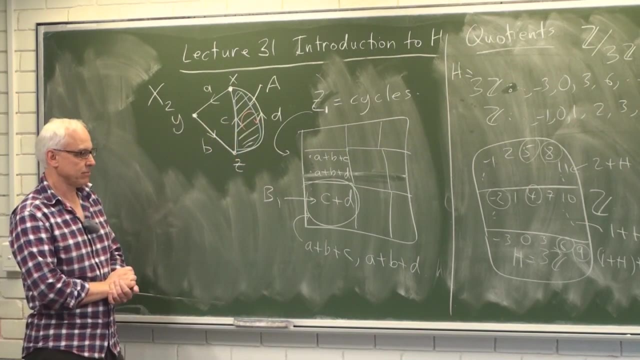 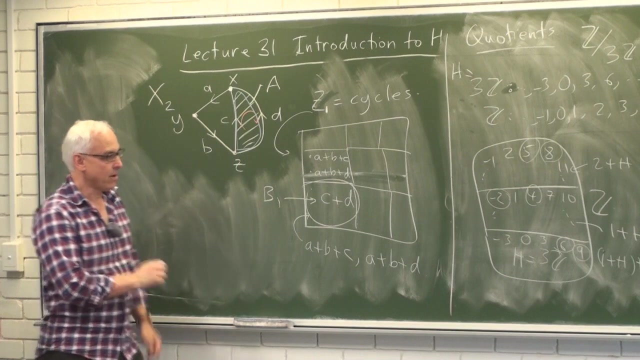 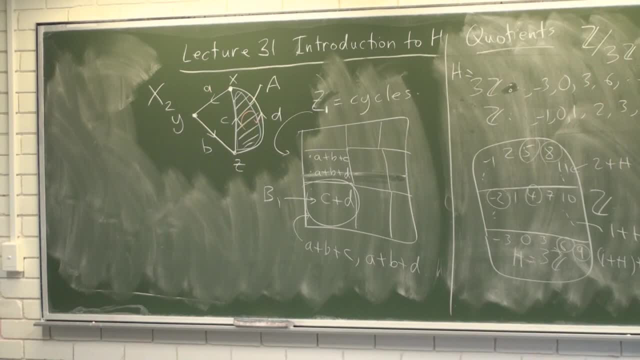 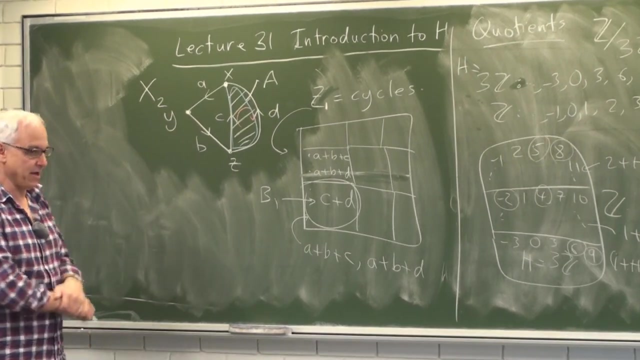 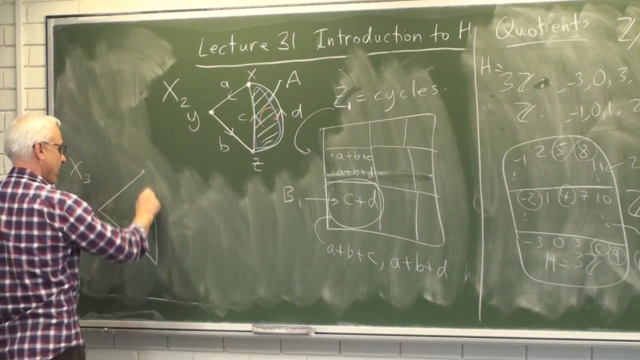 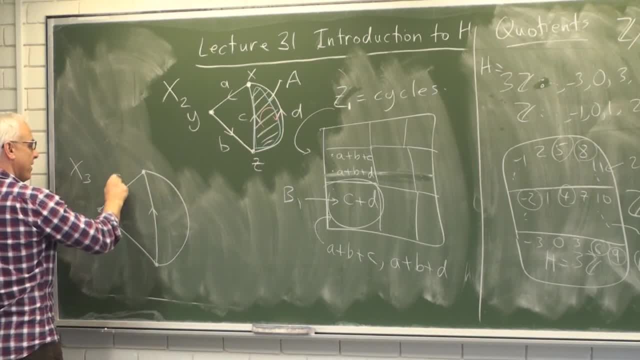 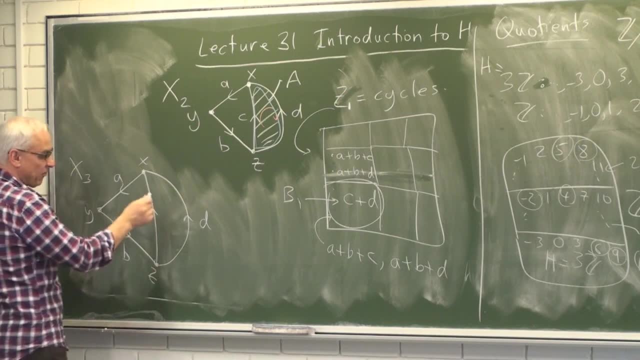 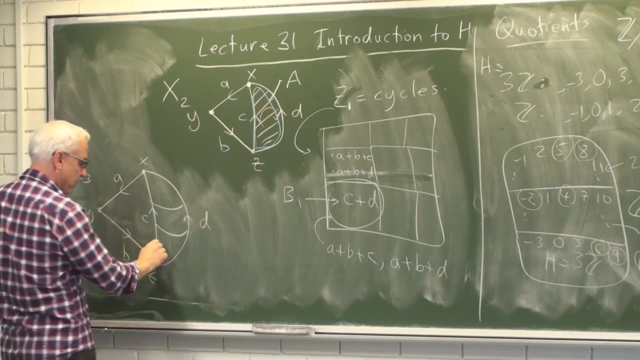 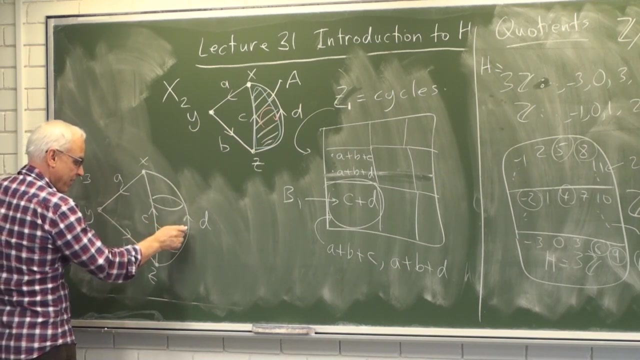 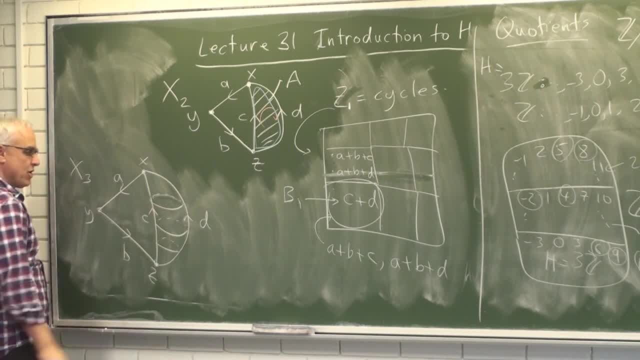 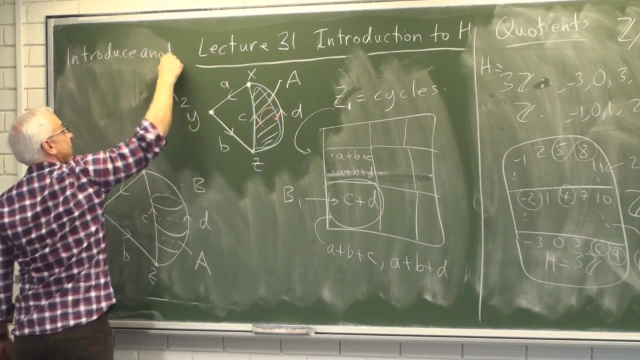 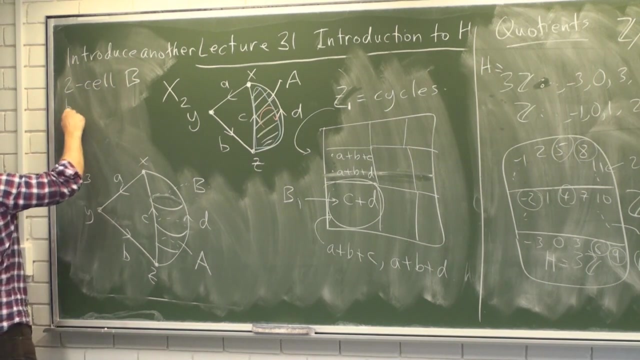 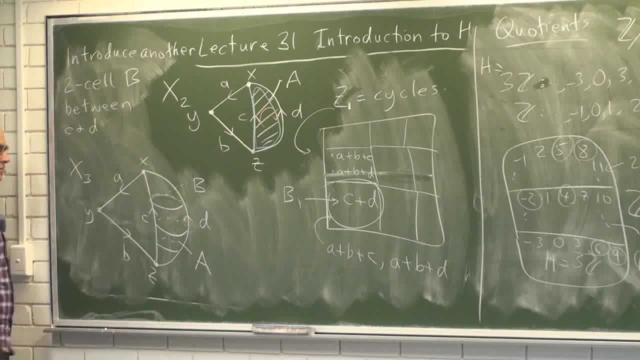 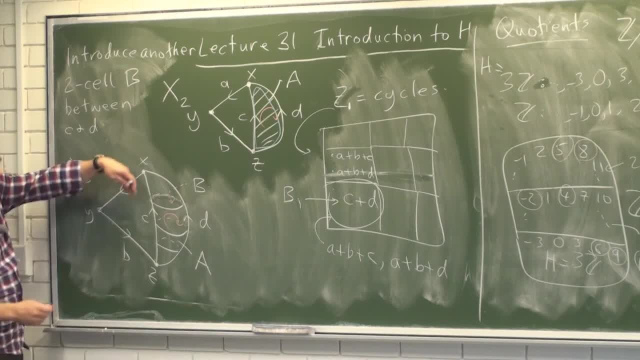 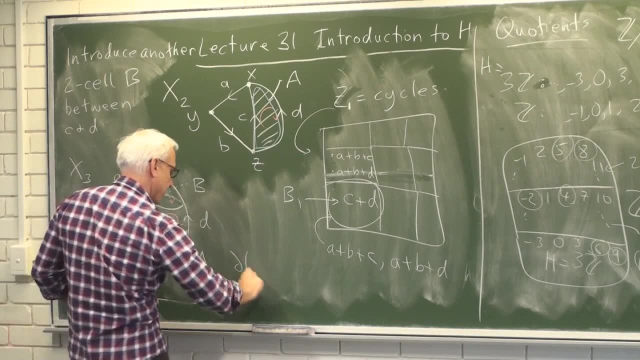 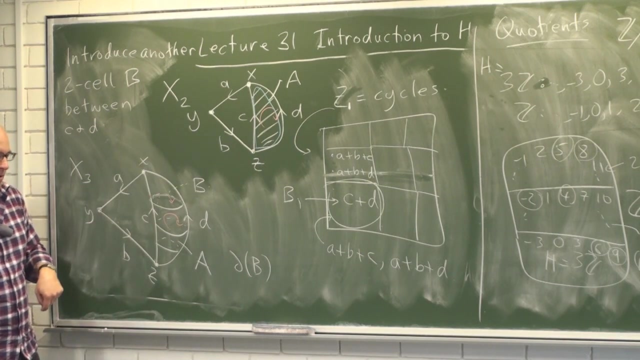 So on the back we'll have an orientation like this. So if you're looking through it, its orientation is like this. So that means that the boundary of B is the same as the boundary of A. It's C minus D. That's still the orientation of the boundary of B. 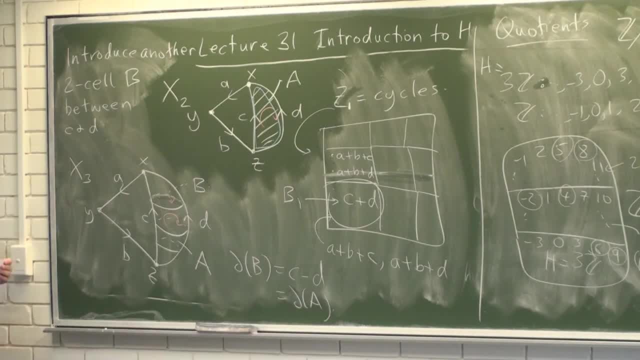 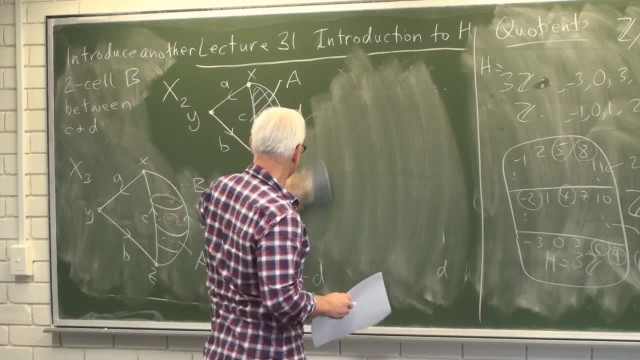 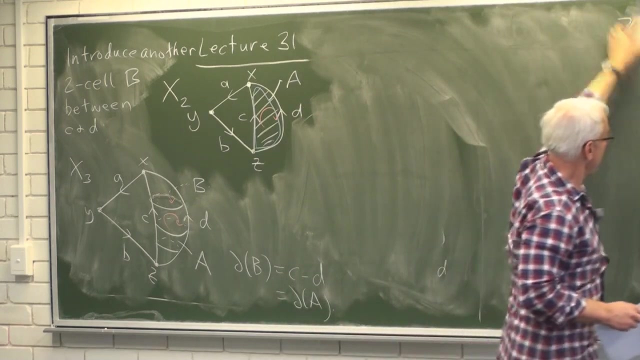 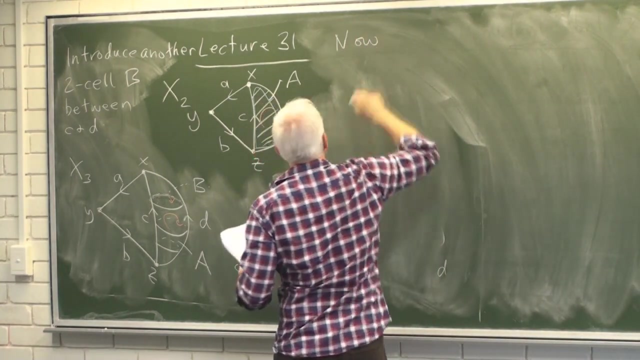 So it's C minus D. so it happens to be the same as the boundary of A. Okay, what is different now? Well, so now the main change is: C minus D is the same as the boundary of A. So C minus D is the same as the boundary of A. 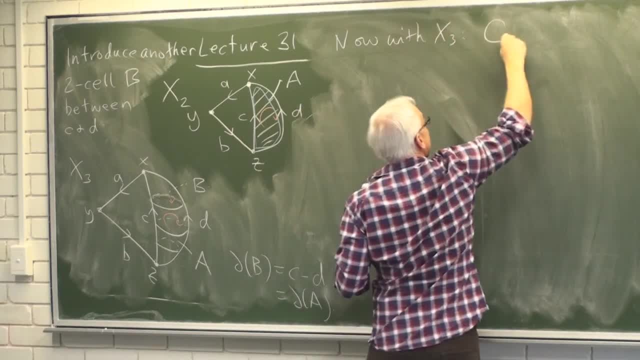 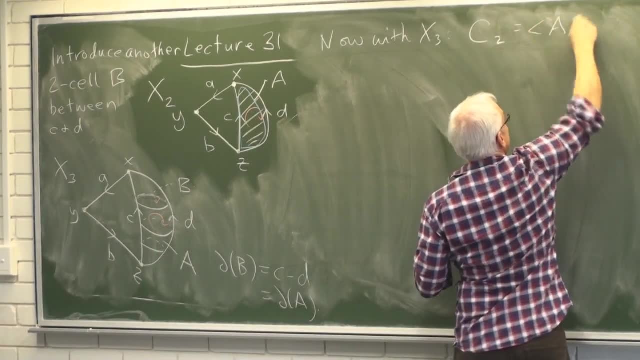 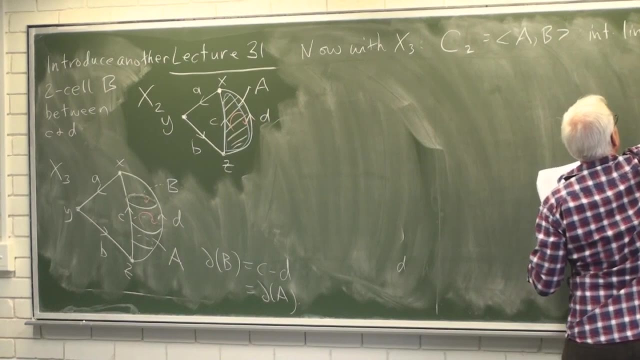 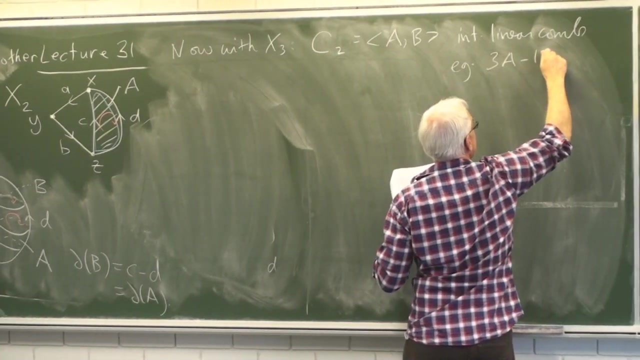 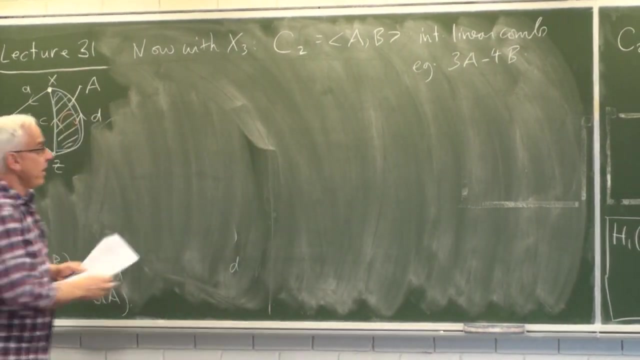 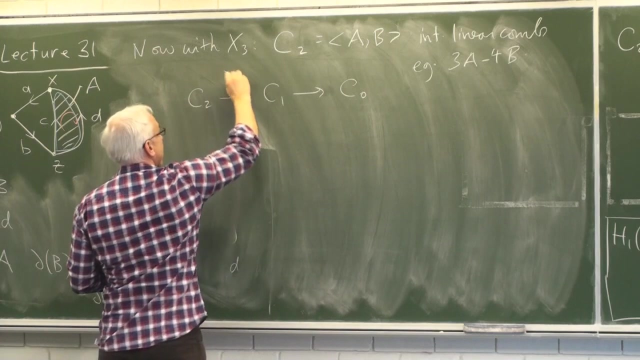 Now with X3, the space of two-dimensional chains is generated by A and B, So in other words, it's integral, linear combinations such as, for example, 3A minus 4B, And we have now our chain, C2, C1, C0, our boundary operators, D2 and D1.. 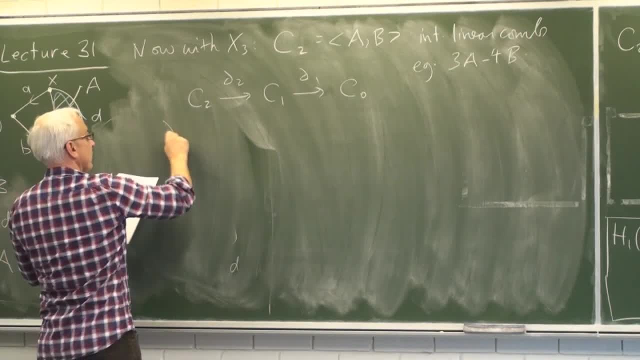 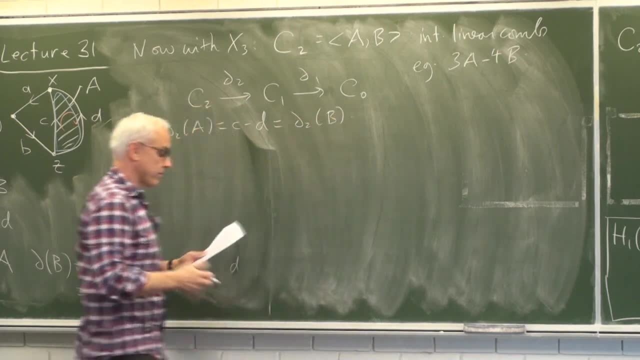 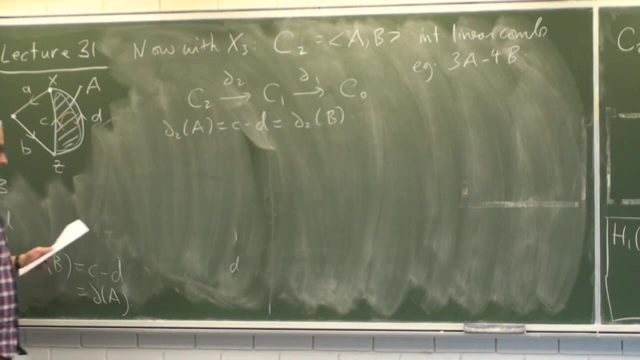 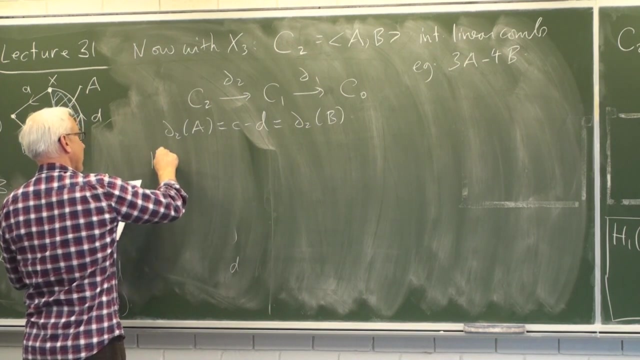 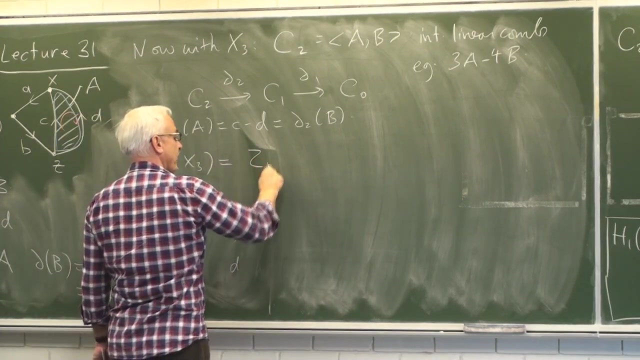 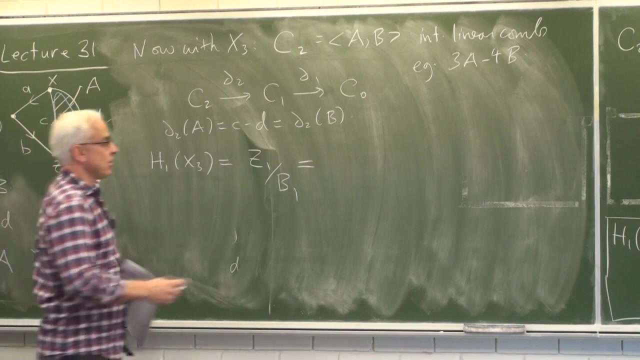 D1 is unchanged. Now the boundary D2 of A is equal to C minus D, and that's equal to D2 of B. All right, so what's happened to the first homology, homology of X3?? So, by definition, this is cycles divided by boundaries or, to be more precise, it's the kernel of the first boundary. 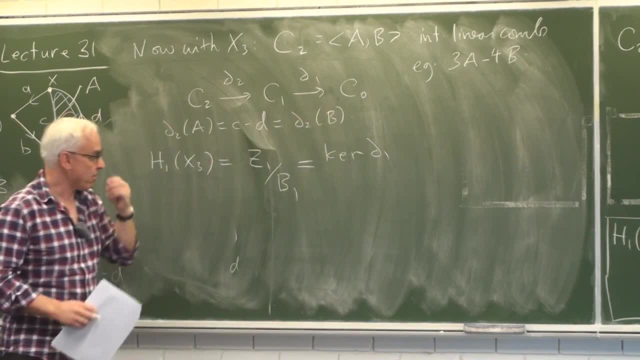 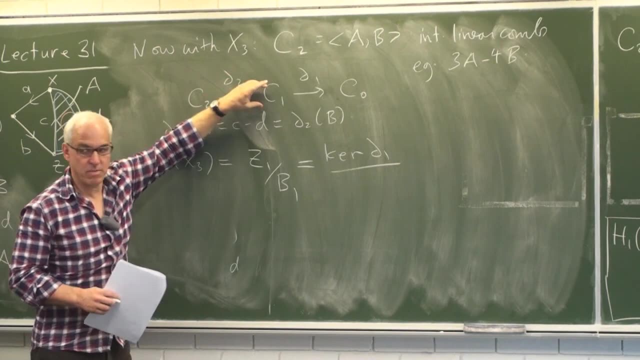 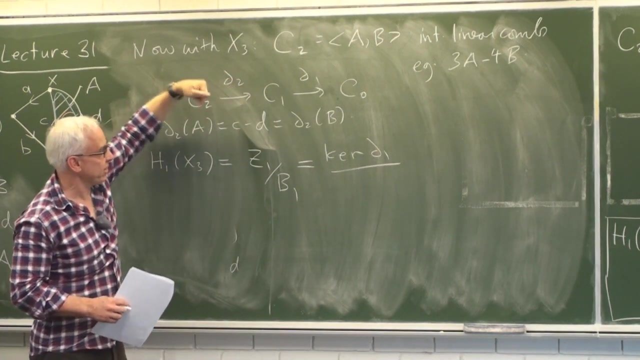 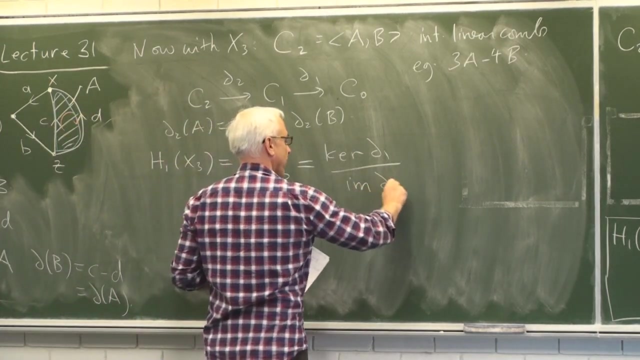 So the first boundary map, those are the cycles modded out by the image of the second boundary map, The image of the delta 2 operator is what we're calling those boundaries. they're the boundaries of two-dimensional things, So we can write image of delta 2.. 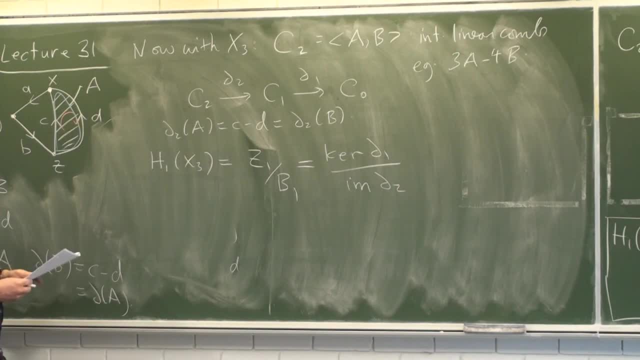 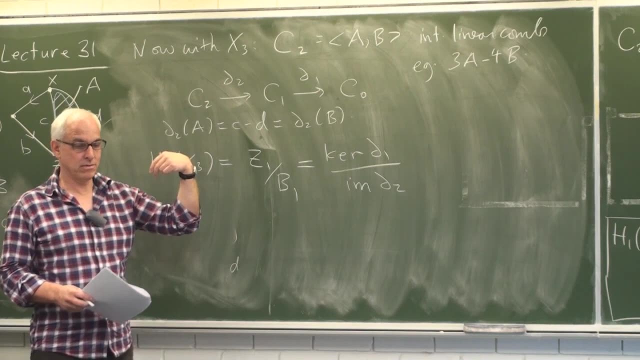 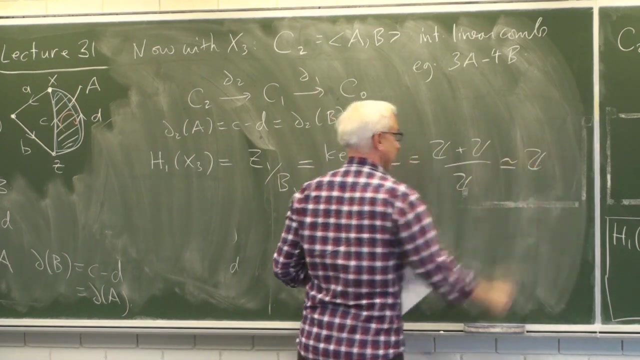 Well, that's going to be the same as before. forward, and nothing's changed. because the image of delta 2 is still just c minus d, just the way it was in the previous example. So this is still z plus z over z, isomorphic to z. 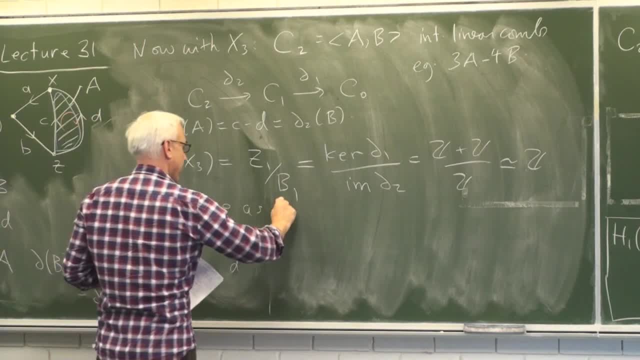 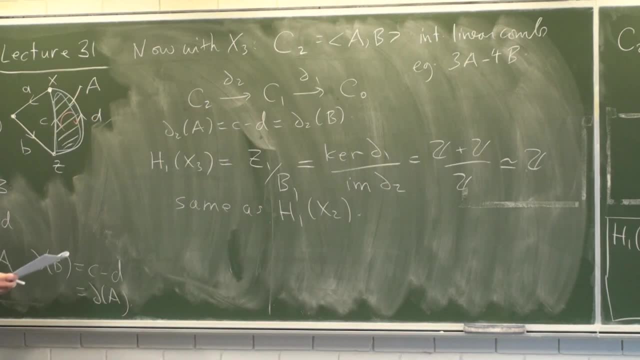 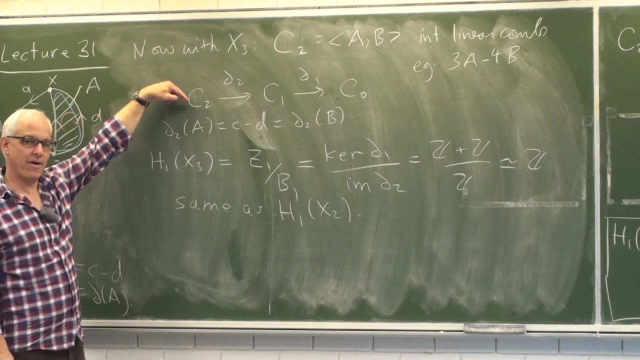 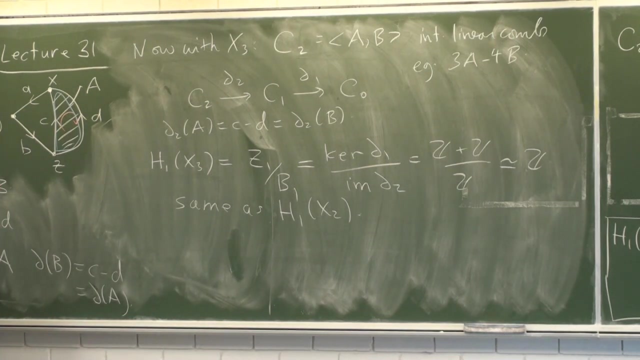 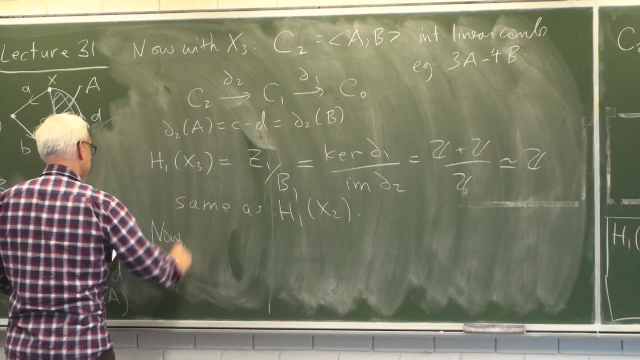 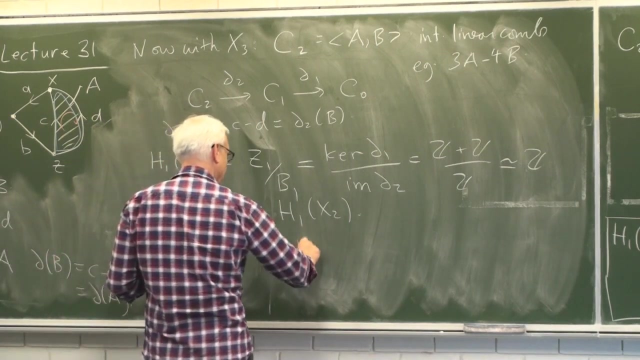 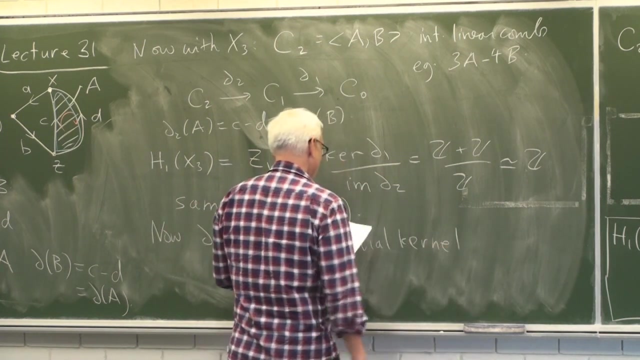 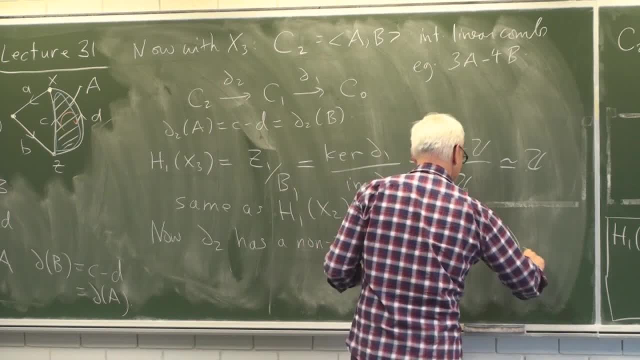 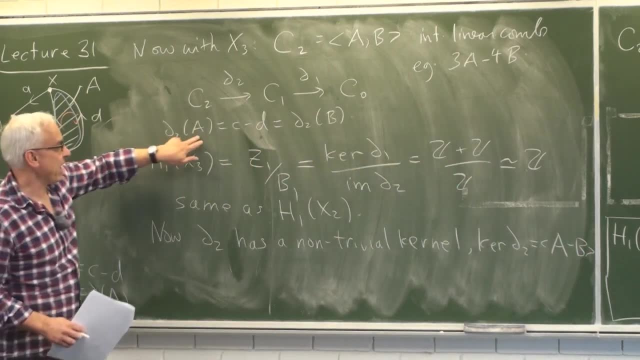 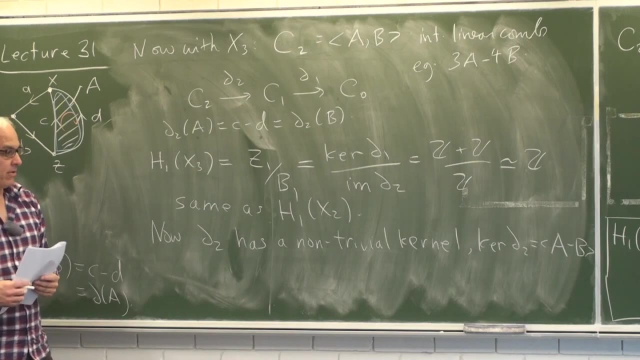 Why? because well, the kernel of delta 2 is generated by a minus b. We've seen that the boundary of a equals the boundary of b, so the difference a minus b, its boundary is going to be zero. So that means that a minus b. 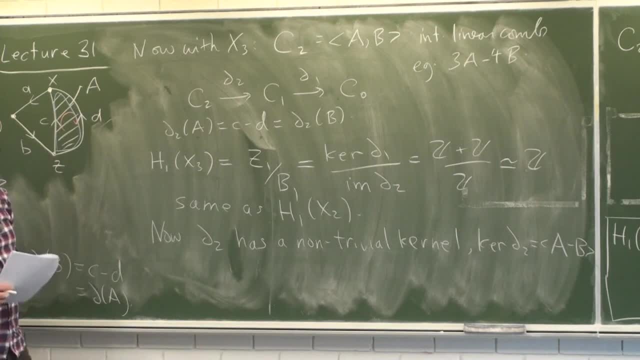 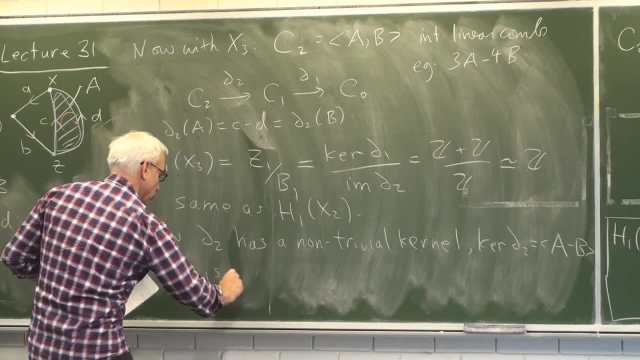 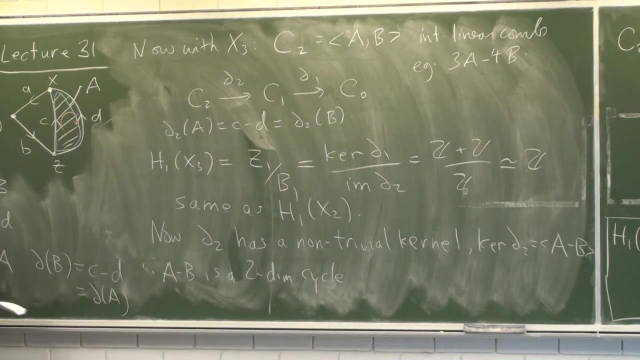 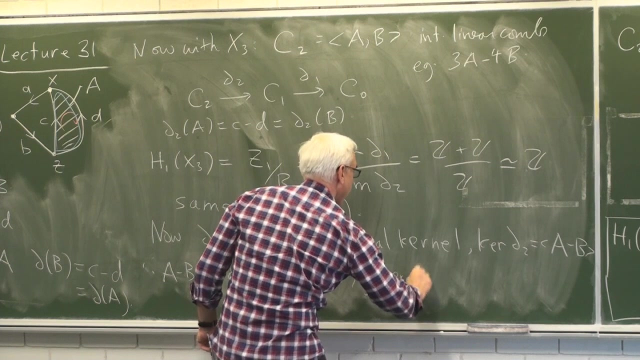 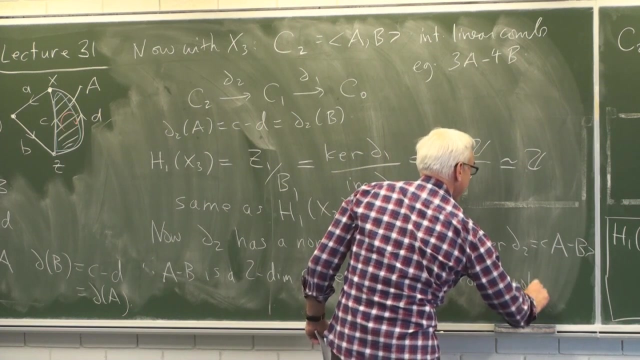 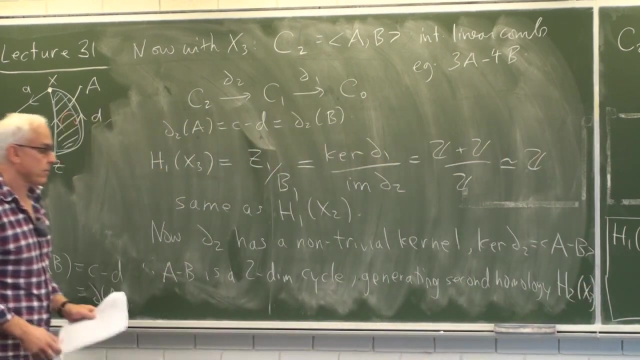 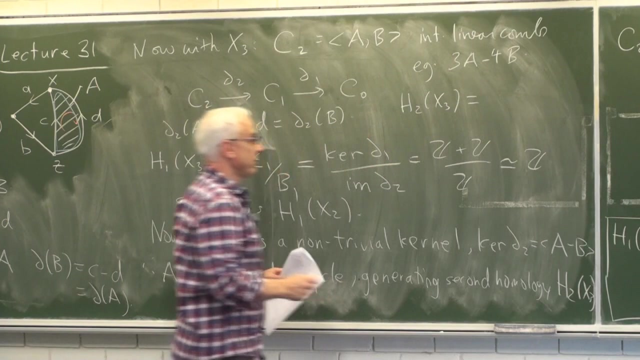 is sent to zero under this second boundary map. So we say that a minus b is a two-dimensional cycle, generating the second homology, The second homology, h2 of x3.. So I can write that h2 of x3 is now spanned by the difference. 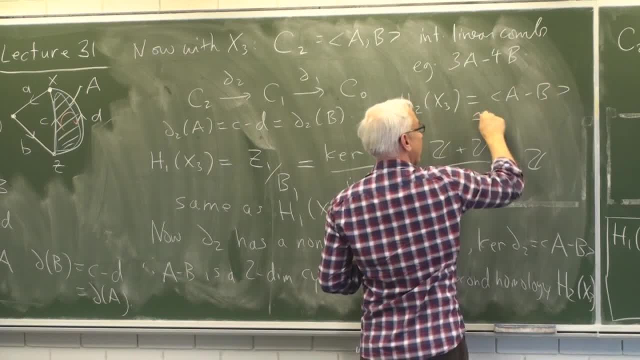 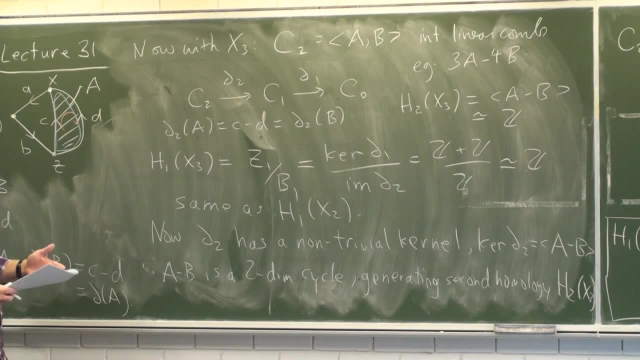 a minus b, And so it's infinite cyclic group generated by a minus b. It's isomorphic to z And this a minus b. we should think of it geometrically as a cycle that captures a hole. This x3 here has a two-dimensional hole. 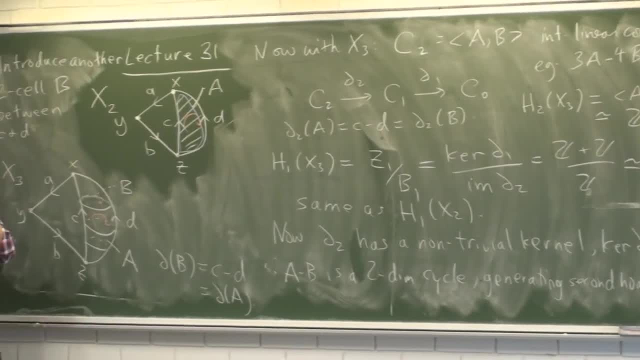 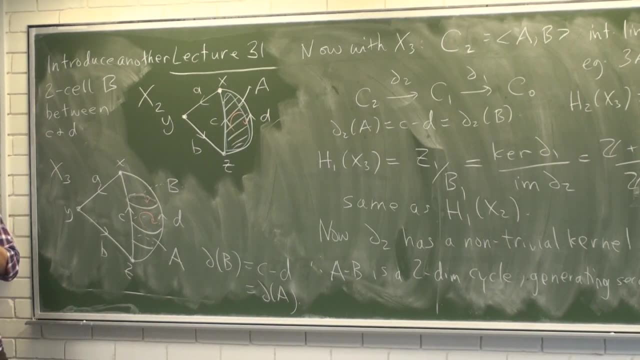 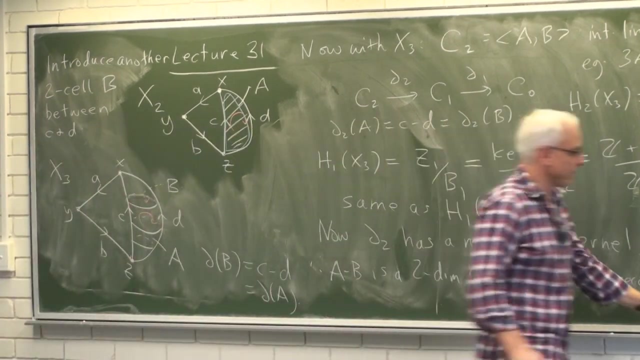 because the two pieces a and b enclose a hole And algebraically, the difference a minus b is capturing that two-dimensional hole And that's being represented by this element in the homology. Alright, so let's go one more step further and introduce: 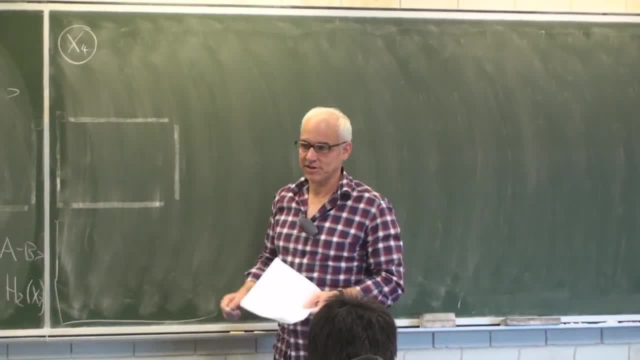 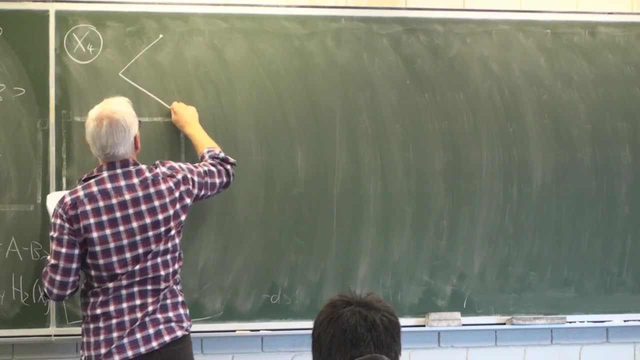 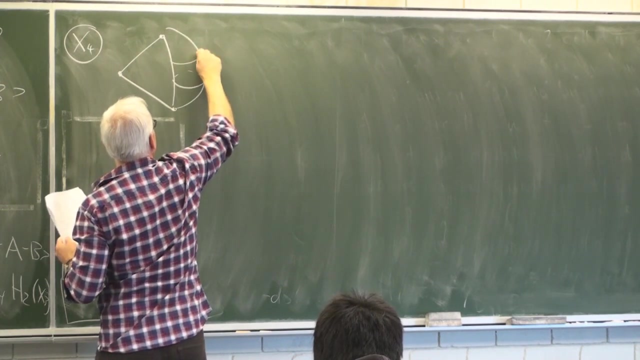 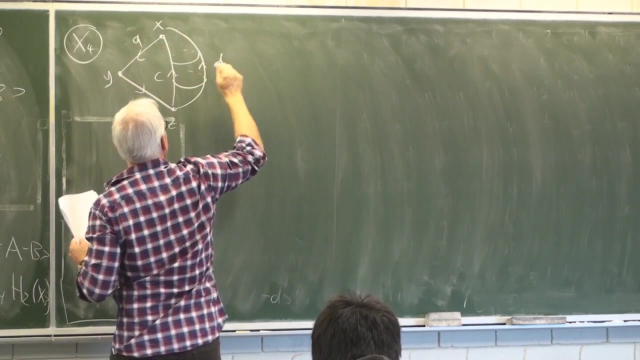 a three-dimensional aspect to this situation. So we're going to take our previous picture and we're going to augment it by adding a 3-cell now. So x, y, z, a, b, c, d, and then we had a on the front. 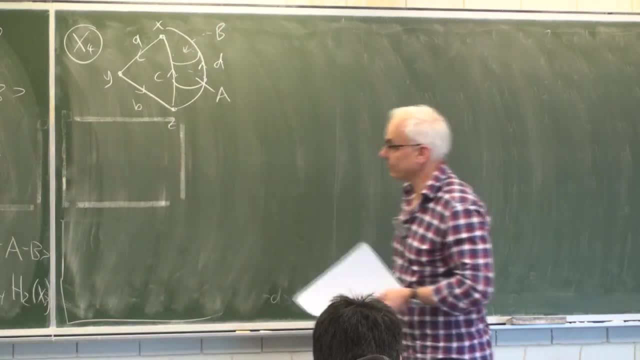 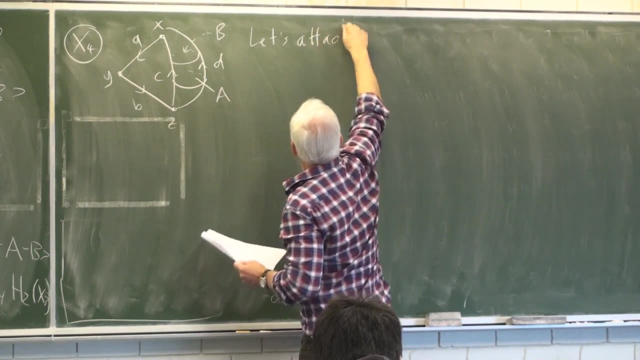 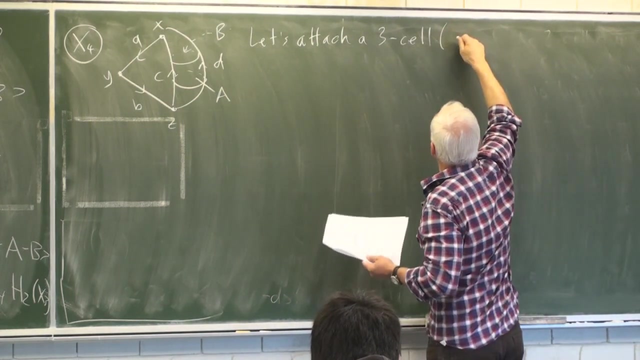 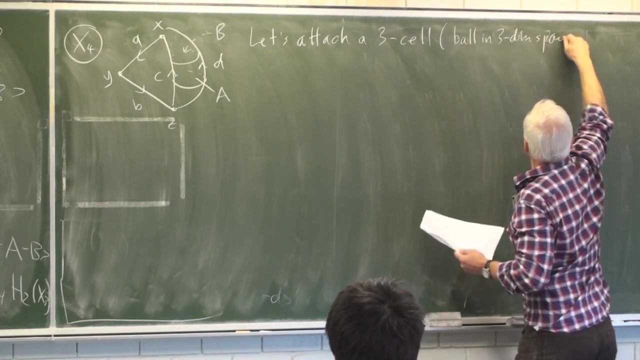 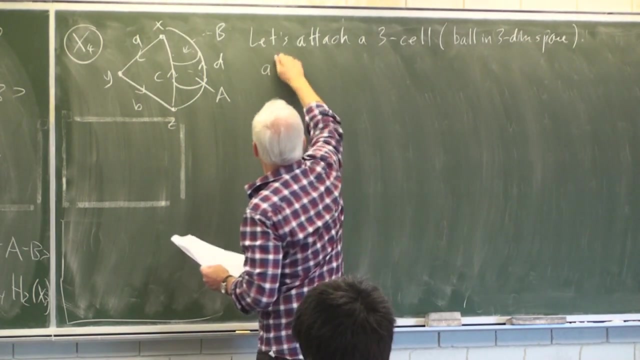 and b on the back. And so now let's attach a three-cell here, cell OK, a three cell. by that we mean a ball in three dimensional space, a solid ball. We're going to attach this solid ball along the two sphere formed. 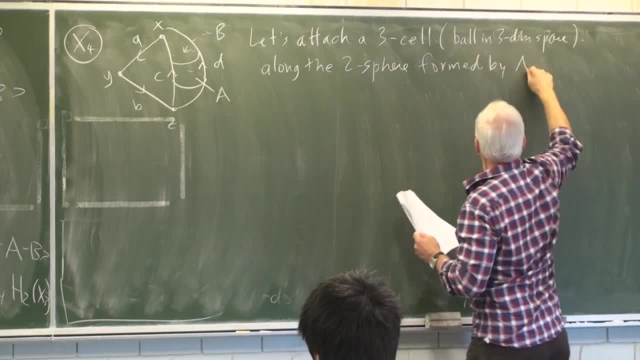 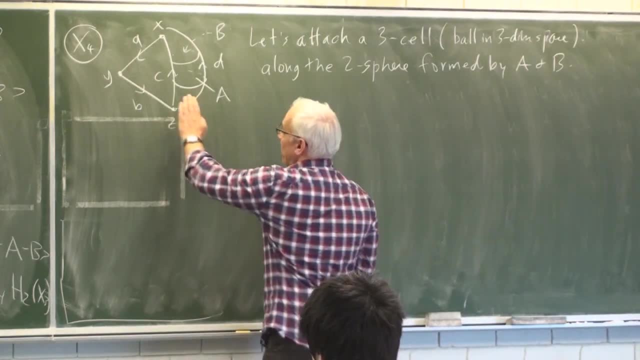 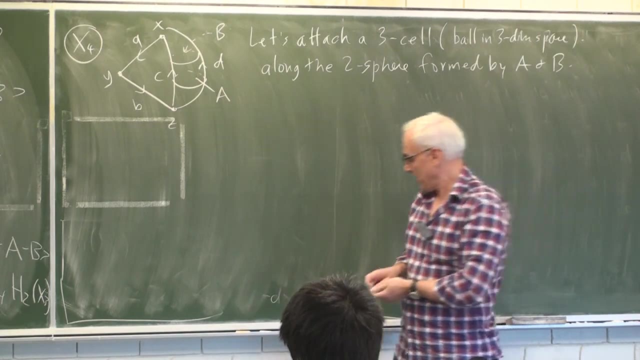 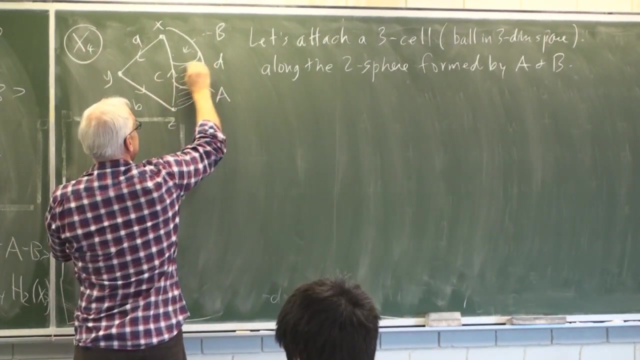 by A and B. In other words, what we're going to do is we're going to fill in the space between A and B with putty or something rather, so that it's now solid. So, inside this space formed by these surfaces A and B, we're going to fill that now with 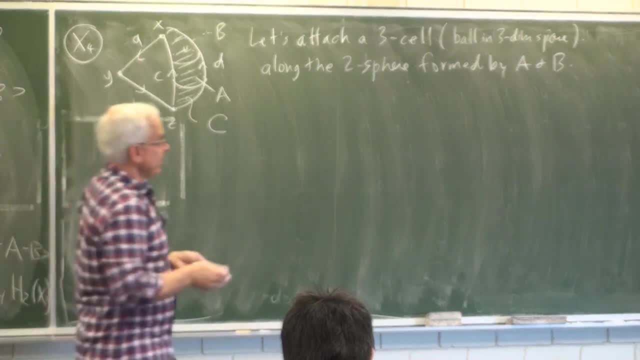 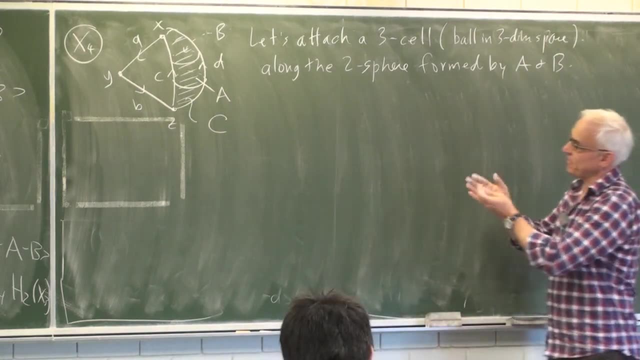 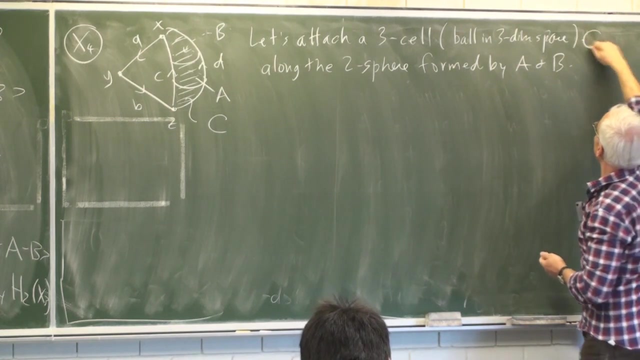 this, This three cell, this three dimensional object, solid ball that goes exactly between A and B And that's called- let's give it a name, attach a three cell. let's call it C Between capital, C between A and B. 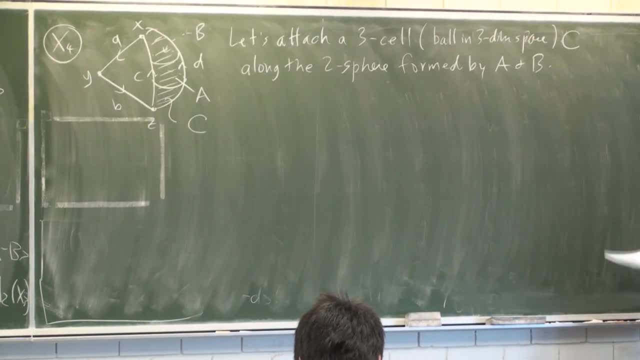 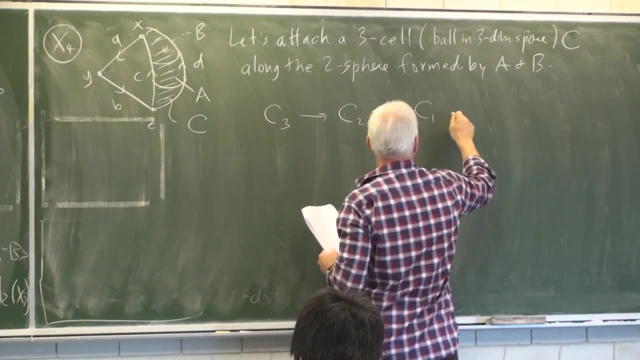 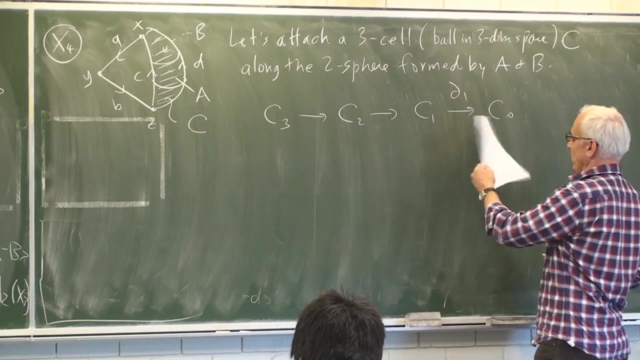 All right. so now we have some three dimensional objects, solid ball that goes exactly between A and B. So now we have some three dimensional objects as well as two dimensional, as well as one dimensional as well as zero dimensional objects. So we have our boundary D1 between C1 and C0.. 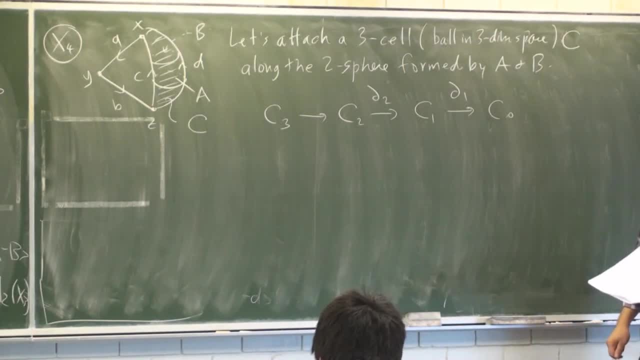 Our boundary D2 between C2 and C1, those are not changed. But now we have a new space, C3, and a new boundary operator going from C3 to C2.. So these are all spanned. Let me just say these are C0.. 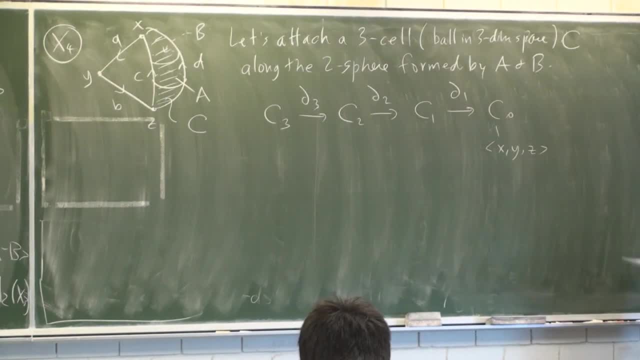 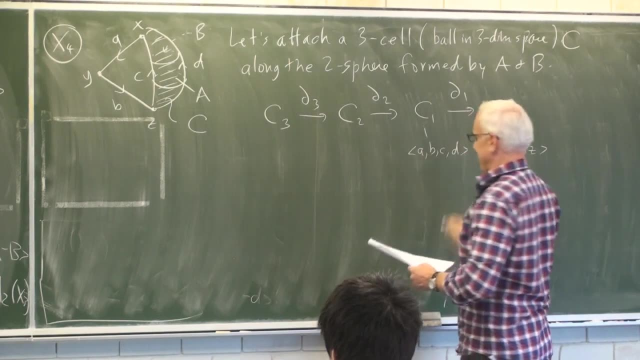 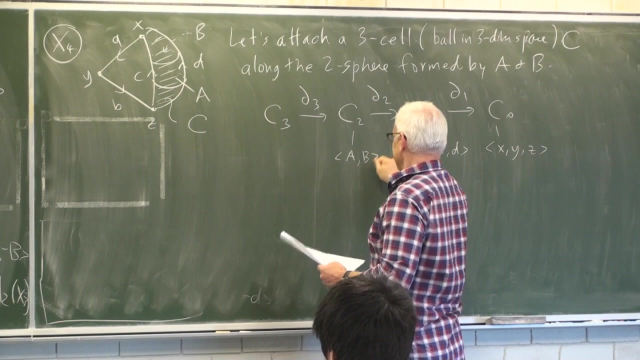 This is our zero dimensional. This is our C2.. zero-dimensional chains spanned by the vertices. C1 is the one-dimensional chain spanned by the directed edges. C2 is the two-dimensional chain spanned by the directed two cells, A and B. 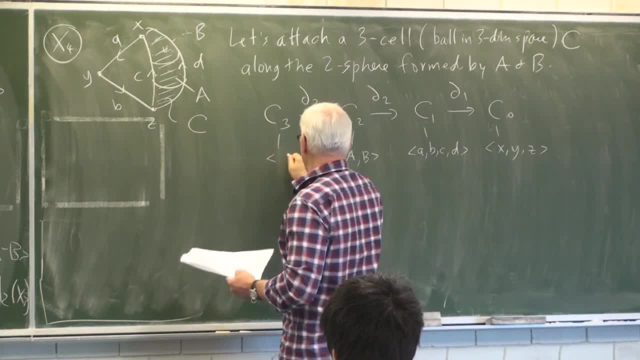 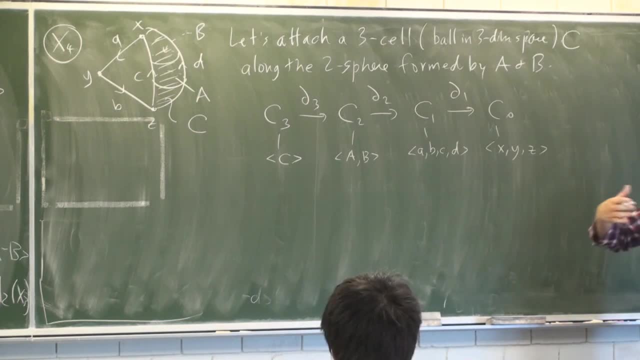 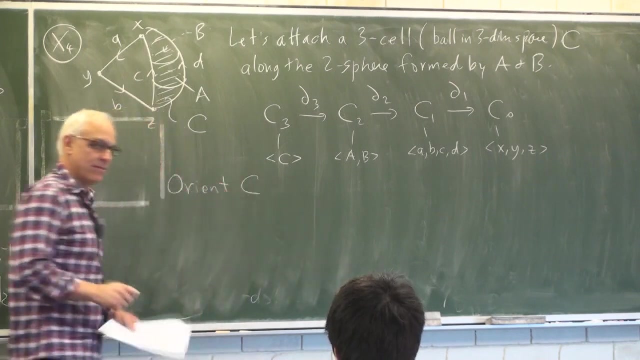 And now we have this three-dimensional chains which are spanned by this three-dimensional cell, C. Well, we still need to sort of decide on an orientation for C. We need to say what the boundary of C is. So let's orient this three-dimensional cell. 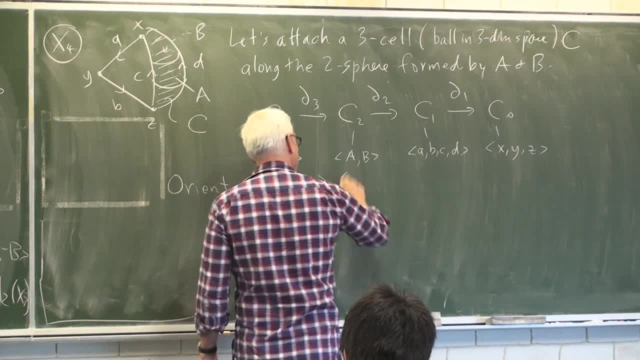 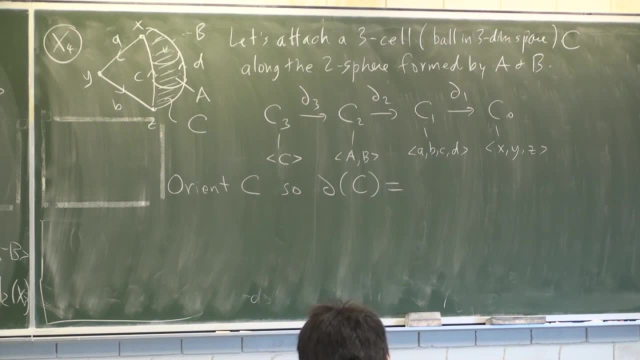 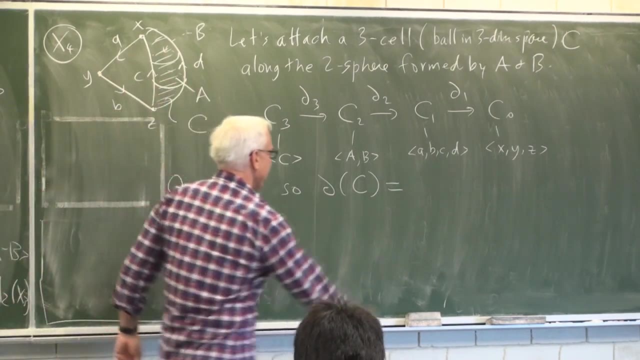 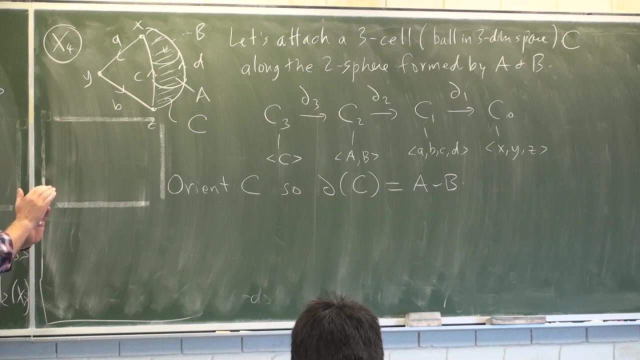 so that its boundary is Well. well, the boundary is going to be A and B, but we have to choose A minus B because, well, we want this sort of to be consistently oriented, in the same way that, when we take the boundary, say: 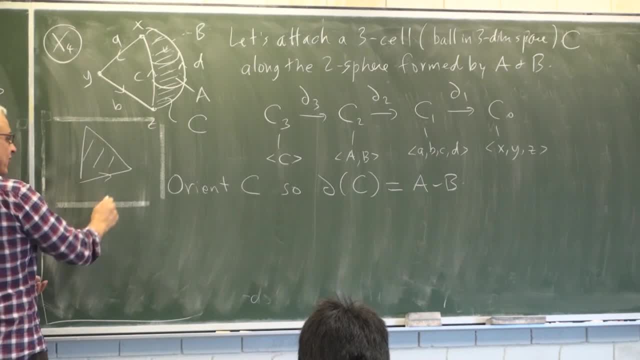 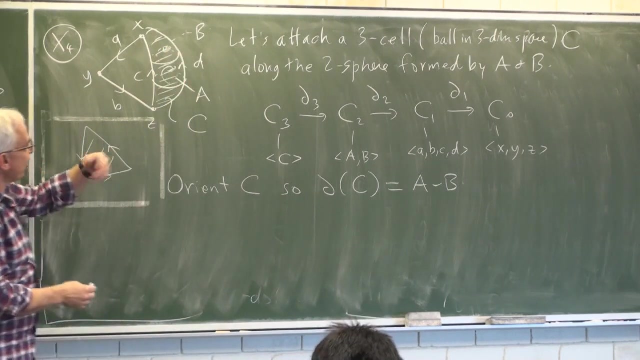 of a two-dimensional piece. we take this plus this. we make sure that these are all sort of oriented, one flowing past the other. So our orientation for A was in this direction and our orientation for B was also in this direction, And so those are not exactly in the same spirit as this. 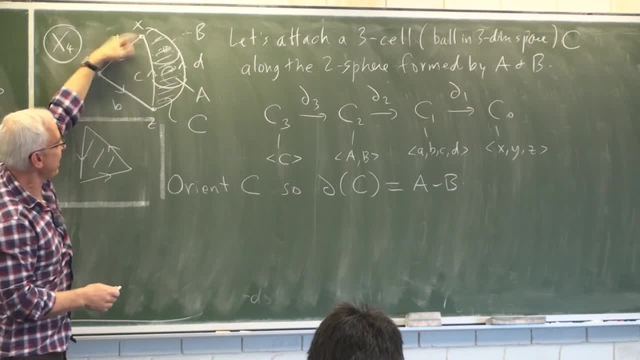 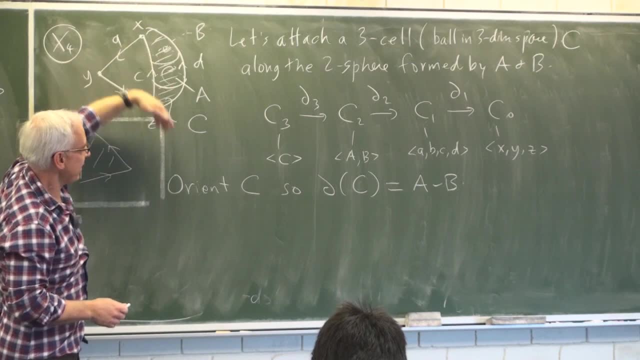 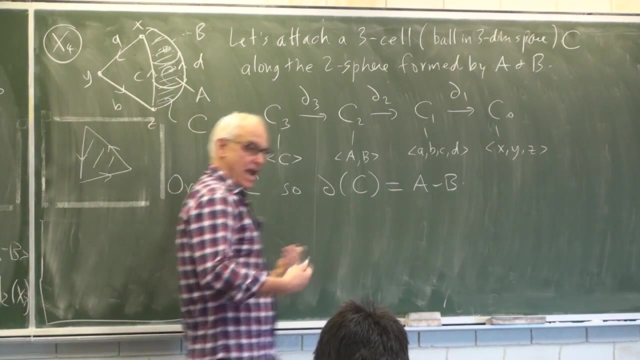 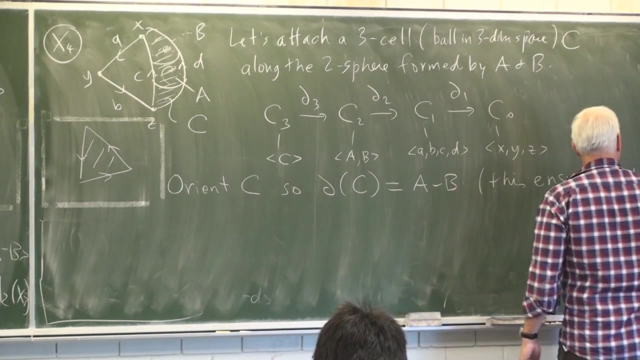 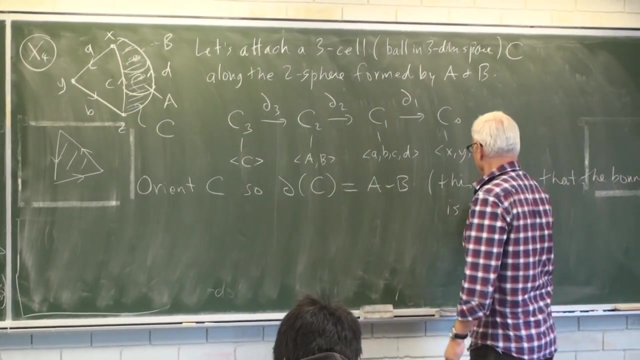 They're kind of going towards each other along this common edge, rather than opposite each other. So we're going to take the oriented A minus the oriented B as the boundary of C. So this ensures that the boundary actually is a cycle. That's one of the properties that we want. 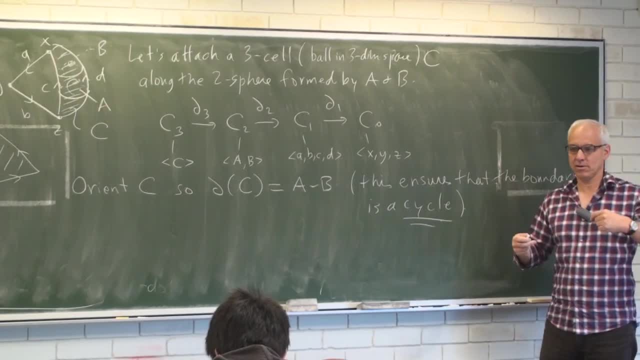 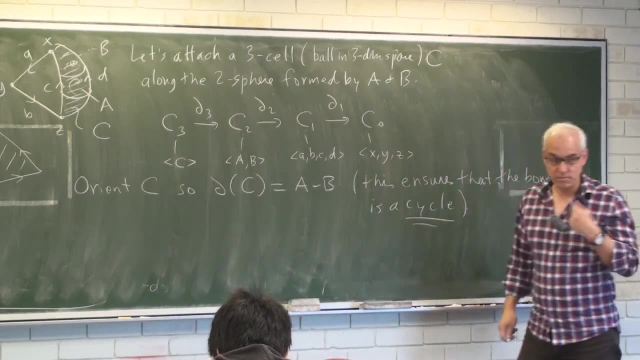 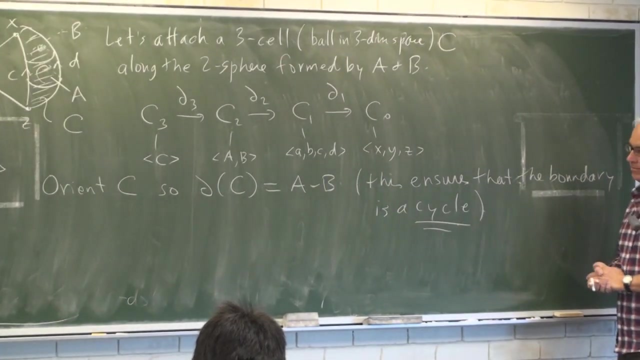 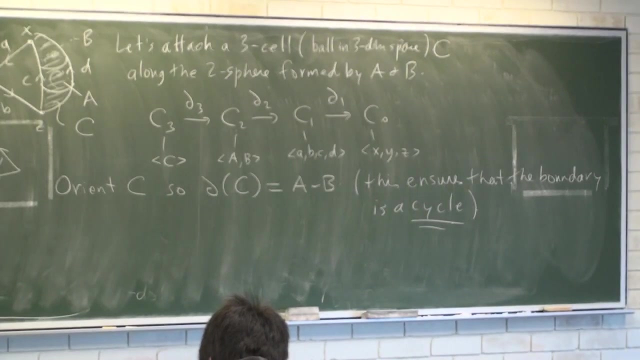 We want a boundary always to be a cycle. We decided before that, in fact, the cycles in C2 were spanned by A minus B, So this is a good choice for the boundary of C, All right. Well, how does that affect the homology groups? 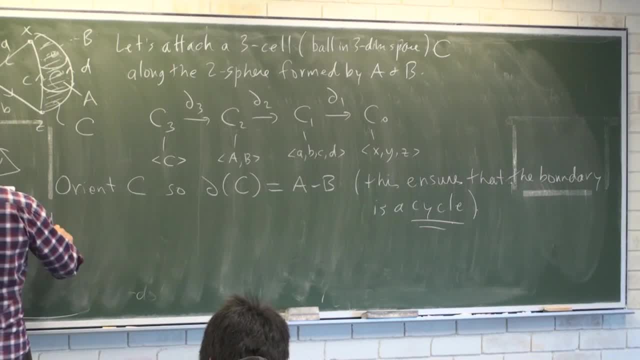 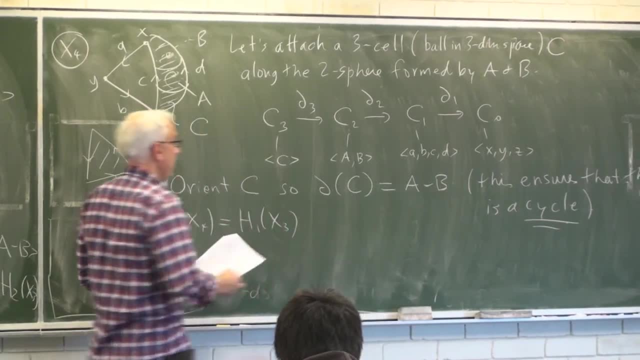 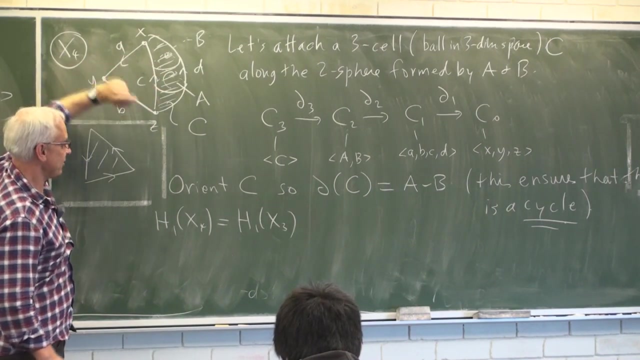 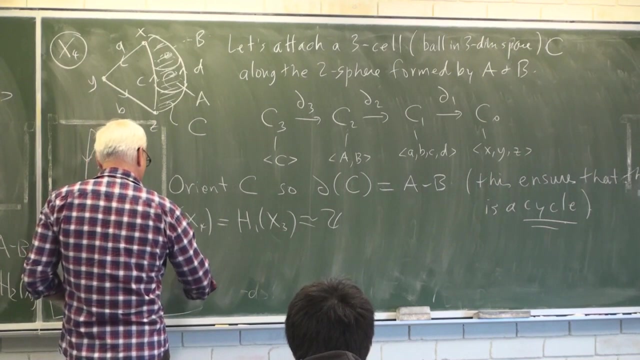 There's now first homology of X4.. Well, that's not any different from what it was for X3.. Basically, this is just one one-dimensional loop given by this cycle here, And so it's just the integers. What about H2 of X4?? 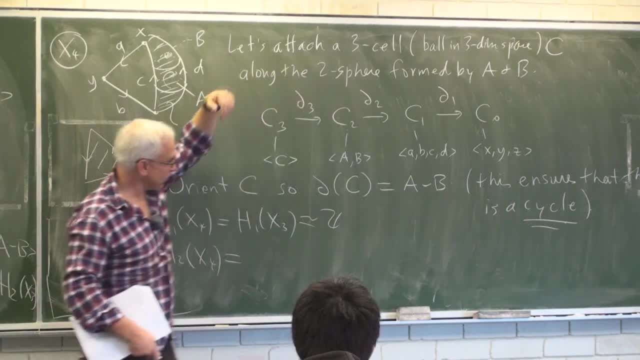 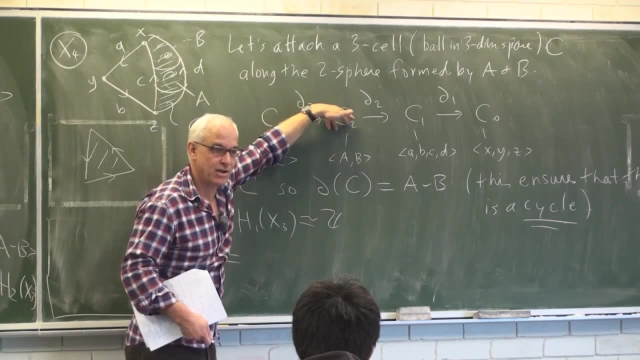 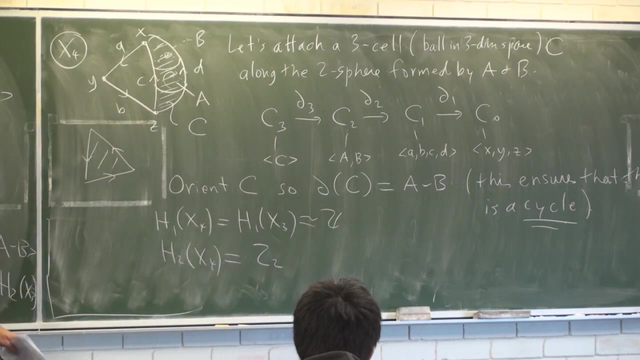 So the homology, the second homology, is going to again be a quotient. It's the quotient of the cycles here by the boundary. It's coming from here. So by definition, this is the two-dimensional cycles mod by the two-dimensional boundaries. 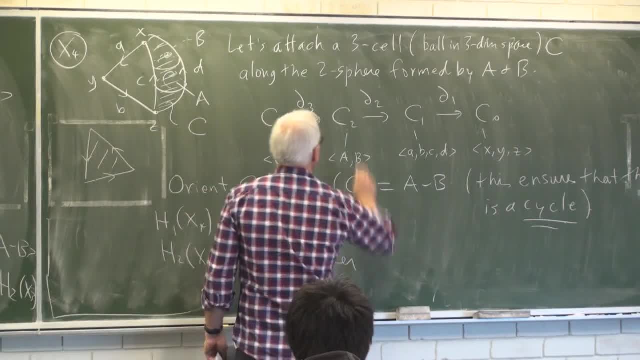 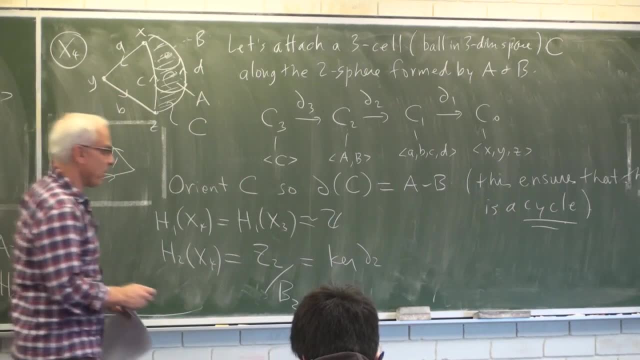 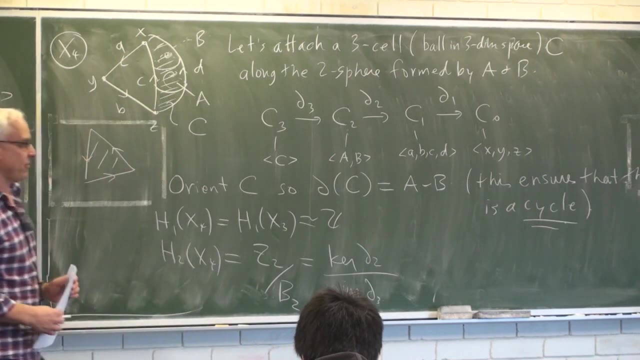 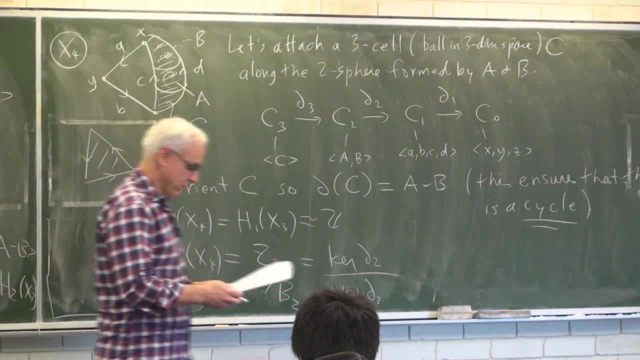 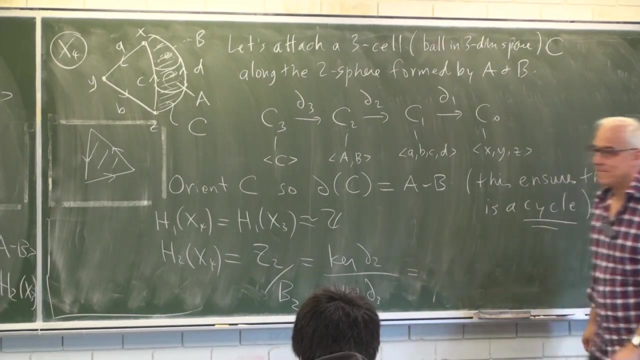 And what that means is we're taking the kernel of delta 2, that's what the cycles are- and modding out by the image of delta 3.. Those are the boundaries, All right? So what is this in this case? This is the two-dimensional cycles. 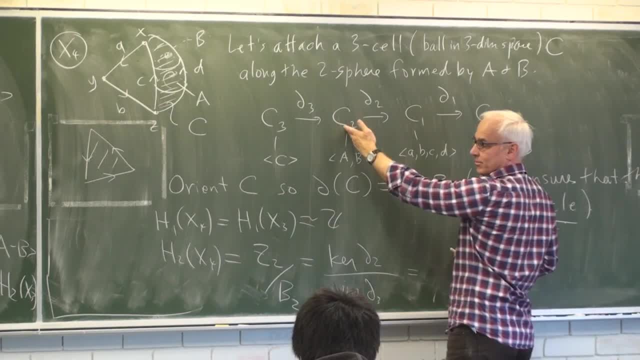 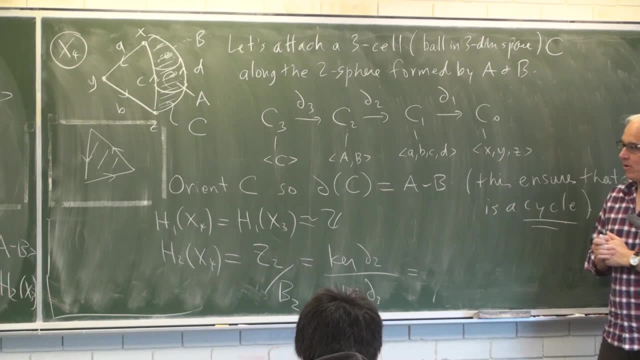 What were the two-dimensional cycles? What combinations of A and B had zero boundary? Well, this is the same as before. Those are the two-dimensional cycles. Those were all the combinations or multiples of A minus B. A minus B was a cycle. 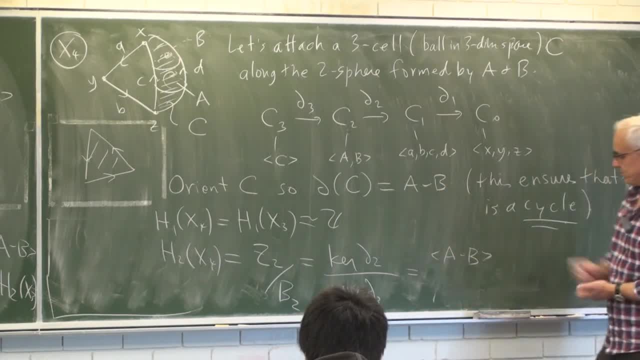 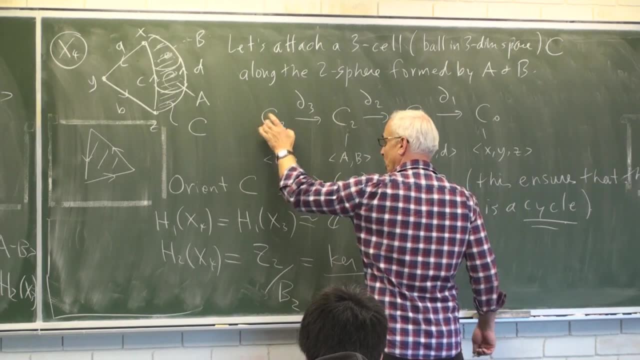 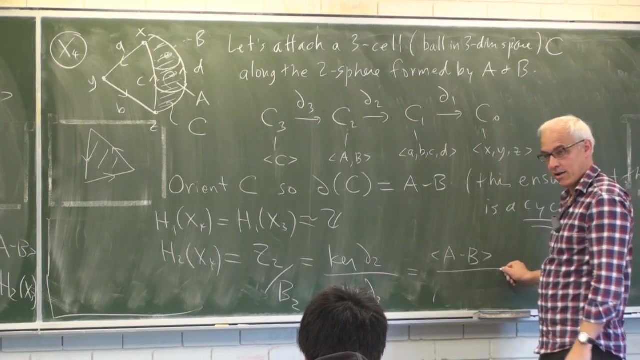 and all the cycles are just multiples of A minus B. Now what is the image of the chain C? Well, we've said that the image of the chain C is A minus B, So we have to mod out by the same group. 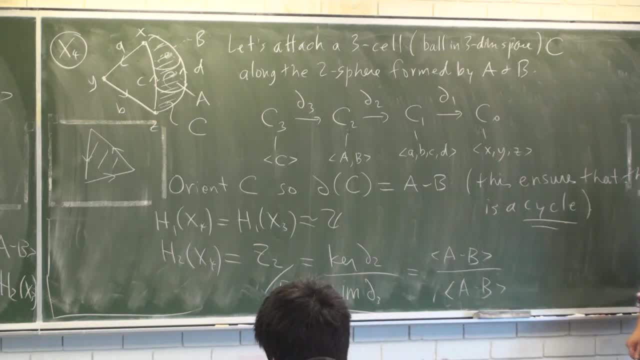 the group chain. So we have to mod out by the same group, which is generated by A minus B. When we mod out a group by itself, we're just getting the group with one element and the additive setting. that's just called the zero group. 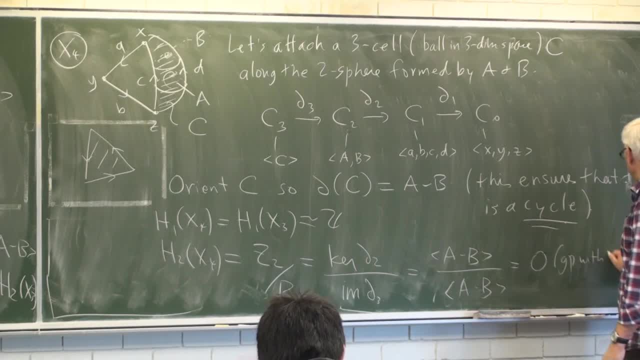 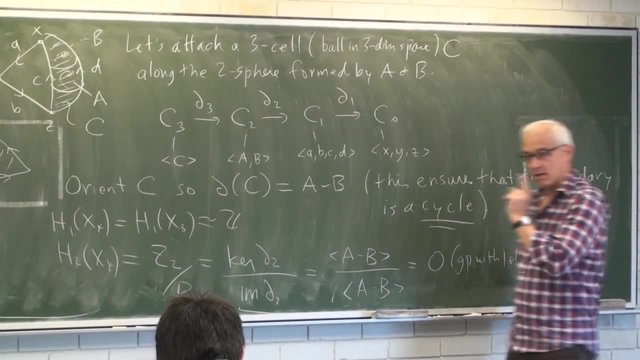 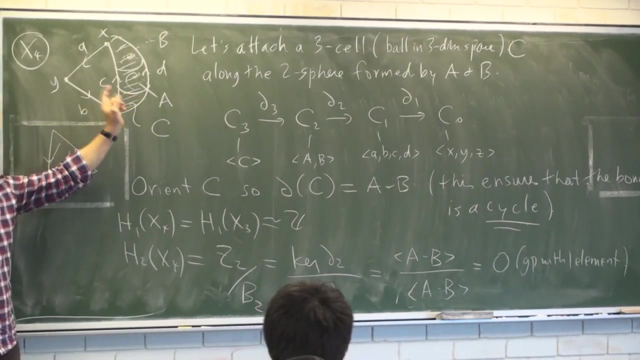 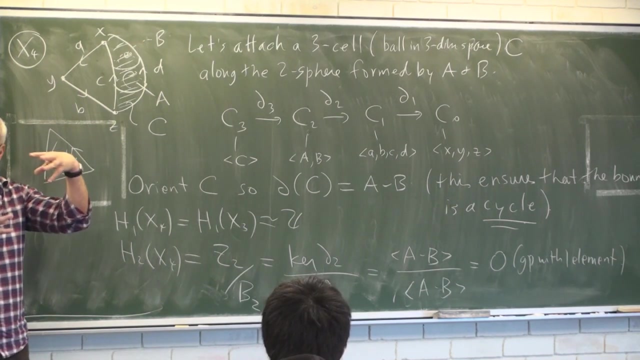 That's the group with just one element. So the second homology has changed. Before we added this cell, the homology was the integers. After we've added the cell, the homology has shrunk to zero, reflecting the fact that that two-dimensional hole. 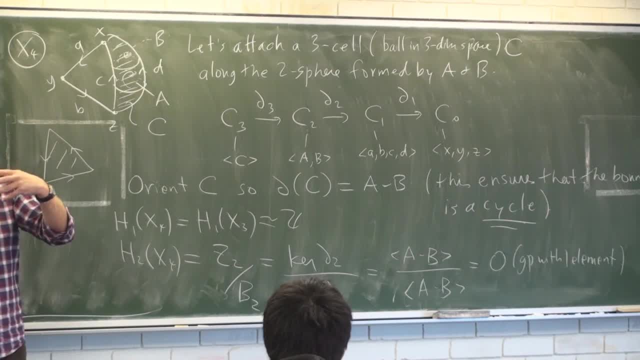 has been filled in and there's no longer a two-dimensional hole. There's still a one-dimensional hole that's captured by this homology, but there's no longer a two-dimensional hole because we filled it in, All right. so this is some kind of introduction. 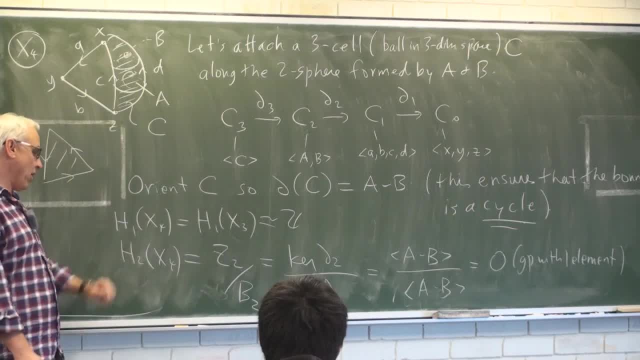 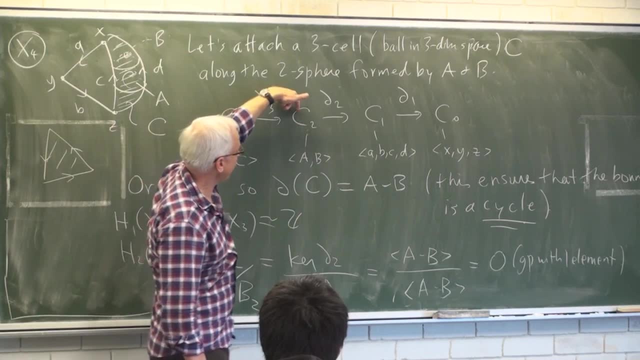 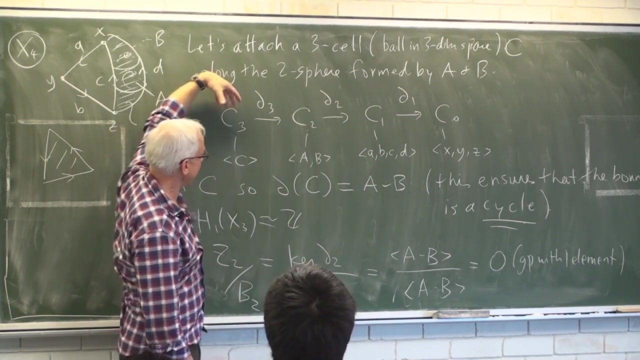 to the ideas, the basic formula of that. we're computing homology by taking a quotient of cycles to boundaries, where cycles at any stage are the ones that get sent to zero by the boundary, and that the boundaries are the images of the one-dimensional higher chains. 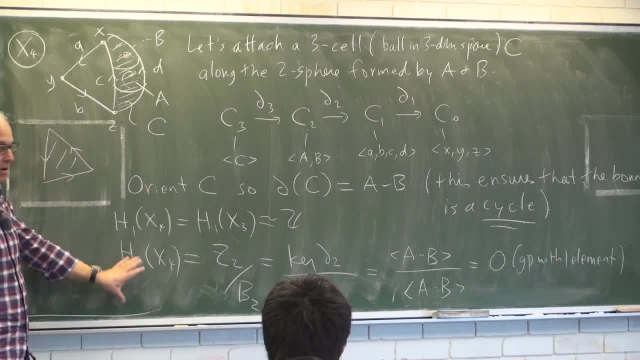 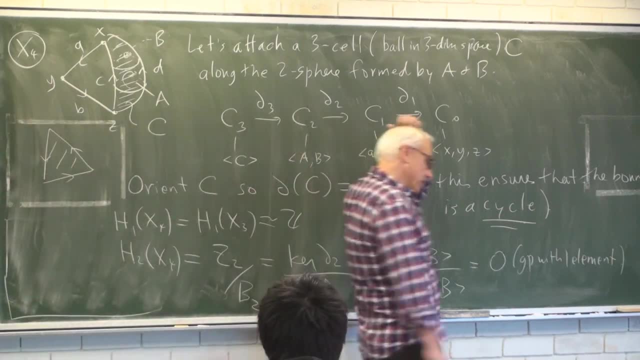 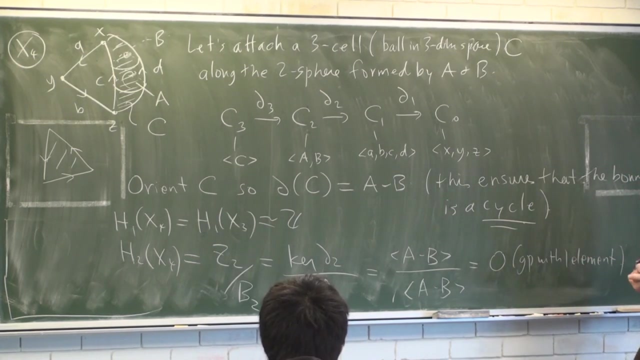 under their boundary map. That's the basic formula for homology. Okay, so what we want to do is we want to make a framework in which we can set this up, this theory up, not just by drawing pictures, but sort of more formally. 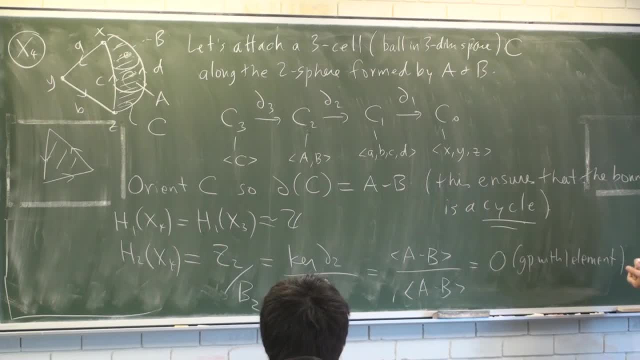 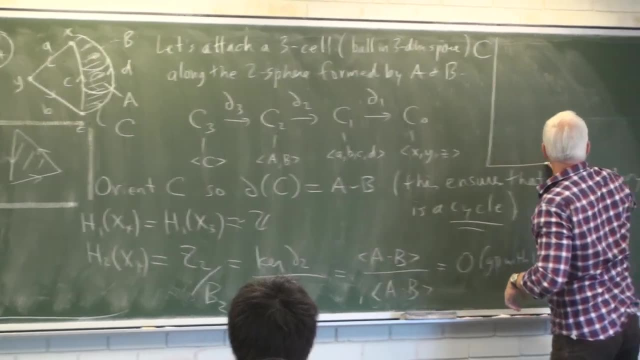 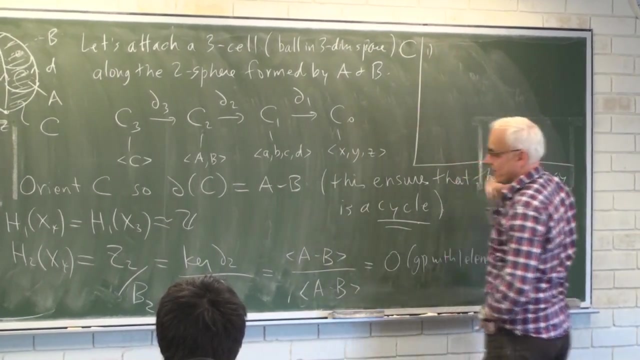 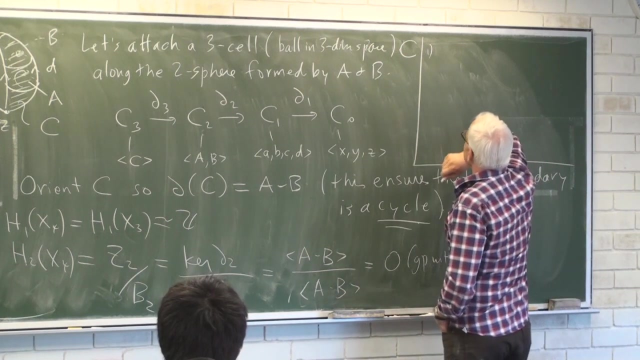 And there's a couple of variants of doing that and none of them are entirely easy. So there's basically two approaches to setting up a theory of homology. One is sort of the initial one that Poincaré introduced late in the 19th century, around 1895.. 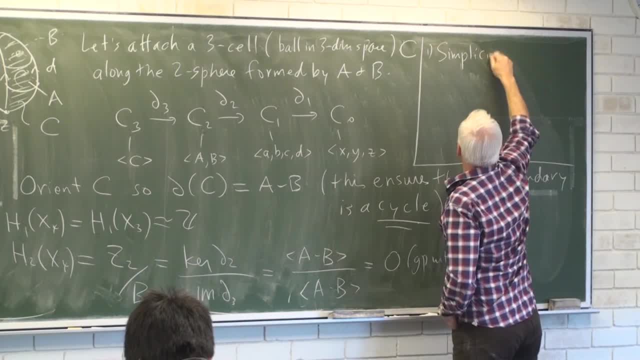 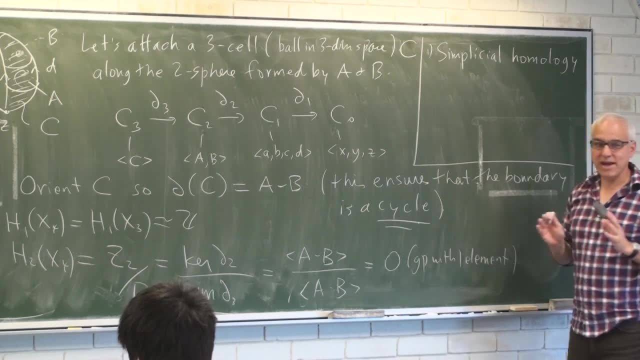 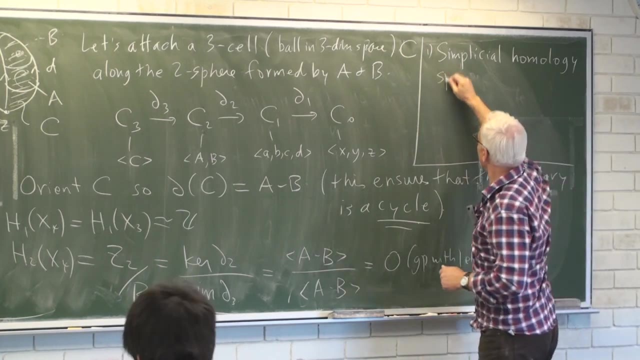 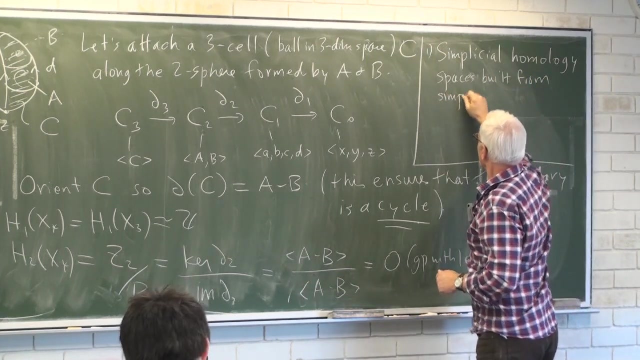 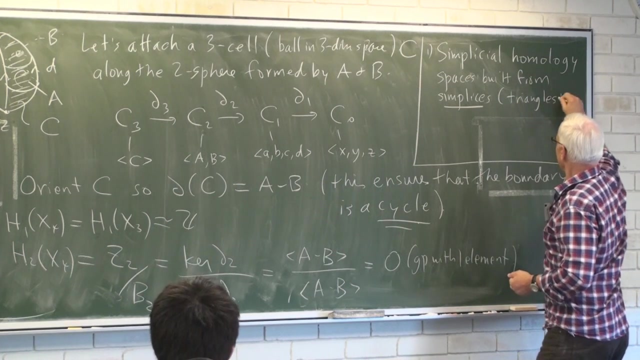 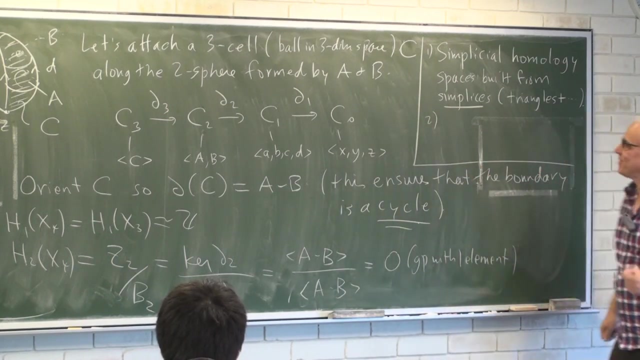 It's basically what we might call simplicial homology, where we deal with spaces of a relatively prescriptive, described kind. So a space is built from simplicies- Simplicies are basically triangles in higher dimensions- And then there's a more flexible kind of homology. 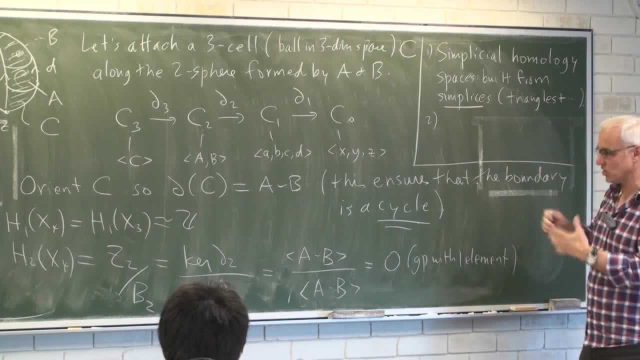 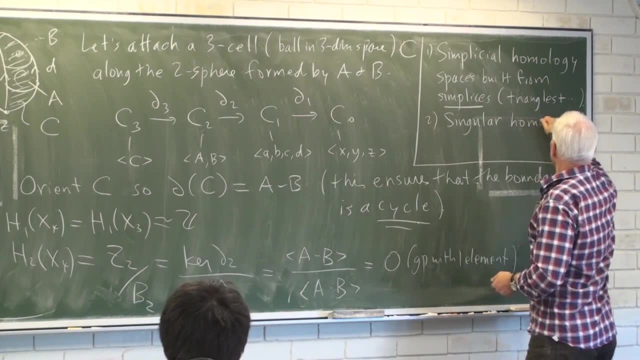 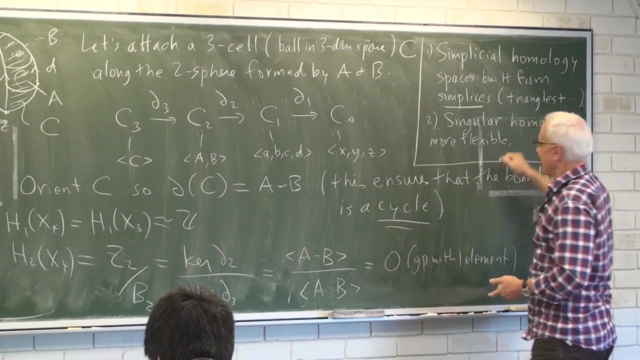 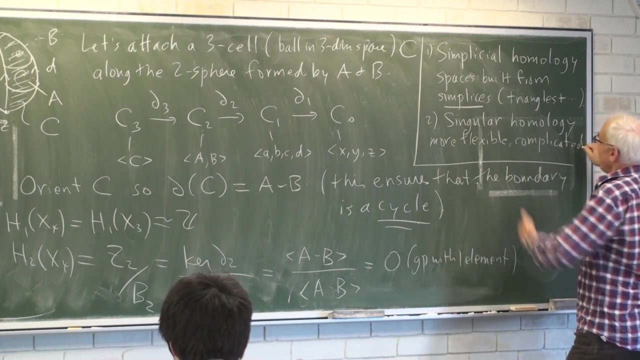 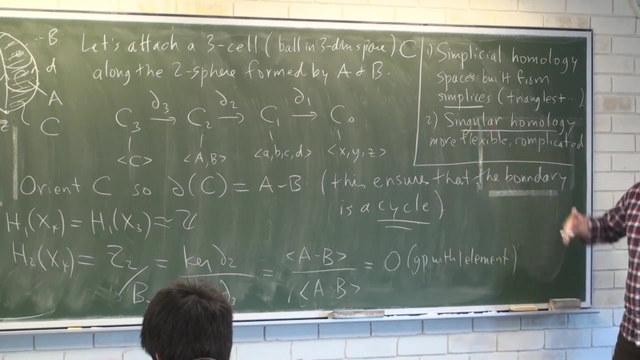 that doesn't orient itself towards such rigid spaces, called a singular homology- Maybe not such a good name, but anyway. So it's more flexible, also more complicated and less combinatorial than the simplicial homology, But for most spaces. 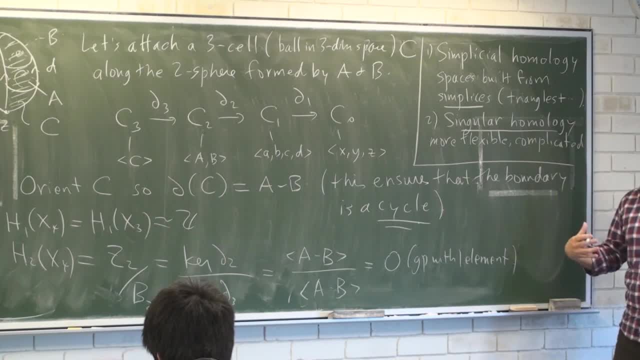 the two theories end up giving the same homology. But for most spaces, the two theories end up giving the same homology. But for most spaces, the two theories end up giving the same homology groups. You end up getting the same actual groups. 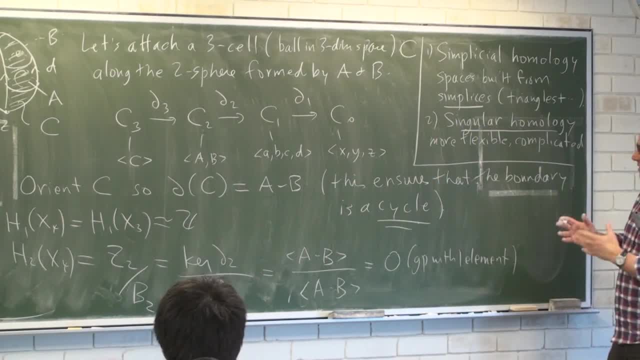 in either theory, but there's sort of a different orientation. So, since this is a beginner's course, we're going to concentrate on the simplicial homology. That's really a more simple version, which is still powerful enough that it allows us to compute a homology. 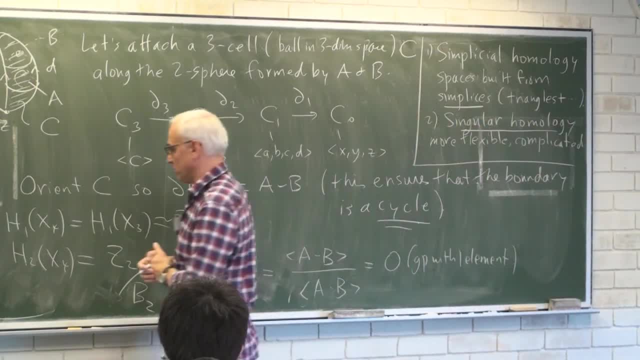 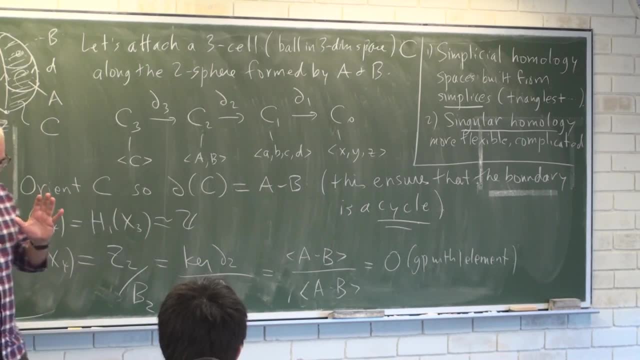 for lots of spaces that we might be interested in and that we might want to construct, and that we might want to construct Okay. so this has been sort of an introduction, a bit of hand-waving. We want to now be a little bit more precise. 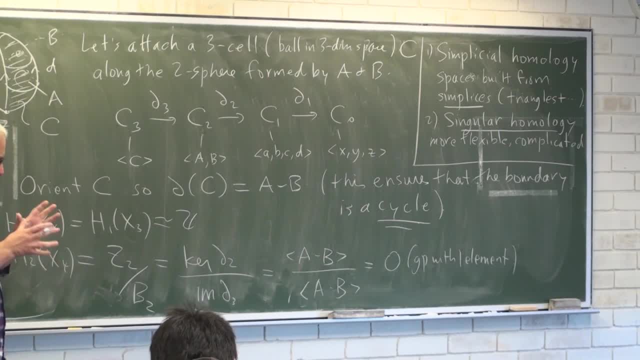 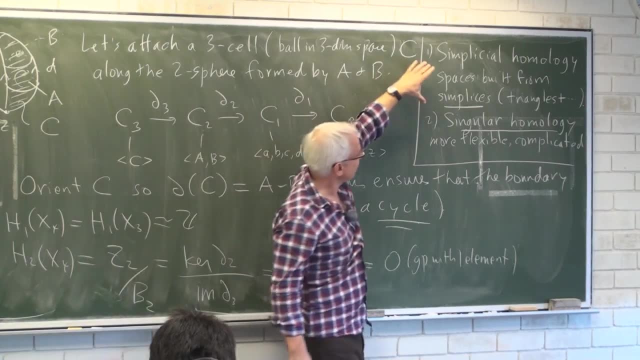 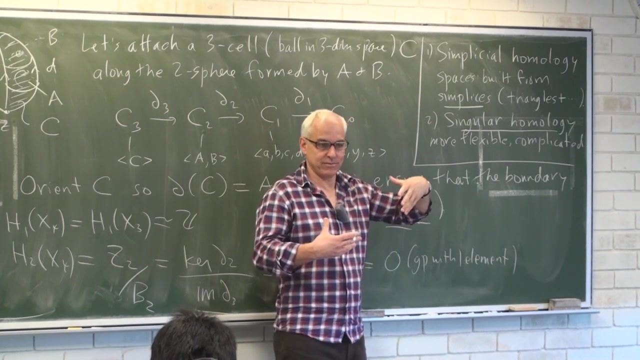 about. what exactly are we talking about? how do we set these things up in a very combinatorial, precise way? And to do that, we're going to have to talk a little bit about these simplicial complexes, spaces built up from simplices. 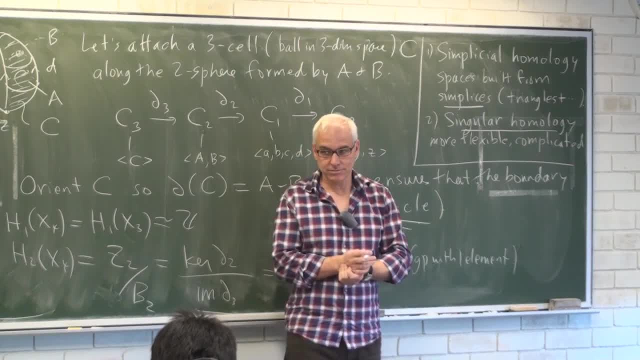 which are higher-dimensional analogues of triangles. So that's what we'll do next. I'll see you then.